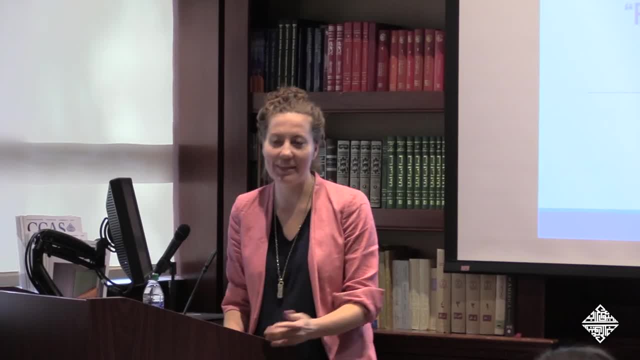 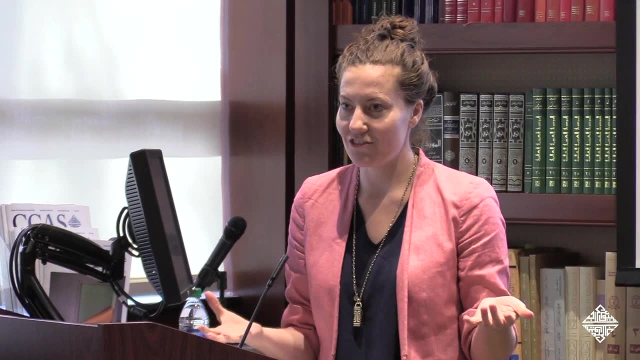 for introducing me and thank you for having me. I'm really excited to be here today to discuss my work with you. So what I'm speaking today about is a work in progress. really, It's a book project that I'm working on and it really comes out of a much larger study. 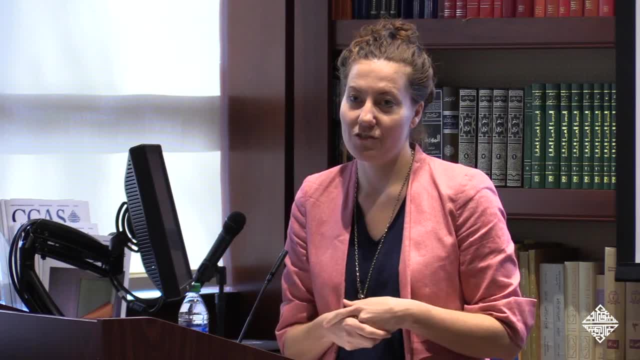 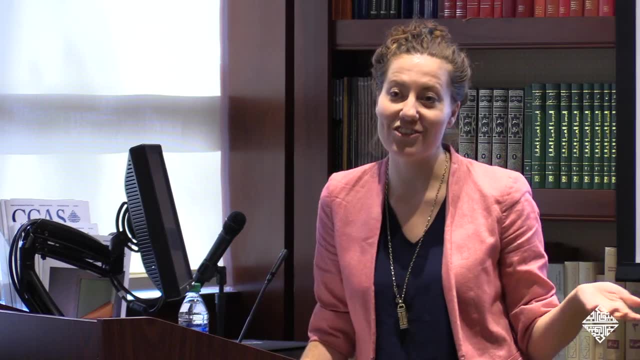 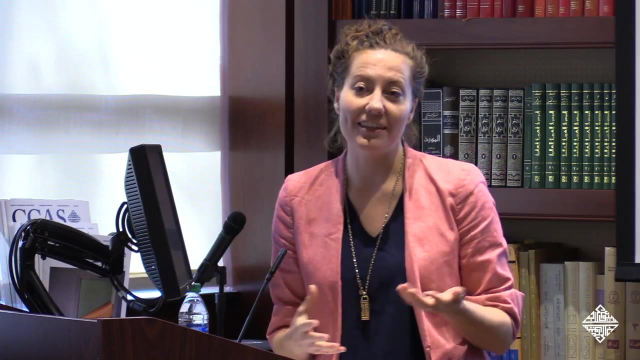 in many ways, of over a decade studying higher education reform in various parts of the Arab Middle East and North Africa. So I thought it might actually be of interest to you how I became interested in this topic. So I was originally not interested in higher ed, you know, or education generally. But 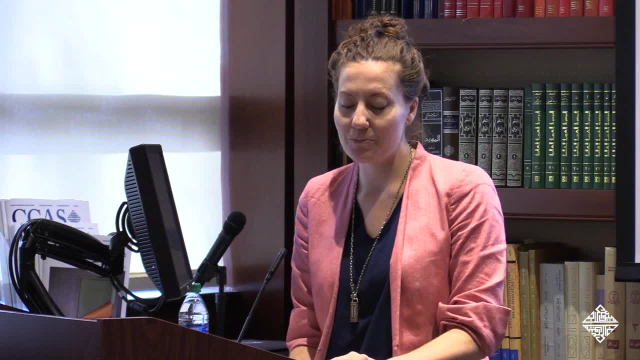 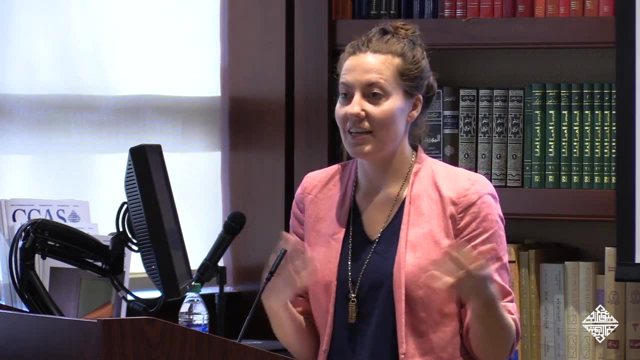 so I had just graduated undergrad and I moved to Morocco. I was a Fulbright grantee there and I was studying the role of English and the sort of growing influence of the English language and how it was competing with French as sort of a language of power. When I started 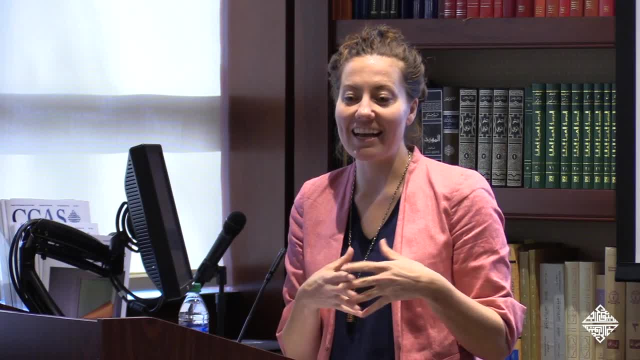 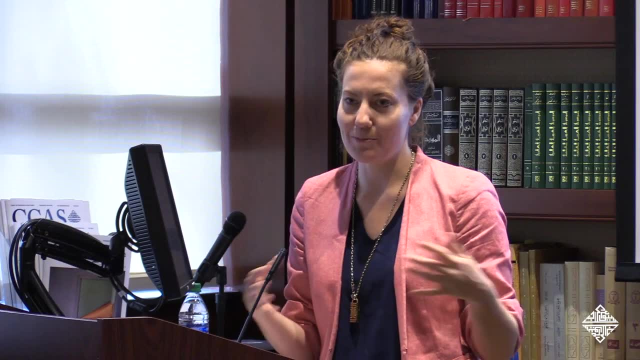 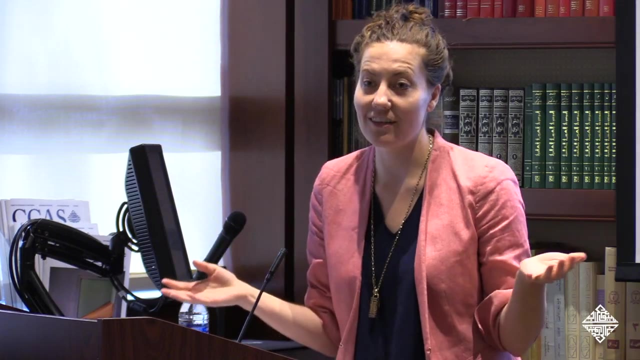 to teach a class at Mohammed Singh University in Brabant and I literally had no advanced degree, no specialization, no contract, no office. I wasn't paid, but I literally was in charge of teaching two university-level classes to about 40 Moroccans in the national 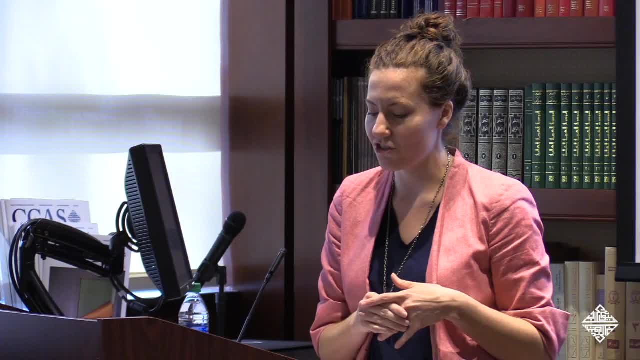 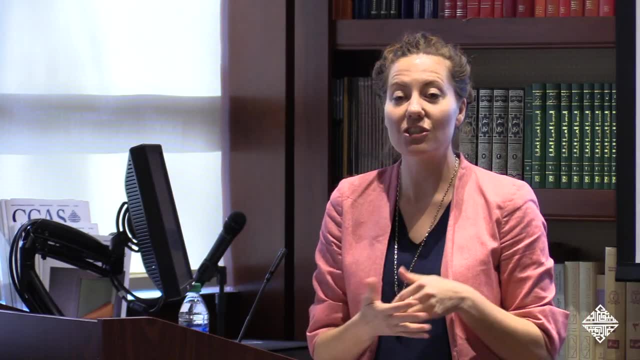 university- essentially the first and oldest university in the country- And it was a really transformative experience for me. It changed my entire life. It changed my entire life. It changed my interest from sociolinguistics broadly to higher education because the students 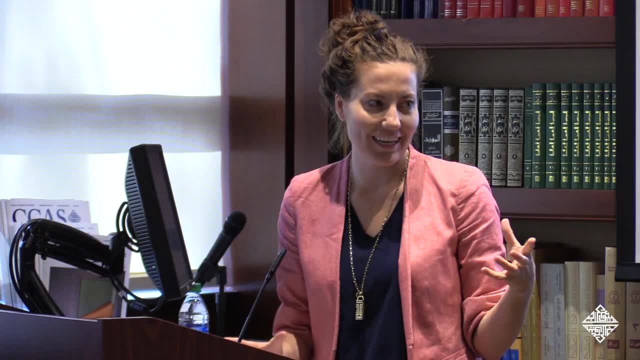 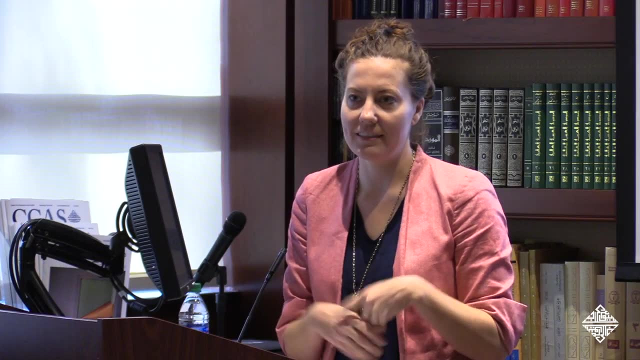 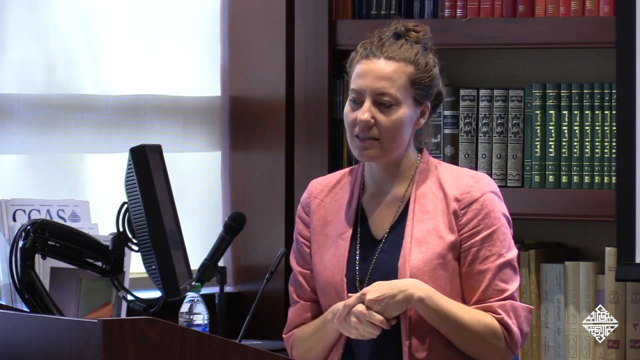 I was teaching were bright and brilliant, And in many cases they also, you know, were struggling to get by. They didn't necessarily have money to buy dictionaries or pay the fee to get to the university, And so I really became interested in this question of how. 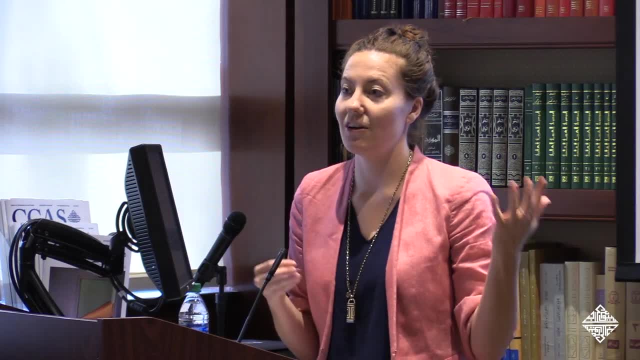 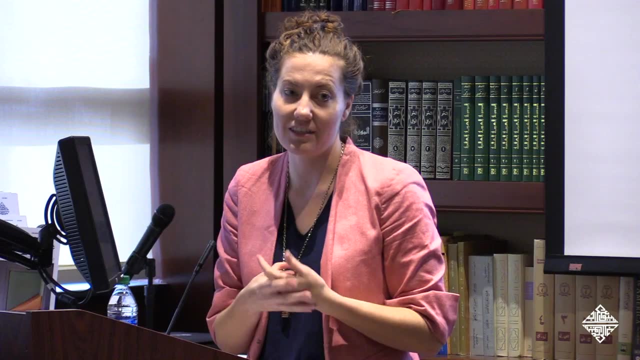 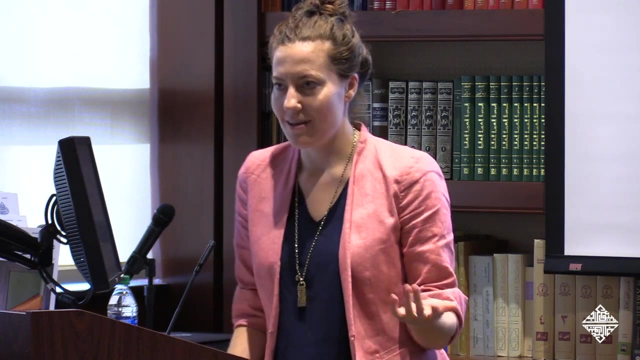 are universities and the states and the governments that are funding higher education and higher education and organizing and managing these universities, providing opportunities or failing to do so for their youth. And that's the question that I really pursued ever since then And that's what took me to do my PhD in comparative education at Stanford, And 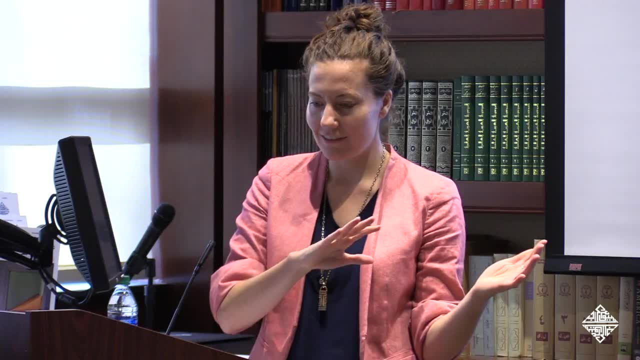 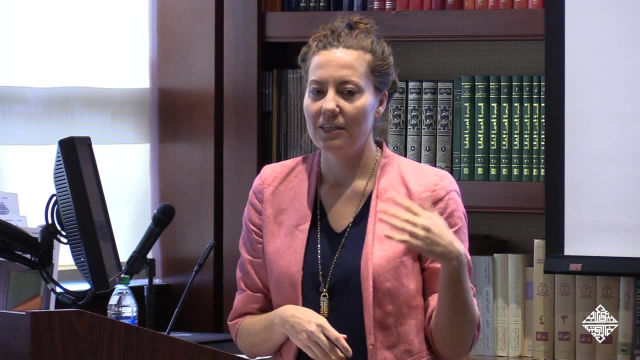 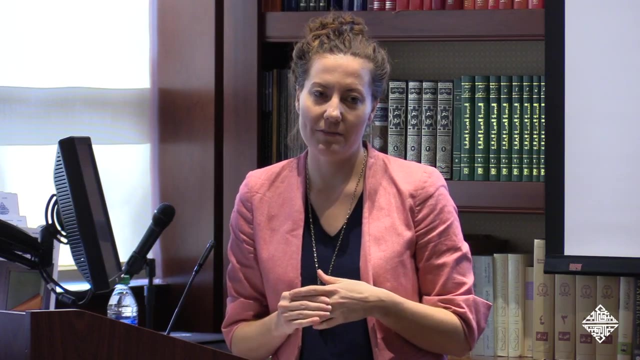 since then I sort of have traveled eastward in many ways. I started to. I spent a long time in Morocco, but have also done field work in Tunisia, Jordan and Syria before the conflict And then, more recently, I spent more time in the Gulf I was affiliated with. 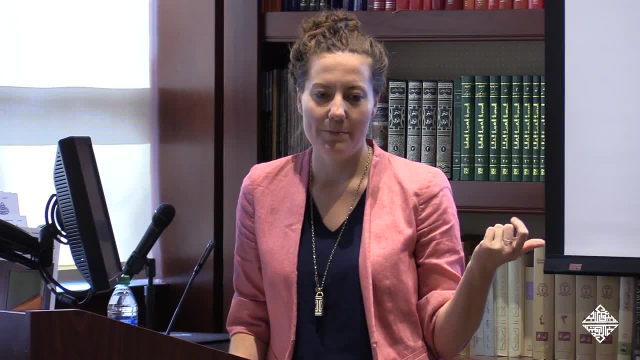 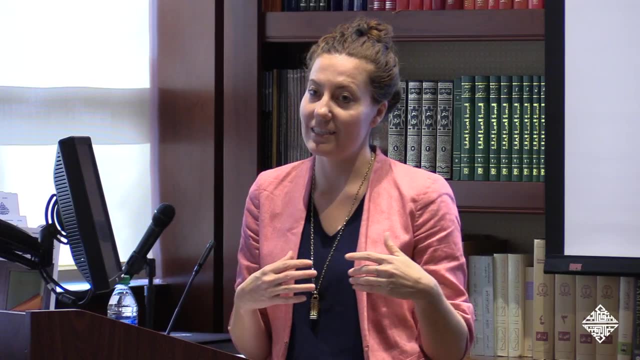 the Kosmi Foundation in Raqqaimah, and so I've been to the UAE and Qatar as well, and Lebanon. So really this book focuses on the countries where I've spent time living and studying- And it really emerges out of many, many conversations- like my dissertation field. 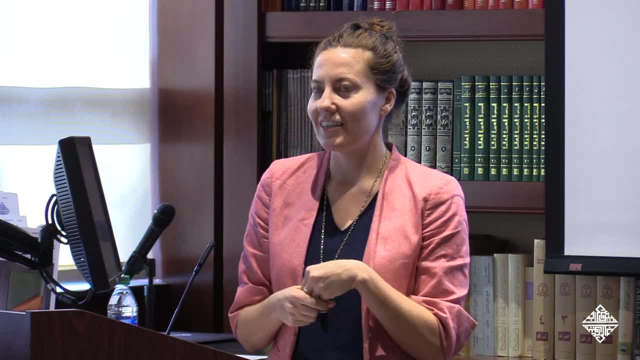 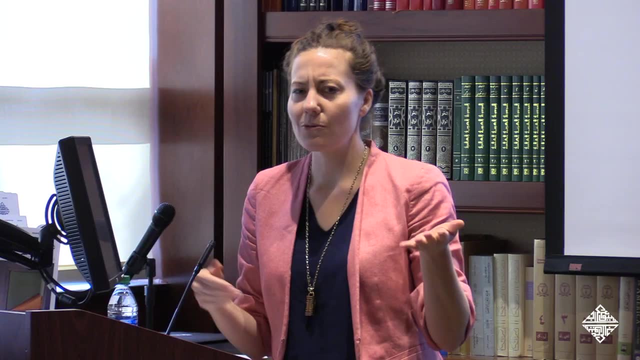 work, but also teaching, lecturing and, honestly, just you know, studying Arabic with my tutors or riding in a cab throughout the region asking people like: so where did you go to university, How did you make your choice, Why did you choose that place? And so, in some 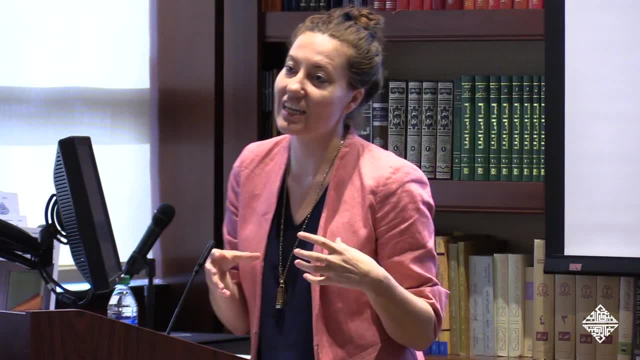 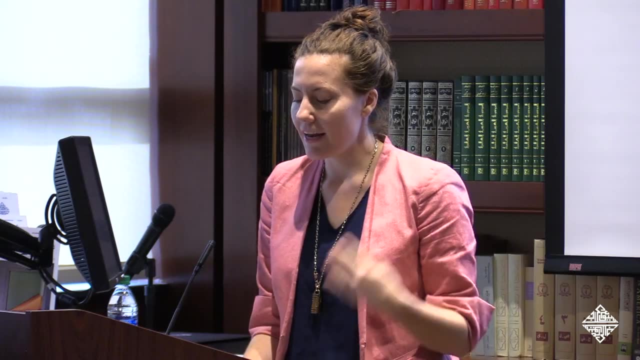 ways it's a bricolage effort of trying to really understand higher education policy and its reform throughout the region. So the and it I have a book manuscript that's currently, you know, under review. those of you I know who are working on books- It's. 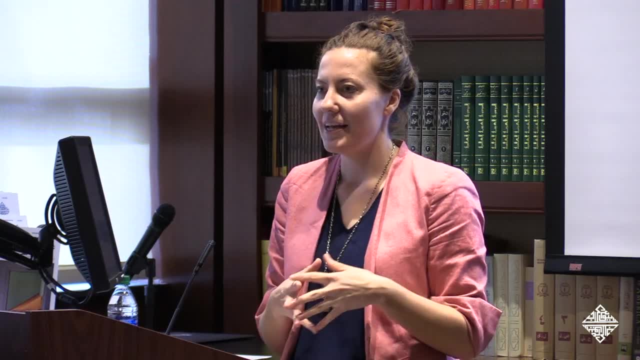 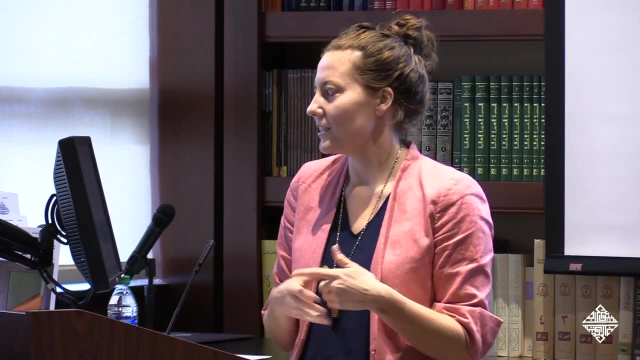 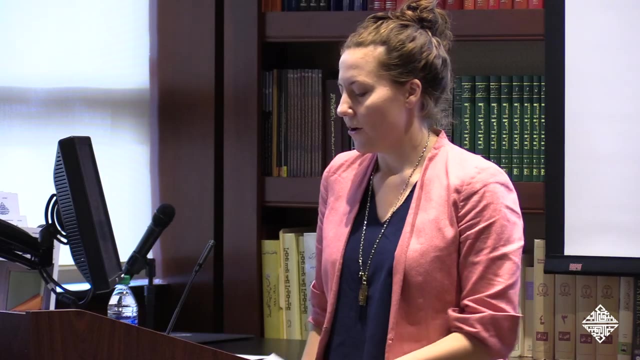 a very long-term effort, so it's not out yet, but I'm excited to speak on- you know sort of where the book is going and what I argue in it, And I call it Degrees of Dignity, Reconsidering Higher Ed Reform in the Arab World, And so I'll just start with this. what? 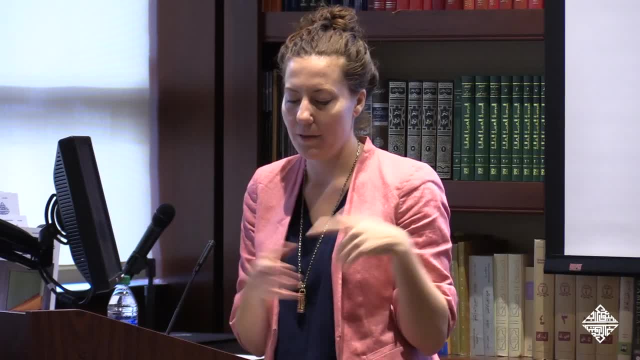 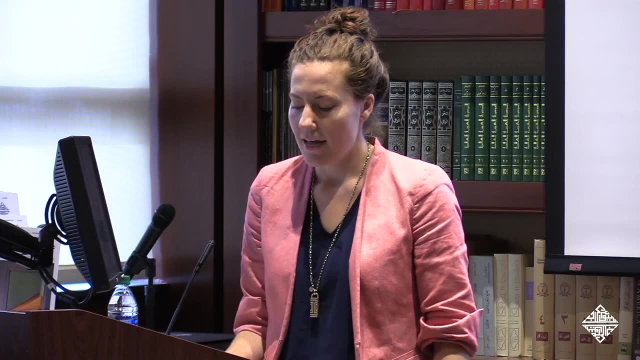 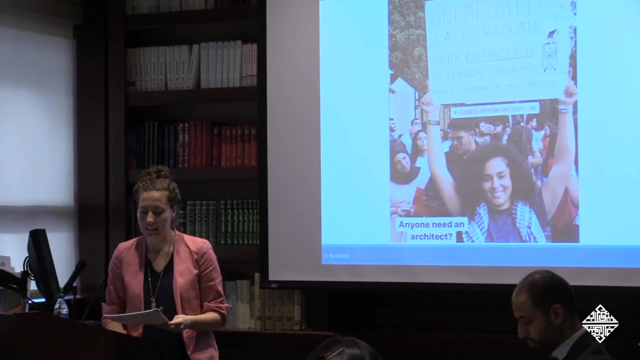 I see where did this book come from? really, Since the late 2010,, when the people-led protests broke out in Tunisia and Egypt, much of the Arab world has really been upended, And so we know, and obviously these are ongoing today, but we know that in the academic circles, 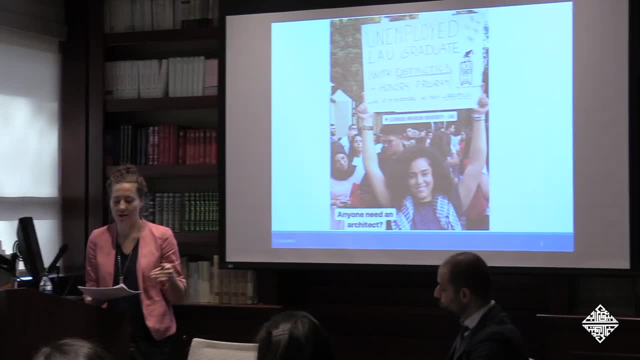 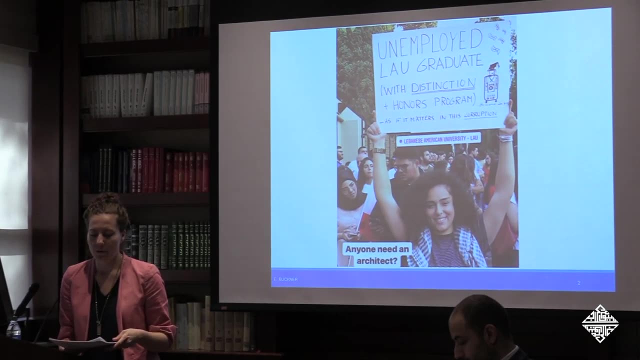 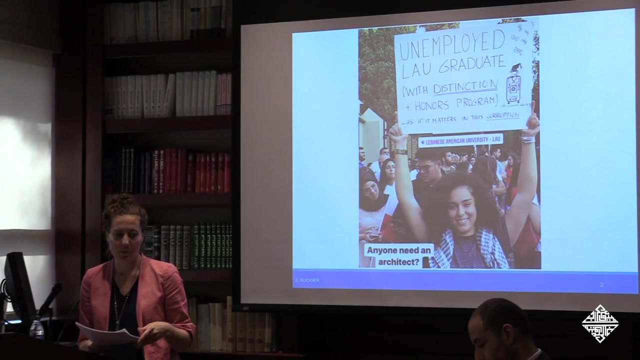 and the popular media. the Arab Spring's call for bread, freedom and dignity has in many ways, been understood as a demand for economic and political justice motivated by inequality, poverty, unemployment, repression and corruption. And, as I said, these protests are ongoing. 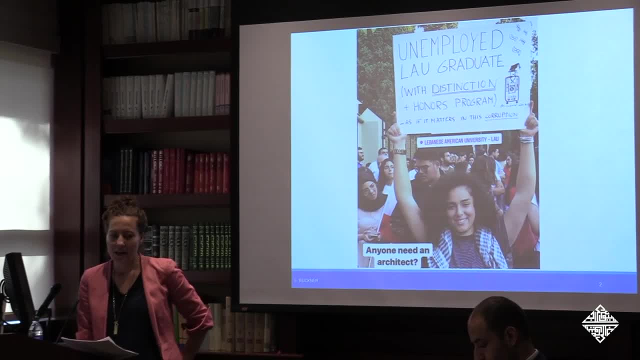 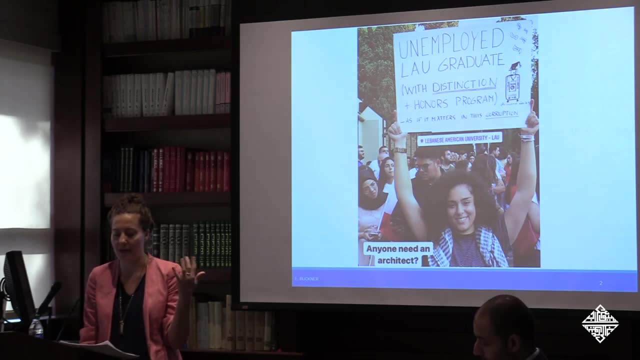 throughout the region, in Algeria, Sudan, Lebanon and Iraq. Hmm, Young people and their discontents really have been central to understandings of the outbreak of the Arab Spring and ongoing protests, But these conversations about the causes and the consequences have rarely touched on the role of education and higher education in 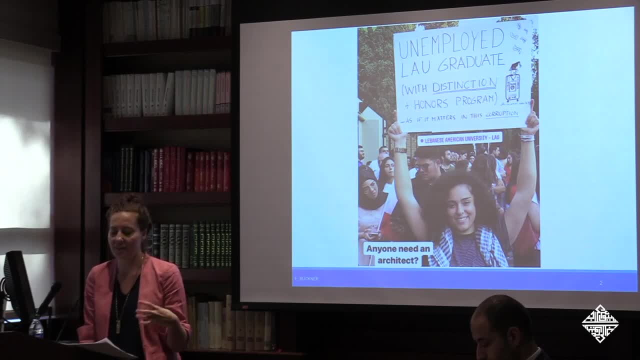 particular in shaping young people's lives and future opportunities, And I think that's in some ways due to like the blinders of the field. Scholars of Middle East politics tend to really focus on who has power or what they do with that power, how they maintain. 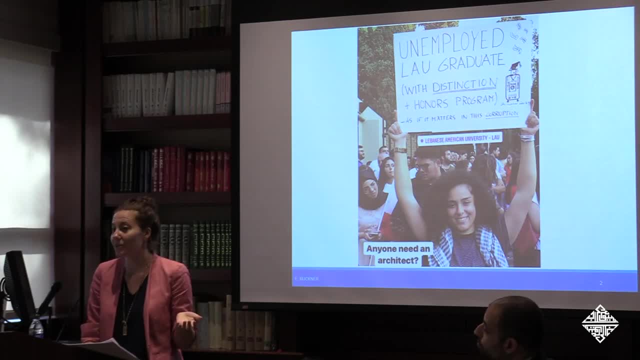 that power without spending much time on social issues such as education. Meanwhile, if you come from comparative ed, like I do, if you work in international development, as I do, international development agencies have a lot to say about education And these. 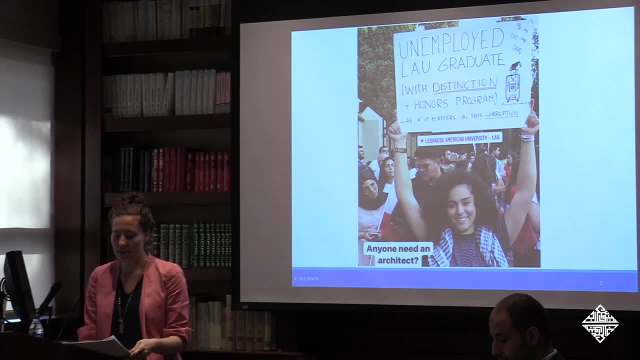 include the World Bank and USAID and others, But they tend to draw almost exclusively on economic theories of labor productivity and they really criticize higher education in the region as inefficient and ineffective And often even worse. sometimes these policy discussions really adopt this Orientalist gaze that casts the whole region's systems. 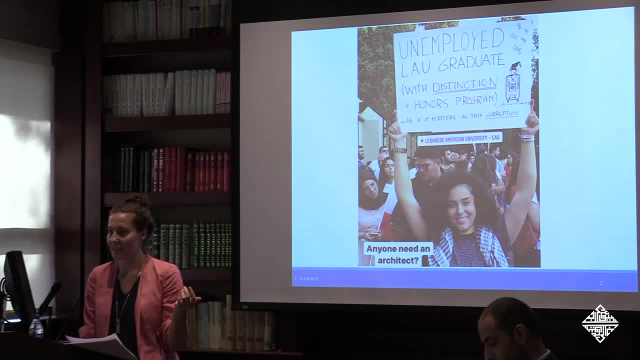 as failing or lacking because they lack financial resources and they're often characterized as lacking in knowledge and whatnot. And so I start the book from this premise that we need better and deeper and more nuanced conversations about higher education policy and its reform in their region. And obviously all of that is not just. there are some excellent scholars. 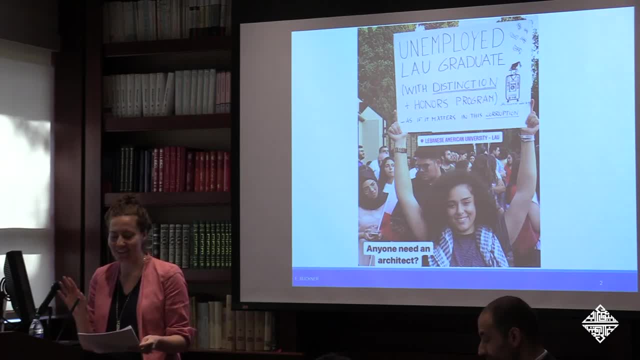 like Hida here, who study education, but in general we lack these nuance. She's really unique in that way to have these nuanced conversations about education, And so I, having studied this topic for a decade, think of higher education as this really dynamic arena. 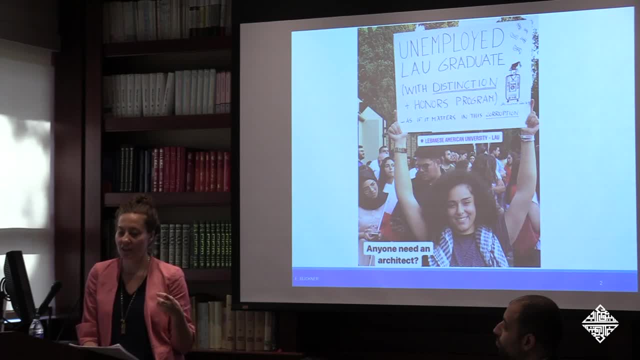 to talk about, And I really think of questions around higher education policy as invoking normative questions about who a society really is, who should profit from education, who deserves the benefits of a credential, for example, as well as many contentious policy debates over quality and access. And so I start from this premise that, as long as the 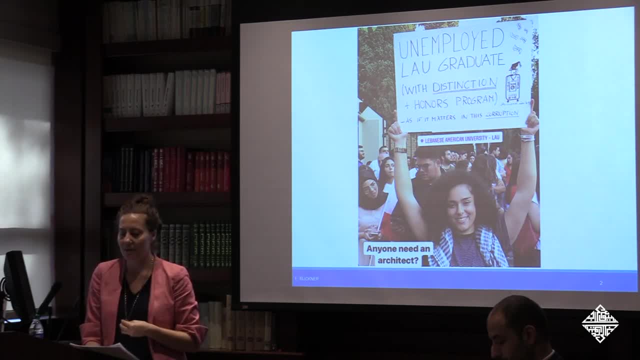 political scientists are ignoring education and the economists are sort of treating it as a purely technical matter, then important questions regarding higher ed reform are remaining unanswered and unaddressed, And so I start in my book saying that there's this pressing theme for more nuanced conversations, where we view higher education as simultaneously. 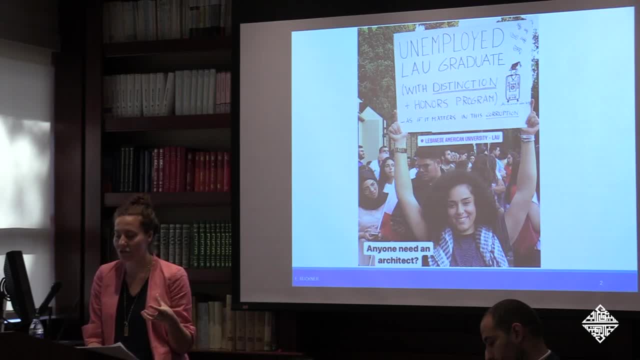 a social and cultural and politically consequential institution, while also fully rejecting stereotypes of Arab societies as inherently lacking in knowledge or capacity or quality or local scholarship, which is entirely true, And so I also start from this premise that studying higher education as an institution is that higher education, the university, is a really important site that we can learn. 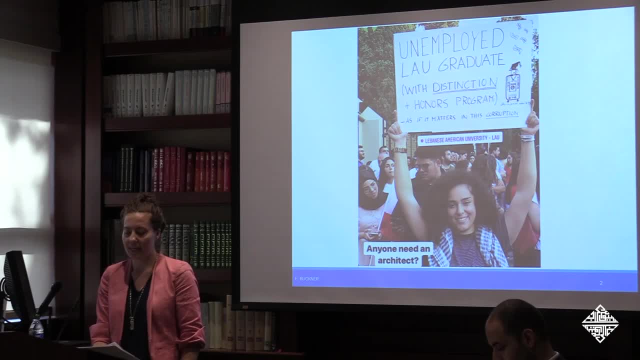 from that has a lot to teach us about Arab societies more broadly, And so I argue that many of the problems that the Arab state is facing today are not simply political questions of non-representative political systems or heavy-handed militias or high rates of corruption. 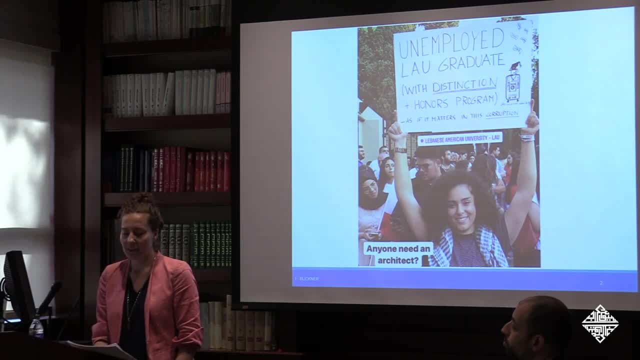 I mean, these are all very true in some cases, but they're also manifestations of low levels of state legitimacy, And so the inability to provide young people with economic opportunity, social mobility and a sense of progress and dignity have undermined the state's legitimacy. 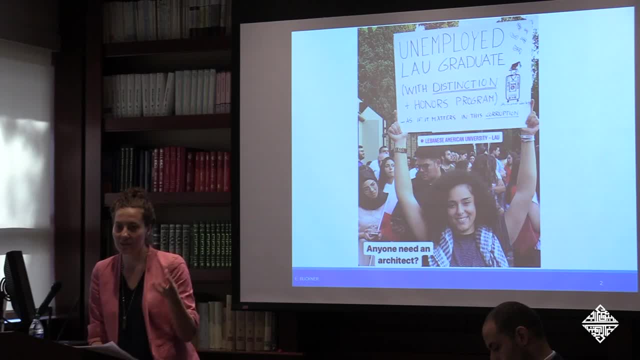 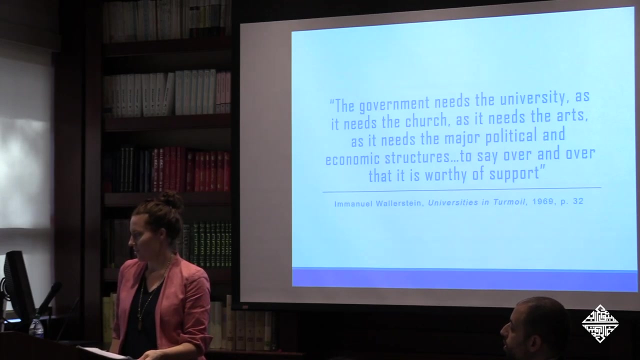 in its young people's eyes. But these issues can't be divorced from higher education, Because that is the role that universities have historically played in their societies, providing that site for national unity, mobility and opportunity. And so, in fact, I draw on this quote, which is from a sociologist from a very different 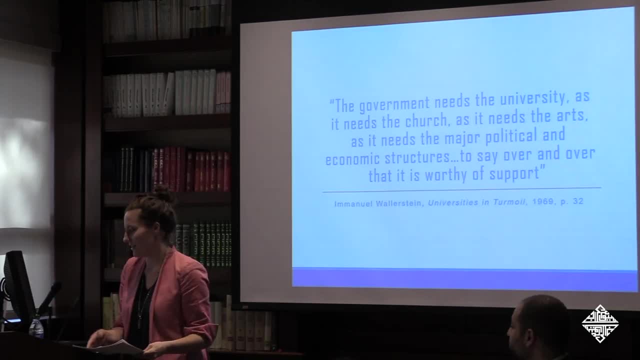 era and a very different context. If you study comparative ed, you might know this name: Wallerstein. But he argues the government needs the university as it needs the church, the arts and the political system And the political and economic structures to say over and over that it's worthy of support. 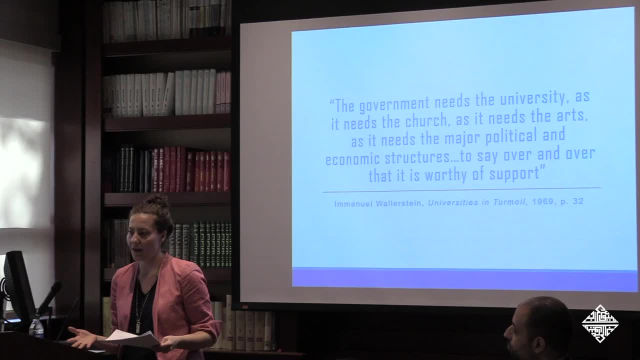 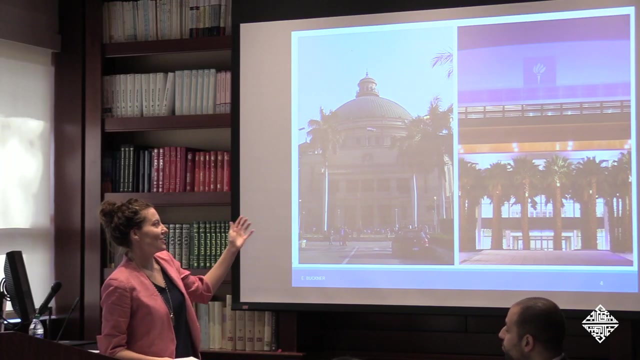 And so, in some ways, I started this book thinking about higher education as this very important institution that we really need to understand better, And so, with that as the background, I really think of my book as the story, of this story, from this to this. 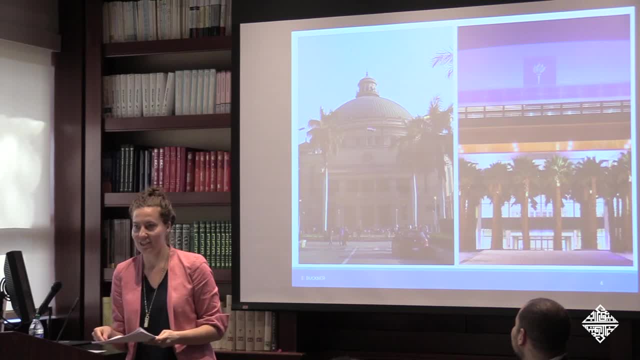 And so, and many of you may recognize these two, These two universities and these two very different models of universities, And so we think of- you know, scholars of higher education really think of the university as one of the most easily recognizable and legitimated sources of knowledge and advanced. 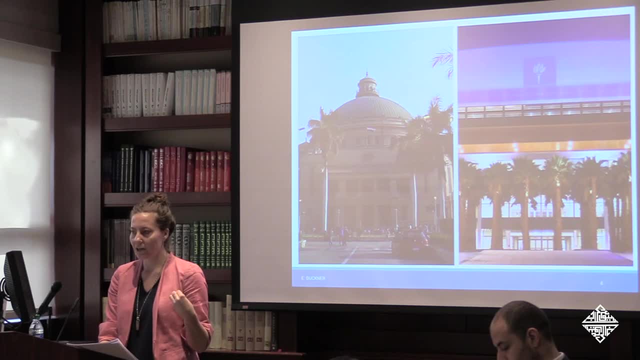 training in a society And in their world, as in many parts of the world, and especially post-colonial states, the university played a crucial role in state and nation building sort of for over 200 years. And so universities in this sort of early, I, in my research, think of these two different. 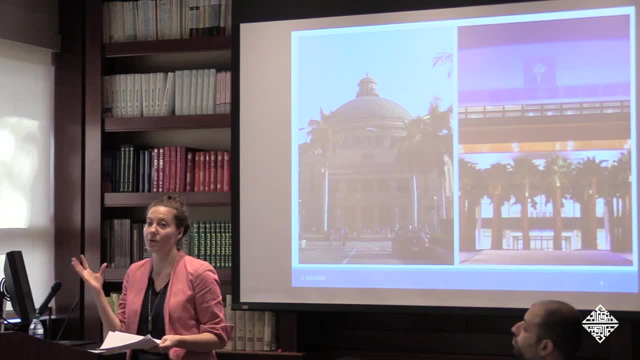 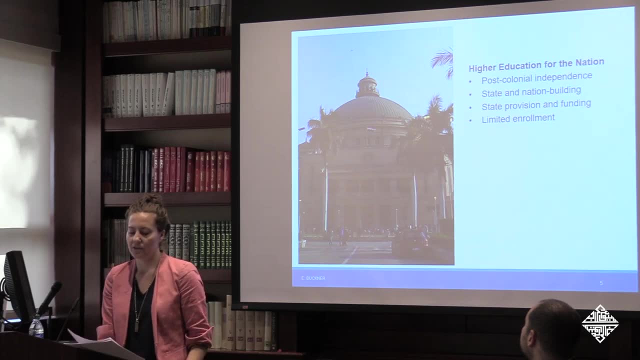 eras, one as nation building and one as the global era. And so, in this era of nation building, the, in many parts of sort of modern era, Middle East and other post-colonial states- Universities, were, these, symbols of social mobility, national unity and economic development. 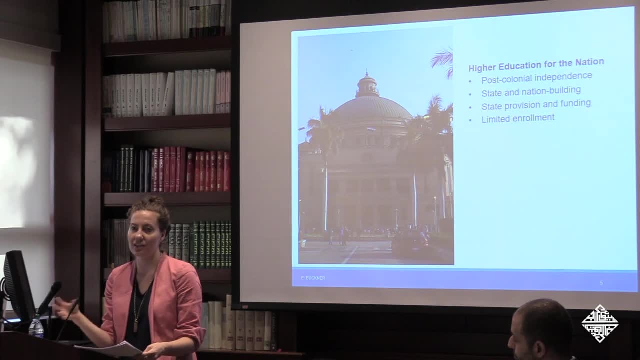 And they played an important role in a larger effort to consolidate power under a centralized state, to strengthen the legitimacy of their own ruling regime and to educate civil servants for an independent post-colonial nation state. And this was so in in this era. not everyone went to university. 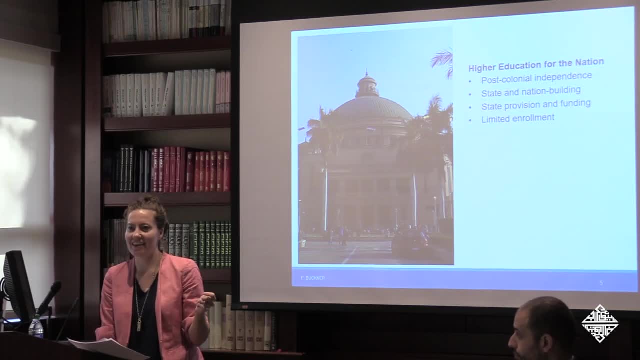 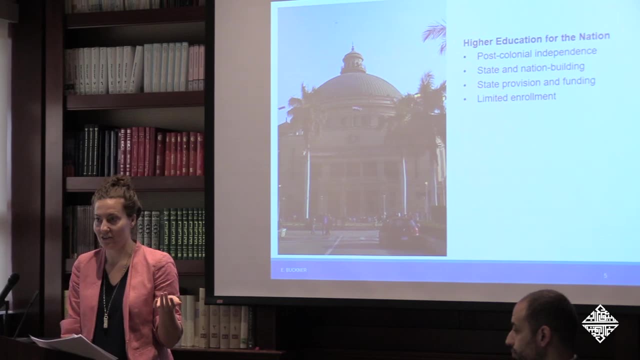 Not very many people went to university. in fact, right They, they served a small proportion of the population. It wasn't considered, it wasn't intended to be mass or universal right It was. and then if you went to university, you often guaranteed employment in the public sector. 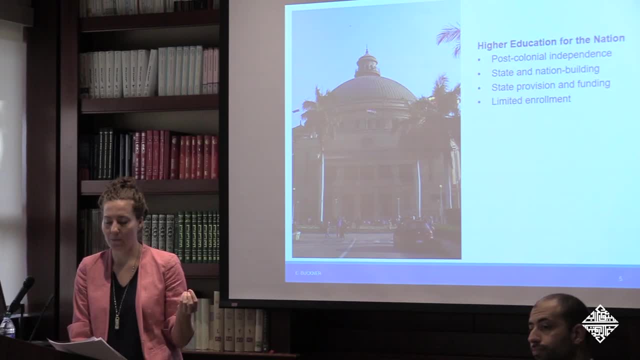 as part of a sort of, you know, nation building. And so now we're in this new era that's supposed to be, you know, this era of globalization. National university systems are being called, Students are being called on to fulfill a very new mandate, and that is to produce highly. 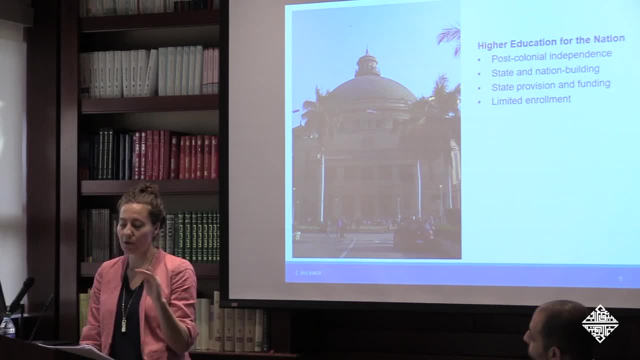 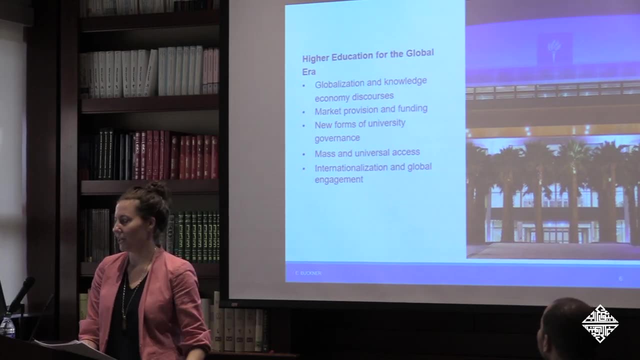 educated, in many cases entrepreneurial workers for a globally competitive and mobile economy, And so I I call this sort of higher education for the global era We are. you know, we are sort of embedding higher education policy within discourses of globalization and the knowledge economy and increasingly looking to market provision. 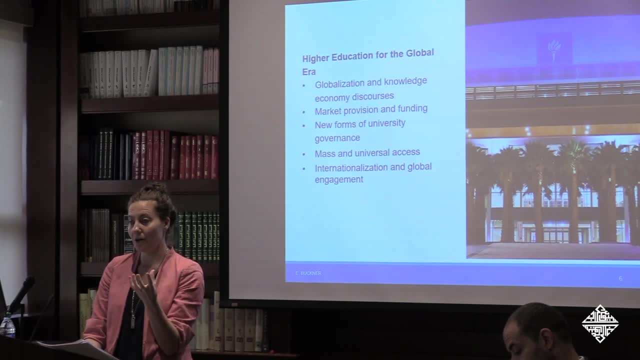 and funding. We have new forms of education. We have new governance, new models, including, you know, the transnational providers or international branch campuses, And in many ways, we are expecting higher education to be a mass institution, if not a universal institution. 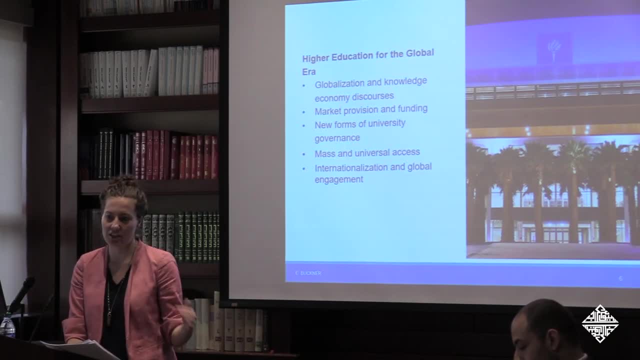 So we in higher ed think of mass access as actually over 40% of the population and universal as like over 60, right? So we are expecting increasingly large cohorts of students, And so this shift from higher education for nation-building to higher education for global. 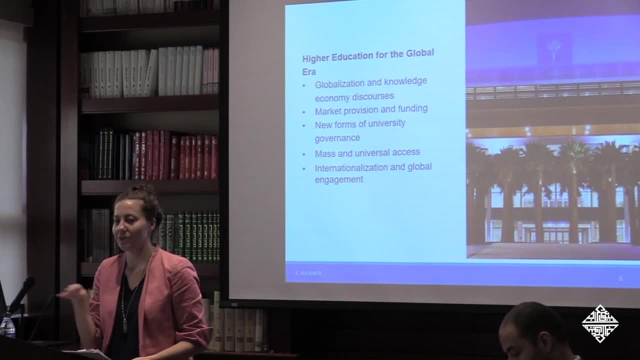 competitiveness is not just affecting the era of what is really a trend everywhere, but it does require. it's not an easy undertaking, is what I would argue. It's actually very difficult to take a system that was designed for pretty small sizes of cohorts. 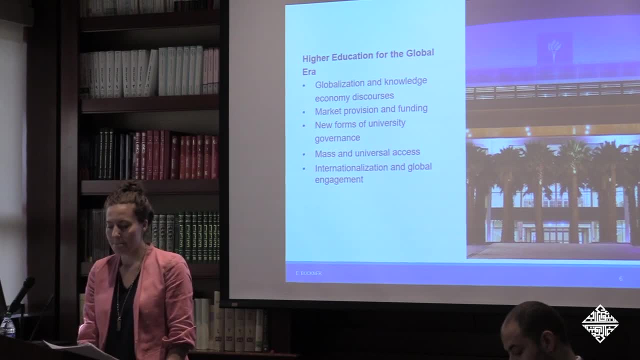 And so it's hard to do, at least to make a system that is so diverse that we can finally expand access everywhere, And so, by most accounts, the era of world is sort of failing at this shift, And that is evident if you study sort of the discourse on this. 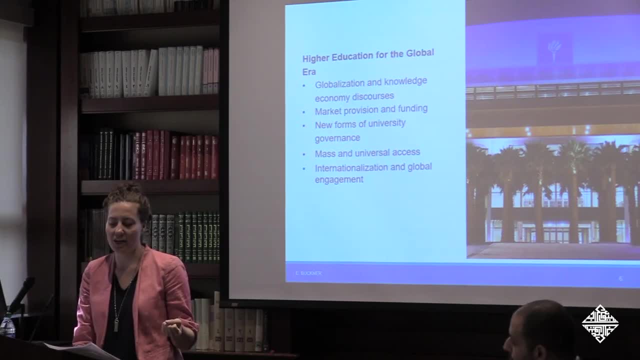 A constant stream of reports decries the problems of higher ed in the region, And it's on many different levels: on admissions, on financing, on governance, on quality assurance, the production of scientific research, research. all of these become sources of criticism, severe criticism, in many cases by international. 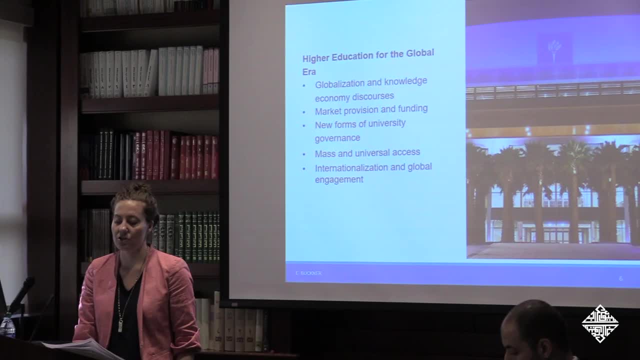 development experts, and sometimes national governments as well. And so the critiques. these critiques are often really rooted in human capital theory, which argues that formal education makes labor more productive, and so, by making labor more productive, it now has more economic value. And so economists in the region have for decades argued that the educational institutions 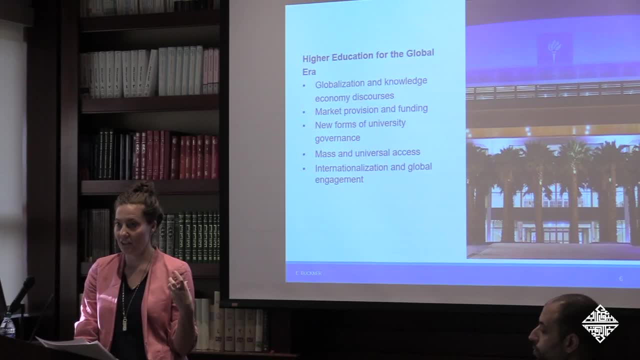 are of low quality and they're not preparing youth for this, their new, with the knowledge and the skills that they need for productive employment in this new sort of global economy. And so what this looks like? yes, this is just one example. 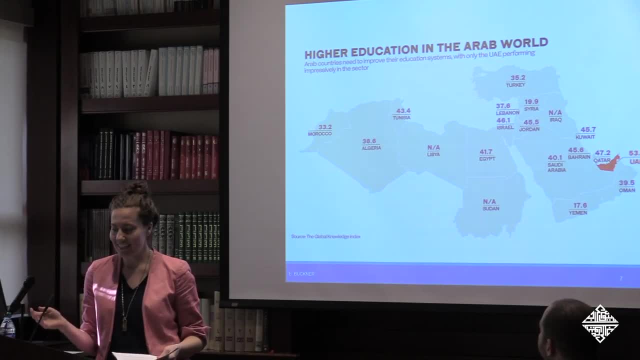 For example, the Global Knowledge Index. I just use this to sort of point out that this exists, That we're now increasingly ranking countries based on their sort of global knowledge, and this index argues that Arab countries need to improve their education systems. That's just, you know. take it for granted. 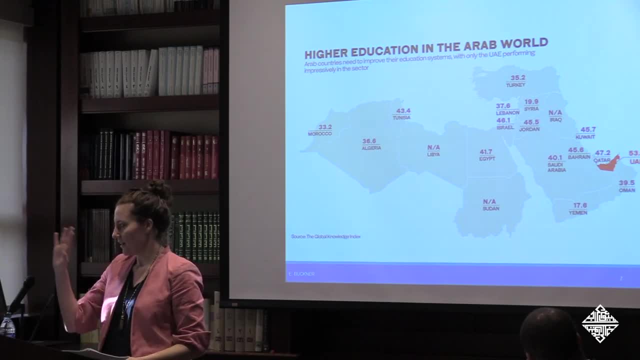 This is an example of the discourse, And so they're saying: oh, everywhere is sort of failing at this, except for the UAE, which is more dynamic. But this is really just. I don't. I'm putting this up there to take it with a grain of salt. 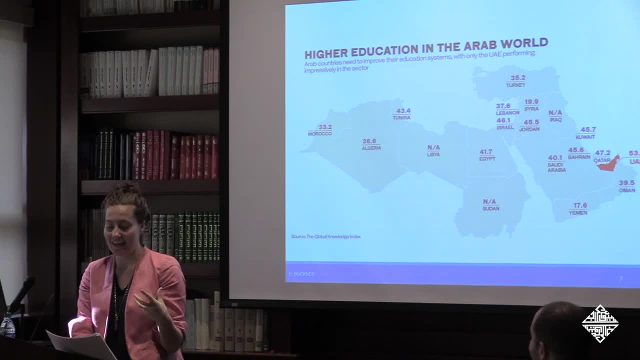 This is one clear example of how this discourse is pervasive And And really ubiquitous. And so the what you notice in this literature, where you're ranking countries and ranking institutions, is that people are very rarely mentioned. I mean, we don't really think about individual people's lives except to the extent where 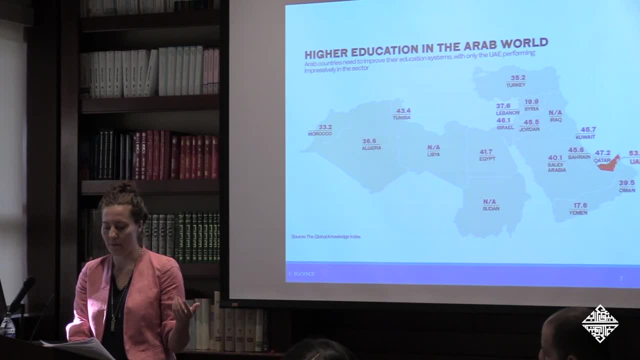 they're sort of undermining effective implementation of policy reform And the higher education system is reduced to its numbers. I mean, like what does 33.2 even mean Right On a global index? And so we? but this is just. it's reduced in every domain, right. 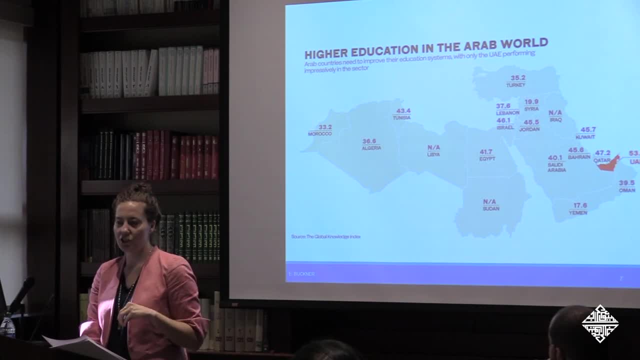 The budget is the admissions rate. quality assurance becomes a particular indicator. Research productivity is measured by how many publications in peer-reviewed journals- typically in English, you know- per 10,000. individuals Like these are very quantified indicators of quality and whatnot. 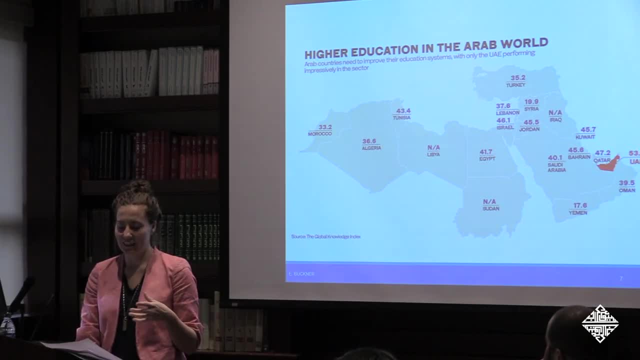 And so the reality of people's lives, their everyday lived experience, Their experiences as they're navigating these changing policies and higher ed systems are very rarely taken into consideration. And the various reasons that we know young people attend university, including social status, their parental pressure, peer, boredom or marriage prospects. there's a lot of you. 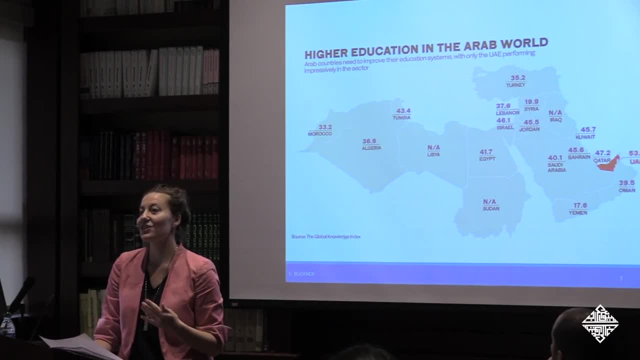 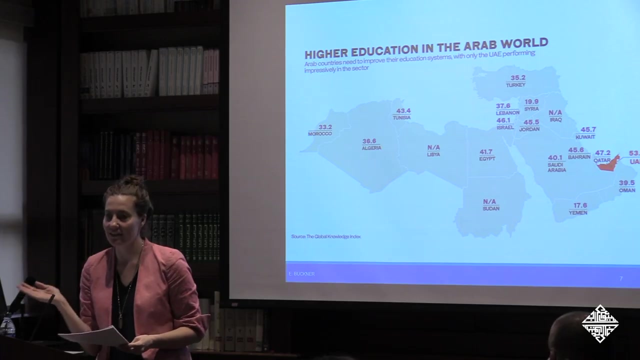 know social and cultural studies that point to the diverse reasons why young people attend higher ed. They are very rarely considered And sort of the dominant. The dominant lens is one of economic productivity right And, moreover, these reform approaches tend to look for a very quick-fix technical solution. 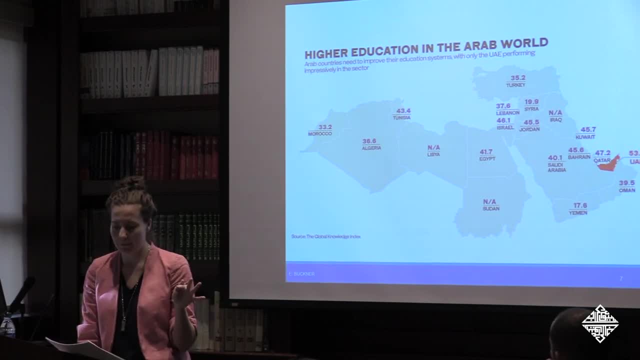 whether it is in the form of privatization or let's just create public-private partnerships, let's have a new quality assurance agency or mechanism or international, let's import an international best practice. And they largely ignore the broader social and political context in which these reforms 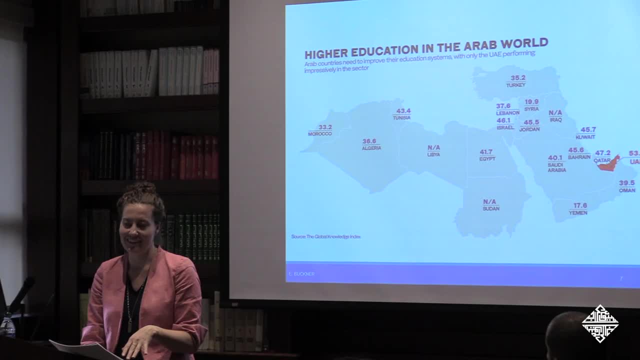 are actually very debated and contested and then often, you know, unaffected, not implemented fully, And there's always a concern of why the reform wasn't effective, without sort of recognizing that the reform was sort of additive in the first place. And so the point that I just make in my book: I take a very different approach to doing. 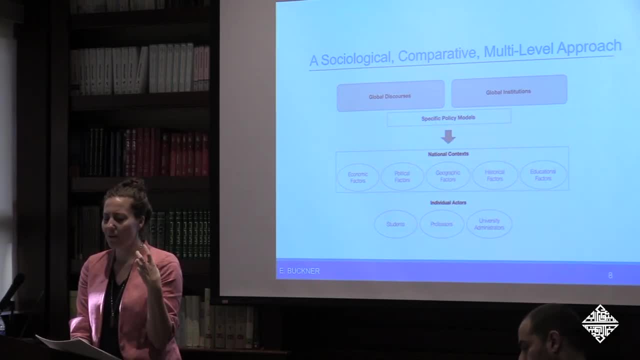 this work And I really want, I hope, that I frame it as trying to overcome some of the limitations of this technology And that is, I think I'm going to focus on some of the most important aspects of this technical universalizing prescription by adopting a sociological and comparative perspective. 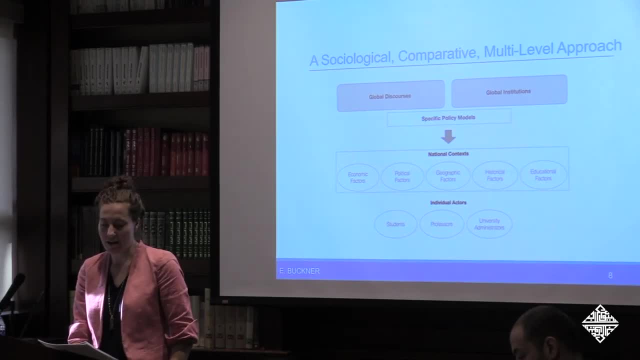 on higher ed reform in the Arab Middle East, which comes from my own training in comparative ed, And so I look at both sort of what is going on in terms of like: why are different countries adopting different policies? What are the big policies that have changed higher ed in the region? 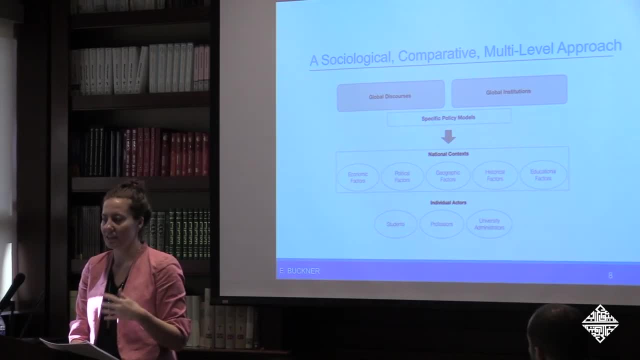 And then what are their effects on young people's lives, or professors, or the different actors negotiating in these spaces, And so this is a very, very broad approach. And then the other thing I want to talk about is that we don't really have a very clear 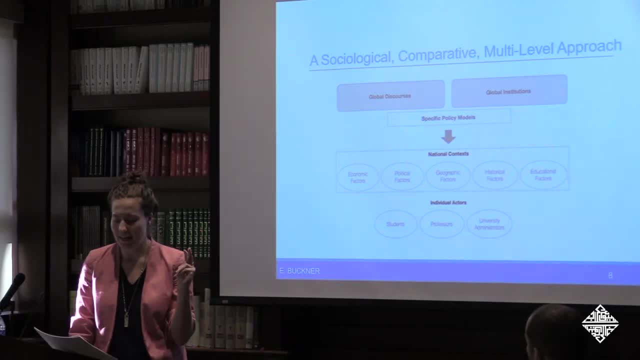 This is the way I think of my book. in many ways, By saying I adopt a sociological approach, what I mean is that I think of higher education as a social, cultural, political institution. So when we think about reform, we're not just asking a purely technical question. 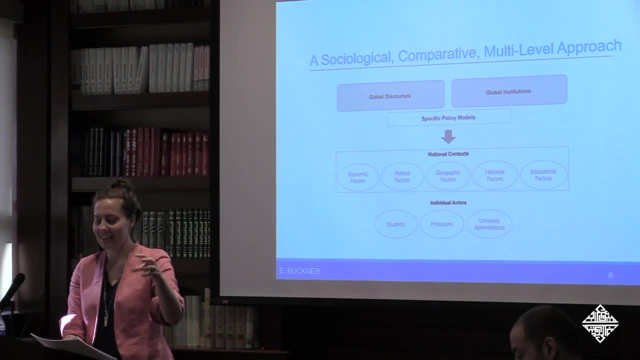 of what works and how can we implement what works right. We're thinking, rather we're recognizing that different stakeholders have interests and thinking through how individuals are negotiating structures or norms that are institutionalized norms and different individuals' interests, And then so by saying it's a social institution, 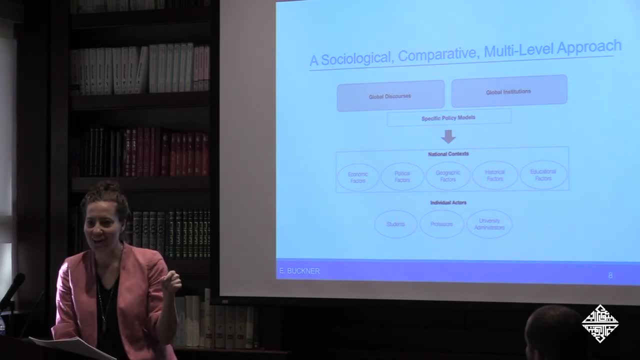 I draw on Andre Mazzaui, who I know some of you read for today in the class, where he calls higher education a precarious and contested terrain. in Arab societies that's linked to social status, political influence and economic opportunity, And I really use that to think about some of these issues. 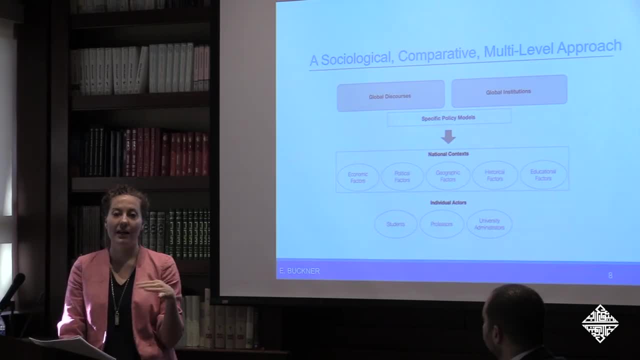 that, for example, the World Bank would position as a purely technical issue of what should be the standard of admissions to university. You know, on the Tajiki, for example, should it be 55 or should it be 60, right? 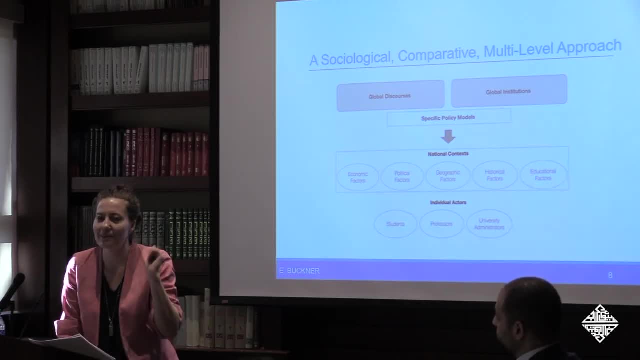 That's a. in one sense it's a purely technical question of what should be the minimum standard, But on another question it's very political: It's who gets access to the, the power and status that a university degree comes with. 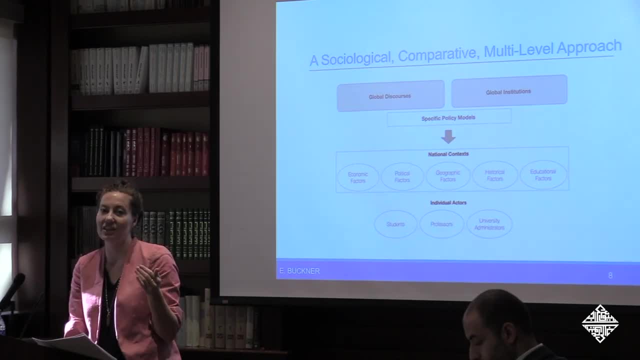 or who should get access to the most elite and prestigious degrees like an engineering or a medical degree, right, And so that's where I start And I say: well, you know then, if you understand how important this degree is, the difference between a 59 and a 60. 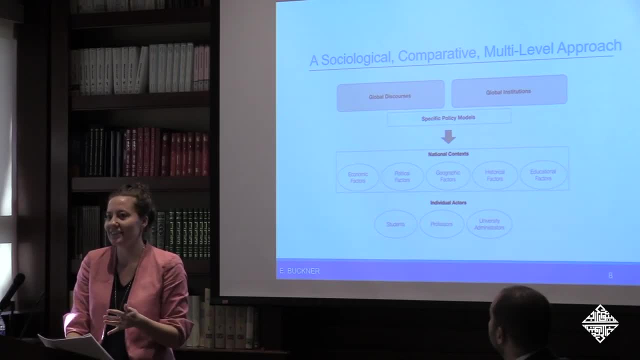 is actually very consequential, and it's not surprising that students and families are adopting many, many strategies, from private tutoring to just cheating- to get that higher. you know grade right, And so that's sort of one of the issues that I study. 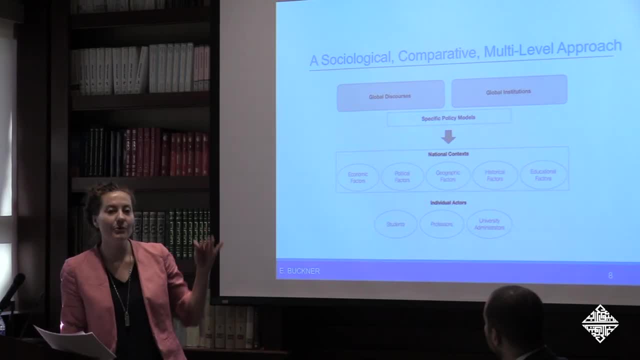 And then, secondly, when I say I adopt this multi-level approach, I draw on a very long-standing tradition in comparative ed, where we situate education systems within global, national and local contexts and we recognize that they're simultaneously being influenced by many different factors. 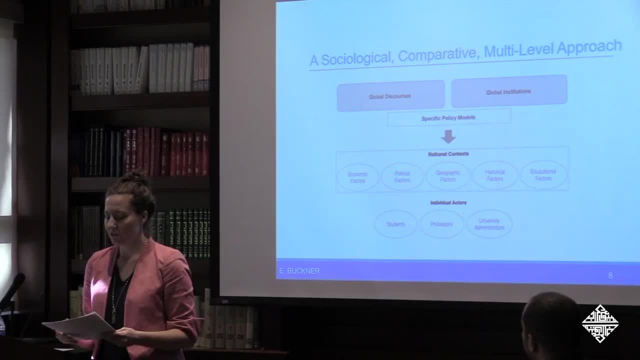 And so, within comparative ed, we point to sort of two big shifts, of discursive shifts in higher education that I, you know, think of as these global discourses, And one of these is the idea that education at all levels, including higher education, is now both possible. 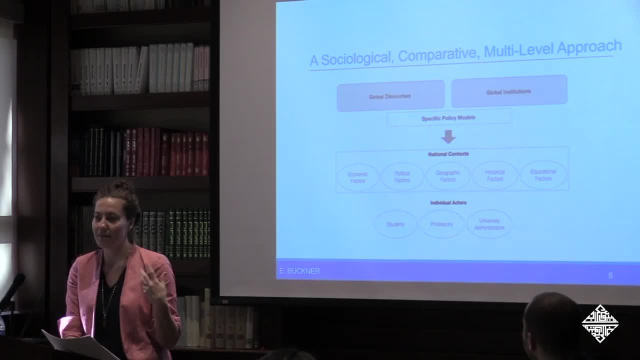 and desirable for ever larger portions of youth And in many cases, at the lower levels. it's framed as a human right, We think, and increasingly higher education is included in those discussions as a right. In 2015,, the US Department of Education 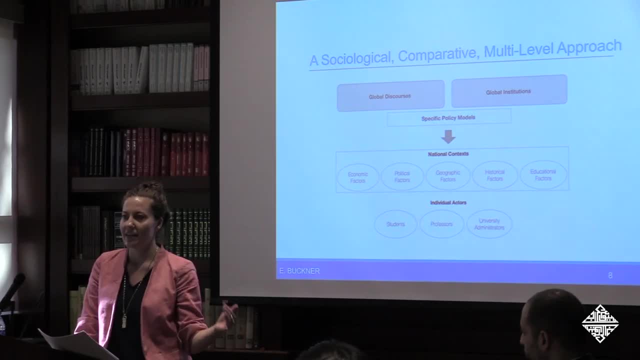 and the UN and all of you know its nations- passed the Sustainable Development Goals, the SDGs, and in that goal four is the goal in education, which includes- it actually includes- a year of post-secondary in it, So it actually commits all nations to provide. 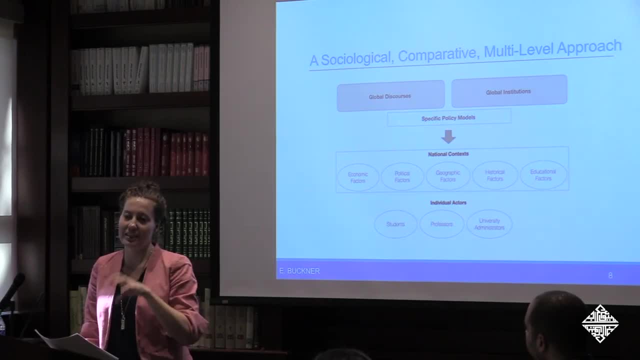 not only a full course of primary- like basic and secondary, primary, secondary- but also one year of higher education as well, And so increasingly countries are committing to expanded access to higher ed, But we see it both as a right and a catalyst for development. 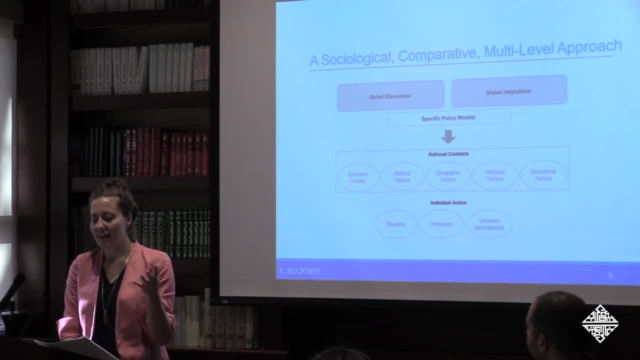 And so, at the same time, the end of the Cold War has meant this rise in neoliberal thinking. Honestly, it's sort of a neoliberal global era where higher education is being shaped by particular and powerful discourses about how to fund and manage higher education. 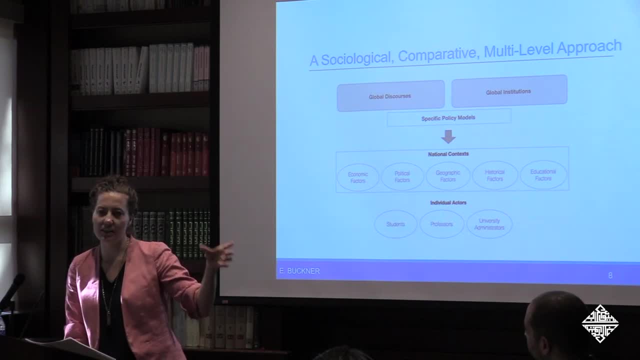 So I have really focused in my book on two: what I think of as the knowledge economy discourse, which positions knowledge as central to national economic development, And neoliberalism, an ideology that contends social policies of all sorts, including education, should be guided by market principles. 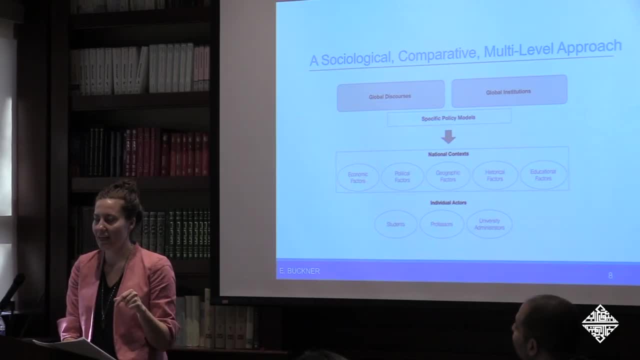 including deregulation and consumer choice, And so that has led to not only the rise of privatization, but also, in many cases, it's filtered down to the individual level, where young people are now expected to be the entrepreneurs of their own lives. 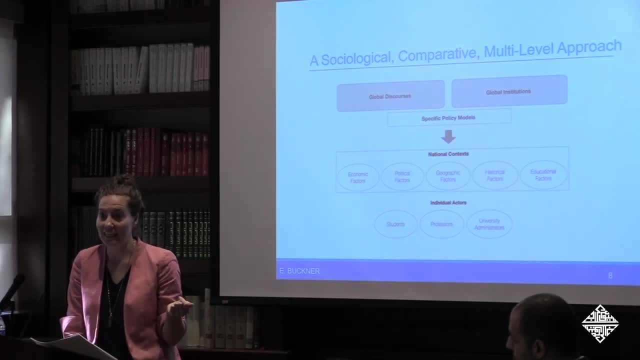 where they manage and navigate their own destiny. And so these two discourses have been developed and diffused by really powerful global actors, including the World Bank, the United Nations and many donors such as the US and the European Union, in the form of very specific policy models. 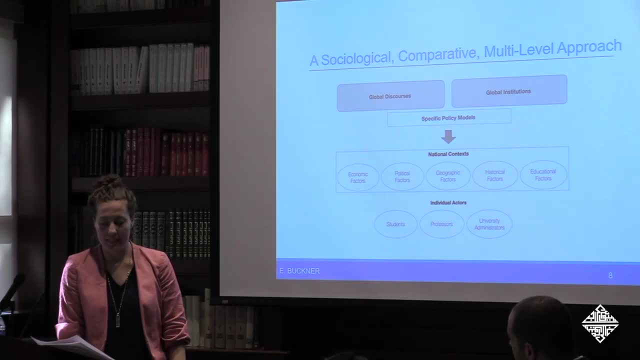 And so that's how we sort of think of this, And these would include, for example, private higher ed or quality assurance, And so part of what I do is I actually focus on these models, these- I focus on topics rather than countries, which 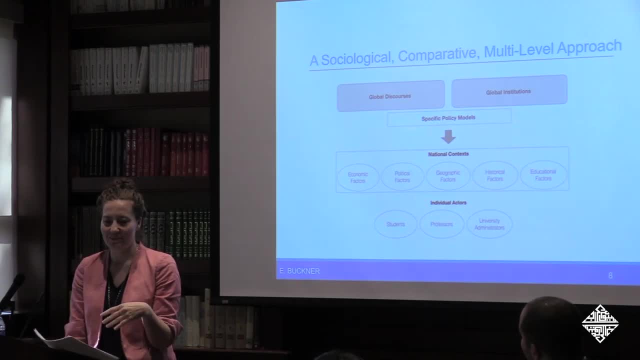 is one of the things that I am happy to talk about. So I then think about how are these models filtering down to countries that have very different histories, very different demographics, different populations, different geographies and political systems? They're filtering down in different ways. 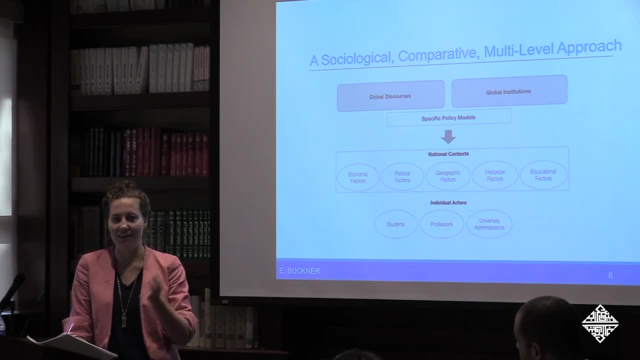 and they're taking effect in very different ways, for example, in North Africa versus the Gulf, and then young people and professors and others in those spaces are navigating them in very different ways. So instead of focusing on countries, which I would say is the norm and makes a lot of sense- 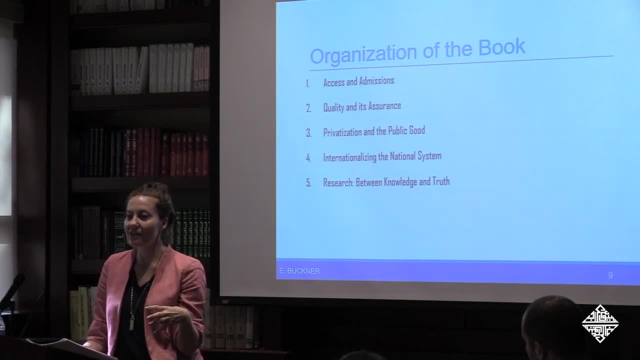 if you're really interested in deep contextual historical understanding. I actually focus on topics And I do that because I'm interested in the contemporary era where the sort of modern era of Middle East and North Africa has been grouped together in development, in particular as sort of a singular region. 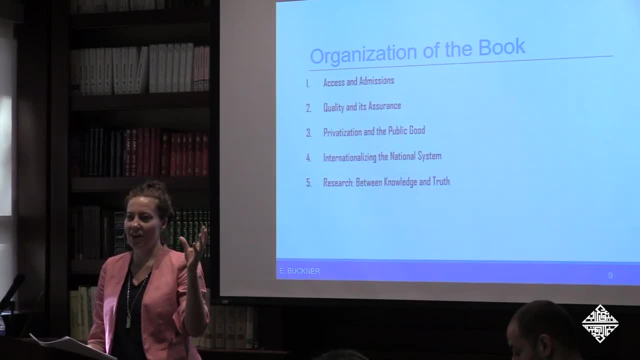 and models And those are sort of thought that they will work throughout their region. They're treated So. the first one is access and admissions, where I do look at this increased demand for access and think about how the admissions to university reflects and perpetuates longstanding state society. 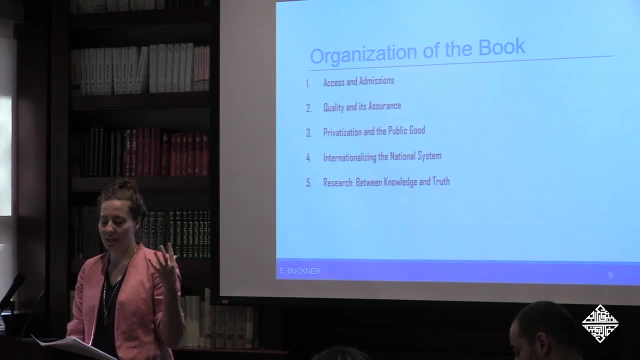 contracts and how those are sort of under pressure in the new era for increased access. And then the one that I'm going to talk about more in depth today is quality and its assurance. So quality is this. as I've mentioned, crisis is perceived to be a crisis, at least. 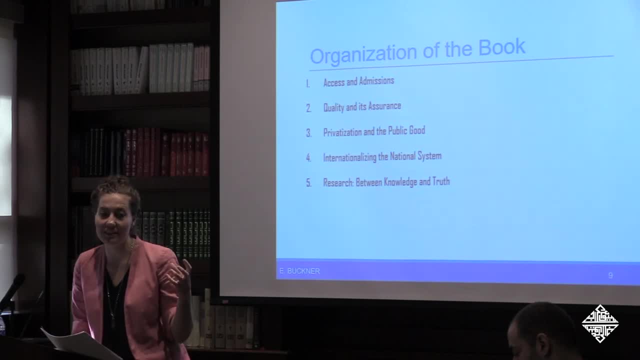 And I focus on- I will later sort of deconstruct this discourse of what this means and then how governments are trying to then assure quality by adopting new reforms. And then, if you guys have questions, I'm always happy to talk about these other three topics. 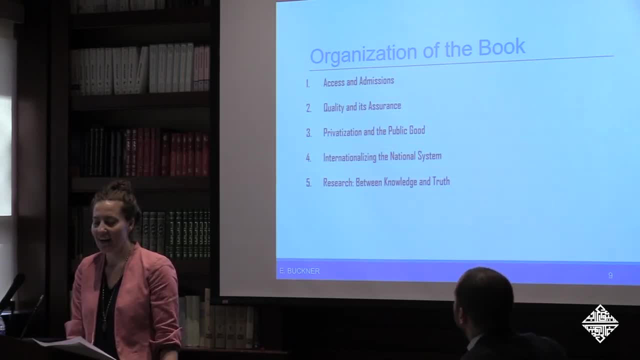 As well that I write about. One is on private higher ed and how. where is private higher ed, private providers, private universities, sort of taking off and flourishing, versus where is? it very contested And I look at that and I argue that it's flourishing. 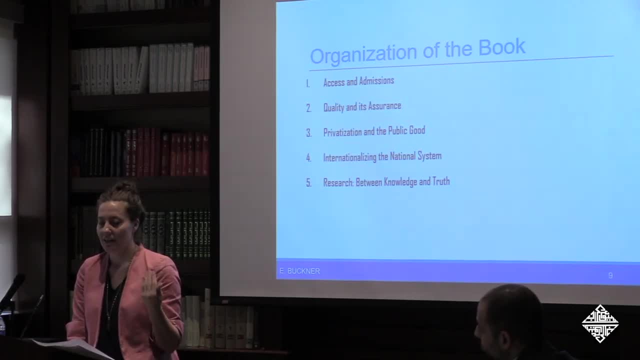 among those who aren't being well served in the public system and sort of what that means for the public university. And then I also look at internationalization, which is a broad term we use in higher ed, to think about many different trends. There are trends around the way that a national university 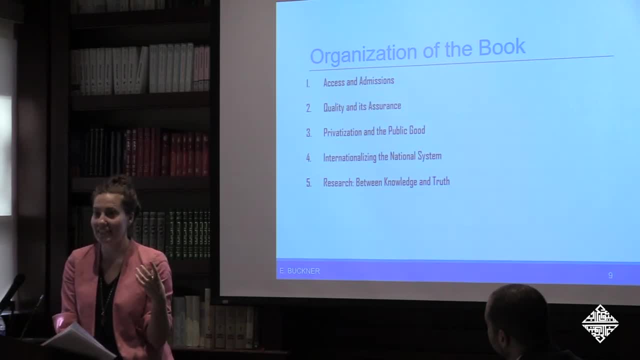 or system is embracing the global in its mandate, And so we're trying to not only appropriate international content, but also branch campuses are one example, or recruiting international students is another, And how in many ways, this is being used to sort of confer legitimacy and status. 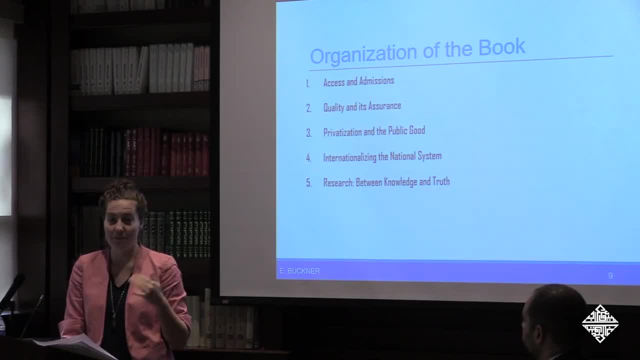 and distinction to those who are either attending or benefiting from these new opportunities, but at the same time the sort of tensions that creates with the national character of higher ed and the way that it is often used to sort of like reify, sort of Western 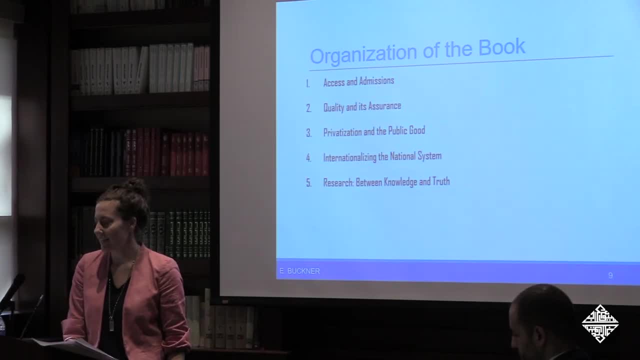 or foreign models at the expense of the local. And then the last thing I talk about is research and this intense focus on productivity- which is often measured by journal articles honestly, like patent production or journal articles- and the fact that these research outputs are not really taking. 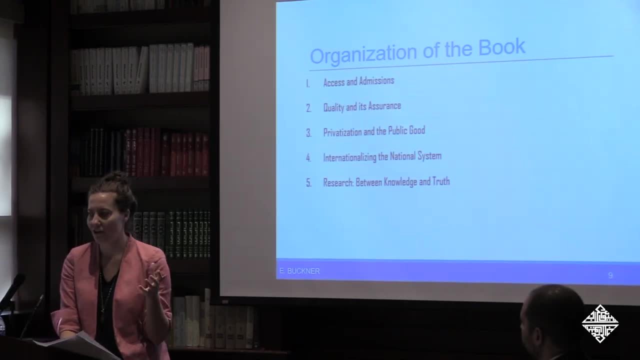 into account structural realities and the mess that's happening in the world right now, And so I think that's a really important part of this, And I think that we need to do a better job of thinking of research as a social and creative act in many ways. 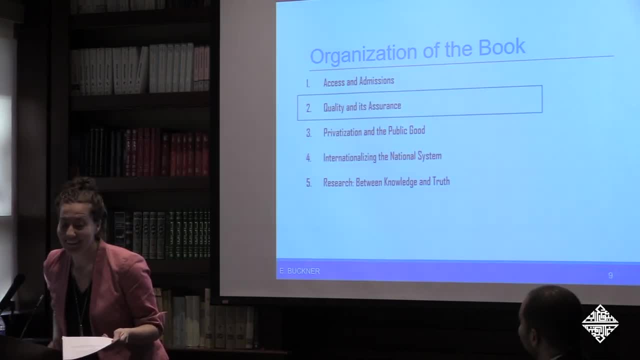 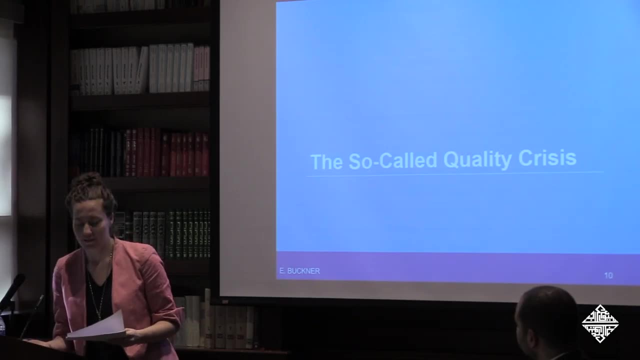 But today I'll just focus on quality and its assurance, And then- but yeah, in Q&A I'd love to talk about any of the other topics, So I call this- in some ways, we can think of this- like the so-called quality crisis. 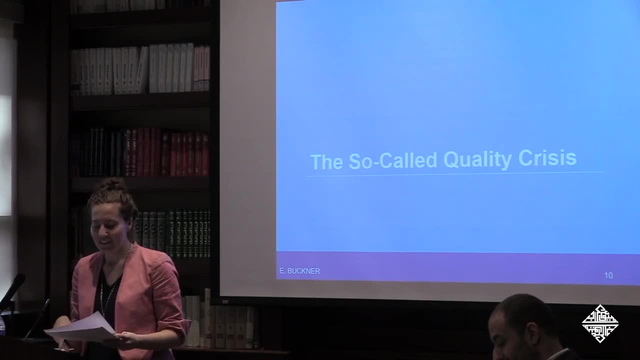 And I stand by this so-called quality crisis. So in some ways, the quality of higher education throughout the region is characterized by this all-consuming crisis rhetoric. That's what Petieri says in her Ethnography of Learning in Morocco, And it's so pervasive I'm sure many of you know. 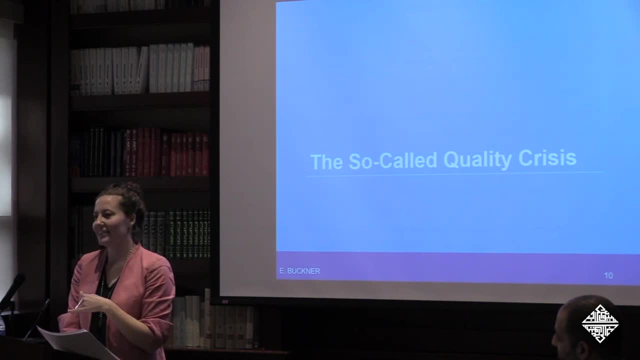 that technical experts, the academics, the policy makers, you know, even leaders themselves, largely agree that higher education, like primary, like secondary, before it suffers from low quality, And I think that's a really important point. So, if you want to understand this, what I mean, 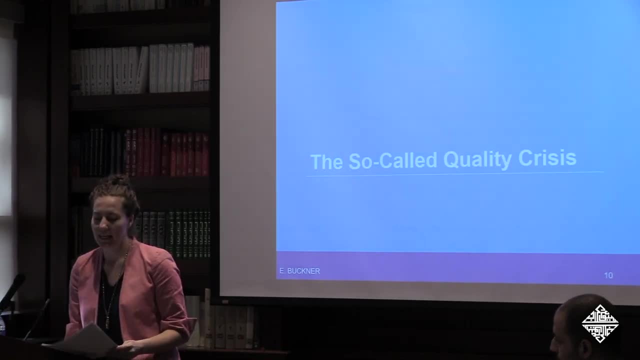 what is the nature of this quality crisis? you do have to put it, I say in global perspective. So there is this increasing global emphasis that goes back to the knowledge economy discourse that quality is crucial to economic competitiveness in a global knowledge economy. 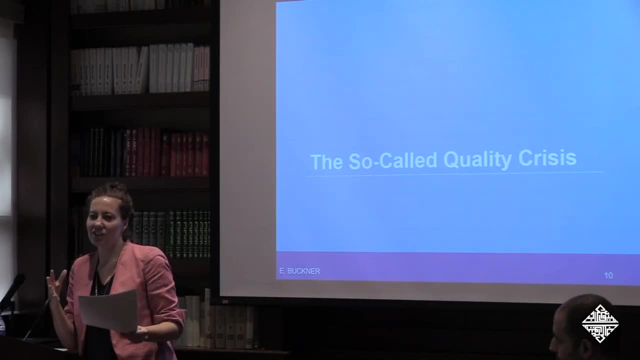 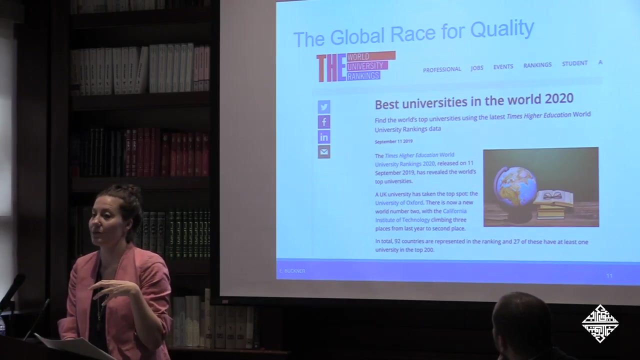 That is the discourse: that we need highly educated, highly skilled workers for the labor market right, And so I think that's a really important point, And so this discourse really positions nation states at the sort of national level as in competition with one another. 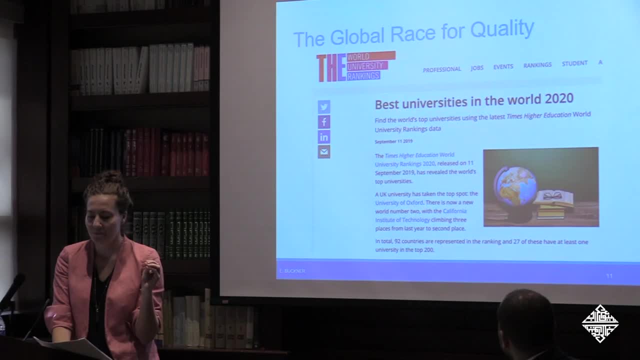 That's like. the overarching message is that we, like at the national level, competing with one another for scarce resources, including scarce human resources, meaning highly skilled individuals- And so supporting higher quality at the by a government or at the by an institution is, in many ways, signaling the desire. 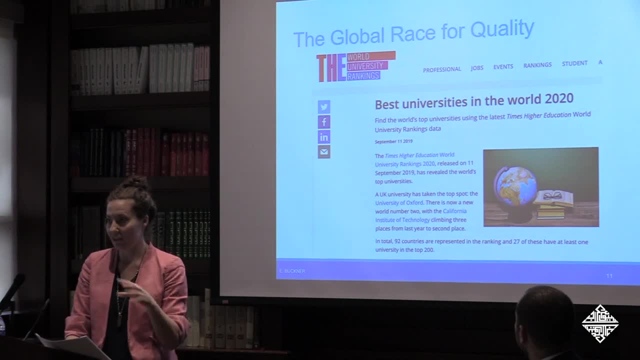 to participate in this knowledge economy, A willingness to do whatever you know it takes to participate, and then ensuring that you will be continue to be economically competitive. And so there's no. there is no definition of quality. If you study quality from an educational perspective, 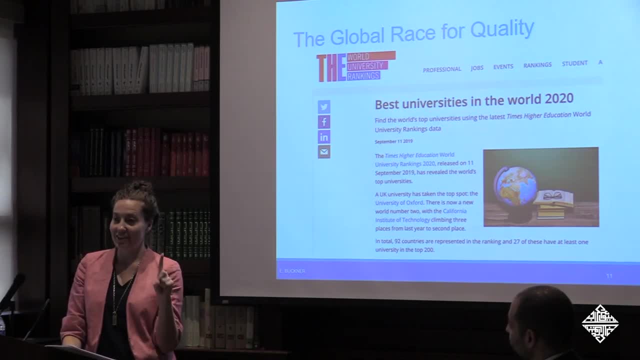 literally, there is no definition. I mean, UNESCO has tried and they're. they have conventions on higher education for the 21st century and they have quality assurance. you know books, very large ones, And so, for example, in 1998, at the- you know higher education convention, 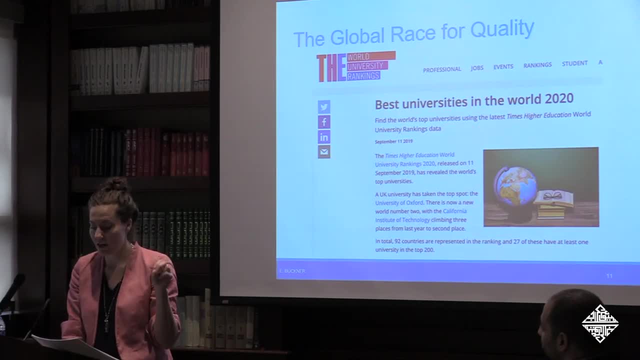 UNESCO defines quality as a multidimensional concept that must encompass- quote- all functions and activities of higher education, including teaching and academic programs, research and scholarship, staffing, students, buildings, facilities, equipment, services to the community and the academic environment. all of that. 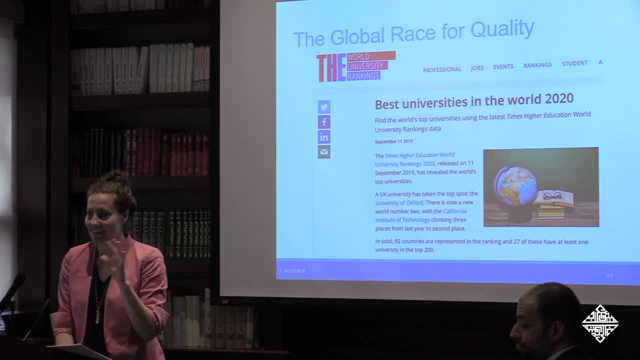 And I mean obviously that's very vague, right and very comprehensive at the same time. And I mean I would say that we in education are very skeptical of this and would say that if you think about who gets to be high quality, it's institutions with lots. 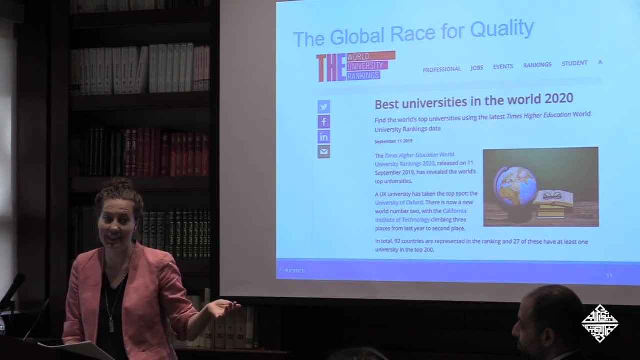 of resources that are have, that have been historically institutionalized over many decades as having those resources right and the and and there's, you know, skepticism to the newcomers who want to have those, that quality and those resources instantly and overnight right. 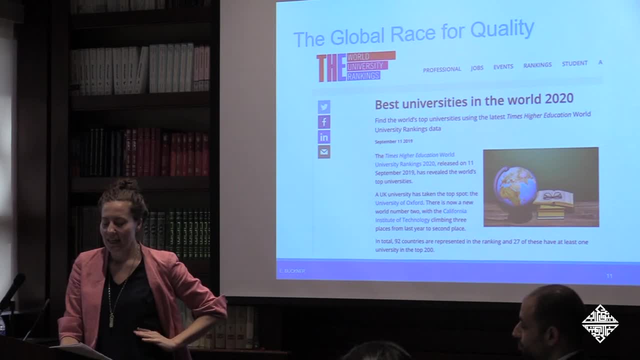 like in the Gulf. But so, in the absence of this clear definition of what quality means we, there are a number of different approaches, but one that I would say is dominant everywhere: is this proxy of using rankings right, and so international rankings become this proxy. 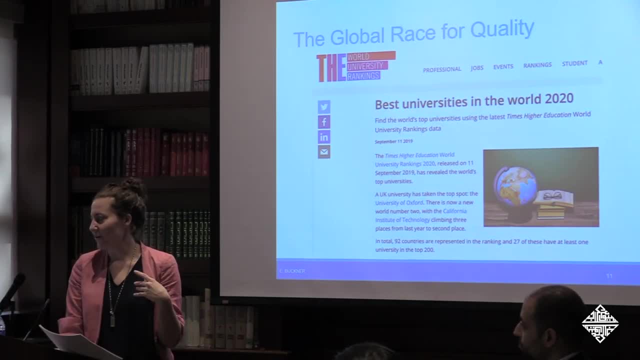 for who is high quality and who is not. And you know there's, you know there's, you know there's, you know. so we see this. the Times Higher Ed has put out their own rankings. there's a number of ranking systems if you study this. but, and then every institution that's. 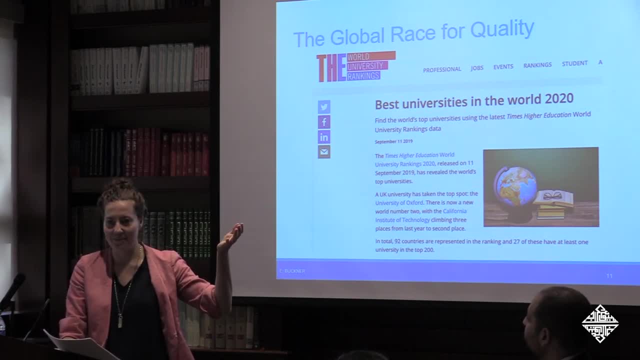 in the top 500 gets to advertise it. you know, I was at AUB and they have a big banner saying that their- you know, their- medical school is this ranked. this is on the QS rankings and then you know, in the the Times, Higher Ed is a UK-based ranking. 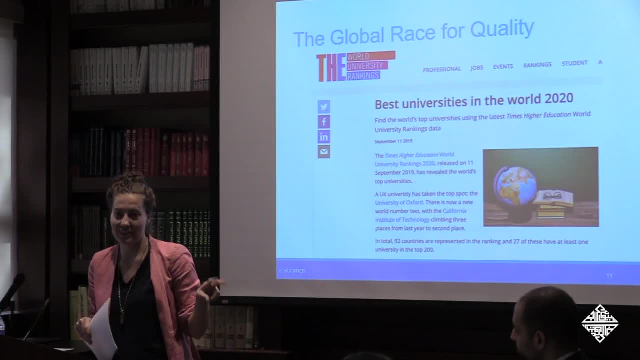 and it specifically gives more weight to international students and international faculty, where UK institutions do very well, and so the UK institutions always look better on the Times Higher Ed than they do on some of the other, like the Shanghai list. but this, so these rankings, are, you know, sort of affecting institutions all around the world. 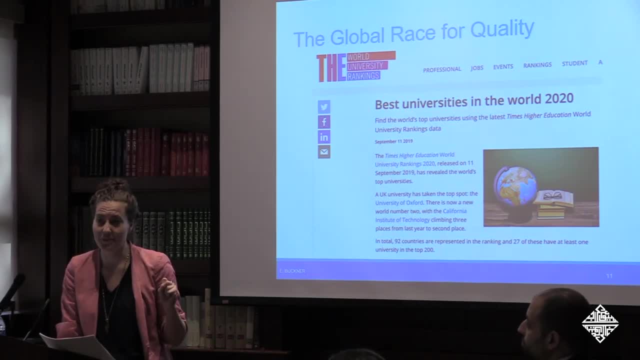 but they're also being used to criticize the R world. I'm not sure if you guys have read any of the critiques of these, but they are always sort of used to like indicate this general thinking that Arab universities are falling behind those. 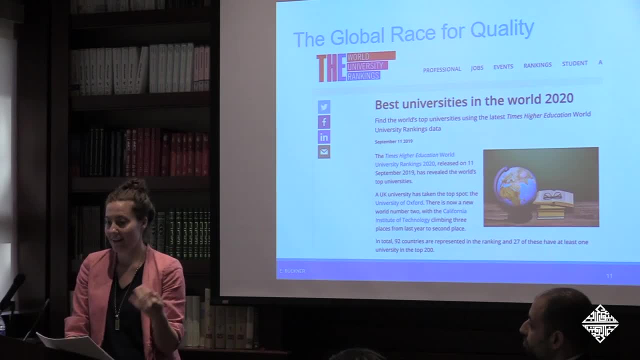 in other parts of the world, and so back in 2009,. an Economist article explains this as a listing of the world's top 500 universities, compiled annually by Shanghai, includes three South African universities, six Israeli universities, but not a single Arab one. 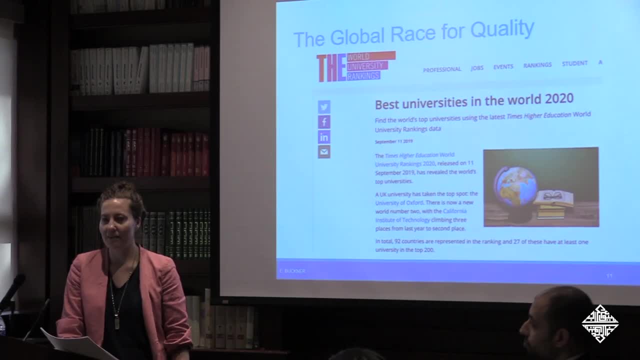 and then, of course, there's been some shuffling, but even in 2016,, the Brookings, a blog post by Brookings, echoes the same sentiment, stating only two or three Arab universities are in the list of top 500 and none are in the top 200.. 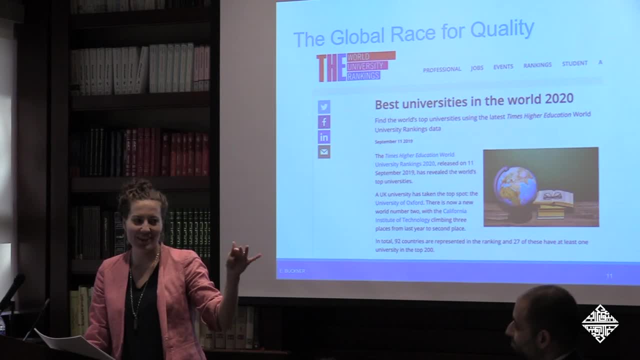 And so, you know, they upped the bar. now there are some in the five, the top 500, but that's not good enough. there are still none in the top 200. And so this is just one example of how this course of competitiveness is being used. 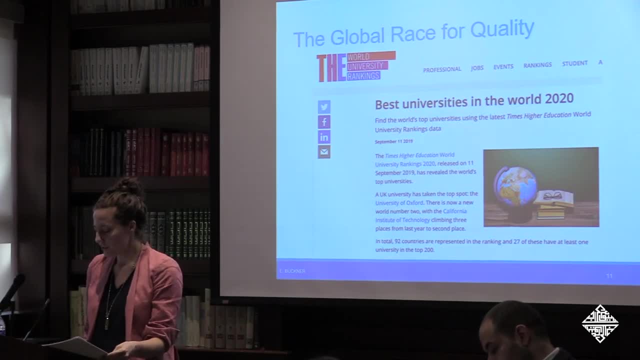 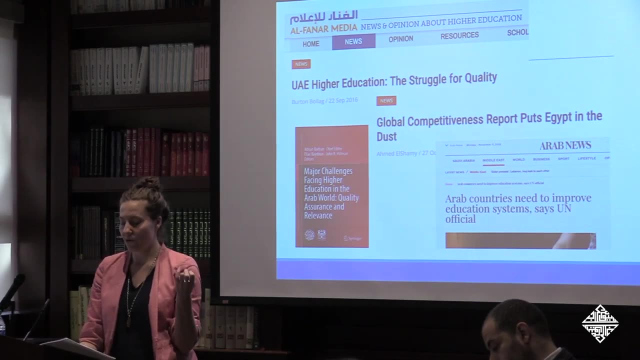 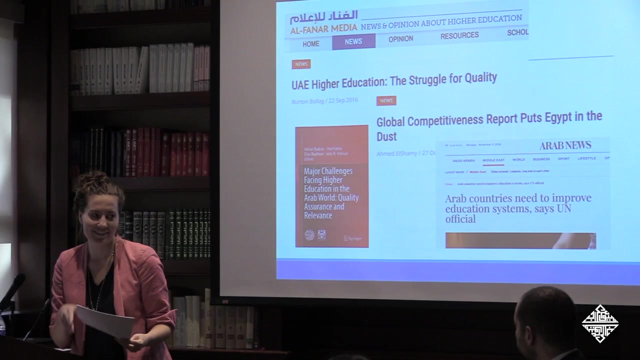 but I would say that, if you, it's also really widespread in the region. for the past three decades, honestly, this quality has been decried in the local media and international reports, and so I just in my book, I mean I go, I have a series of these. these are just some newspaper. 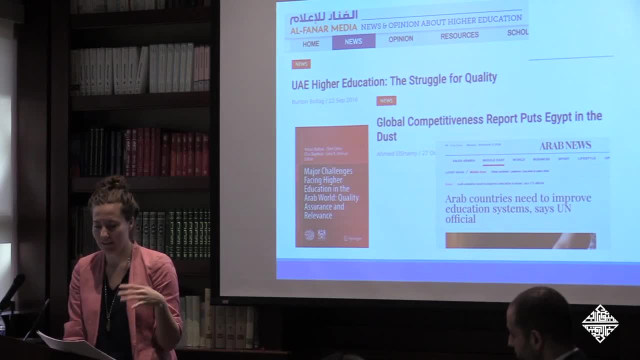 articles. but they're, if you actually sort of read the reports that have come out, like that. all the way back in 2002, the United Nations Development Program to NDP in their Arab Human Development Report. state of the Achilles heel of education in the Arab world is quality. it's the flaw that undermines any 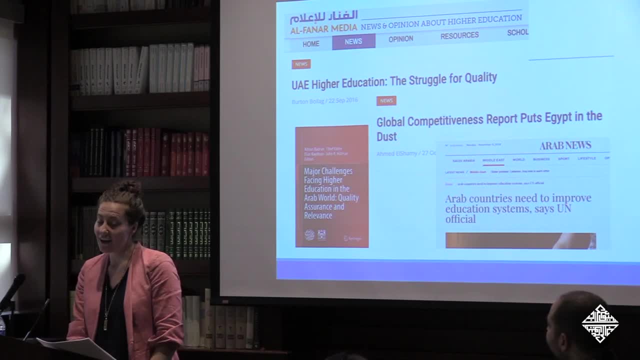 quantitative and then by 2005. the sort of updated version of the Arab Human Development Report maintains this emphasis on poor quality. it says the lack of knowledge capital is the main long-term problem based by the Arab world, and declining quality is the most important factor in the development of the Arab world. 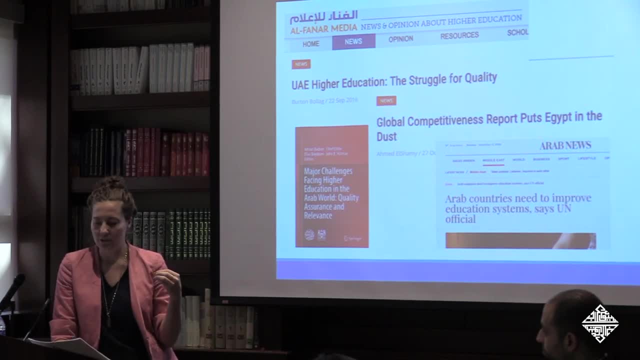 The challenge faced by Arab education and you hear this like over and over, in 2013, the Center for the Mediterranean integration, which is a project by the World Bank, and we reiterate the same idea: the divide between education and employment has not been bridged and the quality of education continues to be. 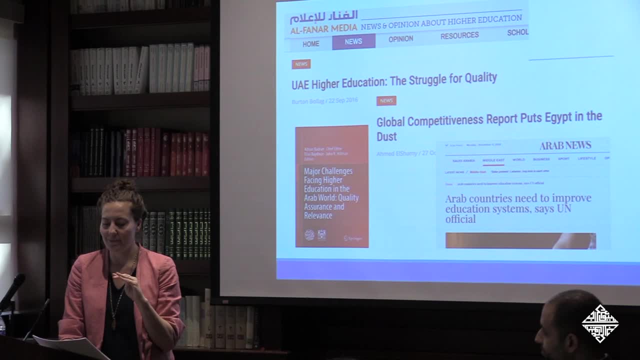 disappointing. this is just. I mean, it's everywhere, it's. and I would just say I, you know, we cannot deny I think that students are fresh, I mean like young people are frustrated and that are really high unemployment rate. the point that I am going, that I will. 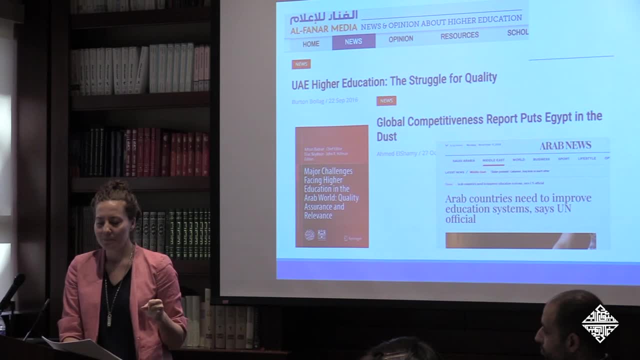 continue to argue in my book and in this talk is that the we blame higher education for that, and I think that is where the blame is often misplaced, rather than looking at the labor and get them a structural constraints in the labor market. and so I'm not denying that height unemployment rates are a source. 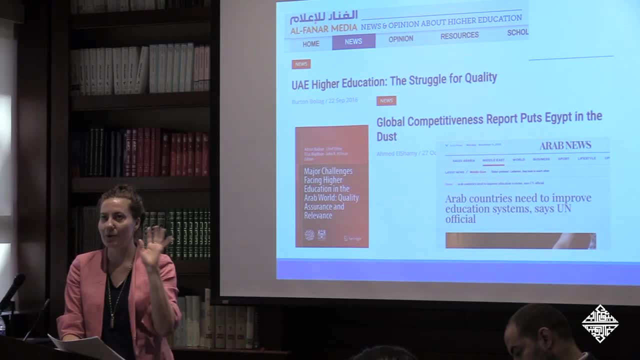 of frustration. I just think that it's not the airport is not alone in this, these frustrations, and that it is that there's only so much higher education as an institution can do, and then in many cases it's a we're looking, we're thinking about problems in the labor market, and so that's sort of what I do. 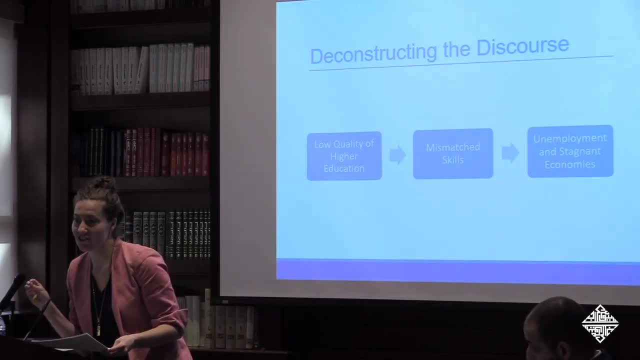 in my book. is I really deconstruct this discourse? what is this discourse really saying? and I would say that this widespread consensus that higher education suffers from low quality is actually a series of arguments which you can deconstruct, and each one of them is flawed in its own way or it's overly. 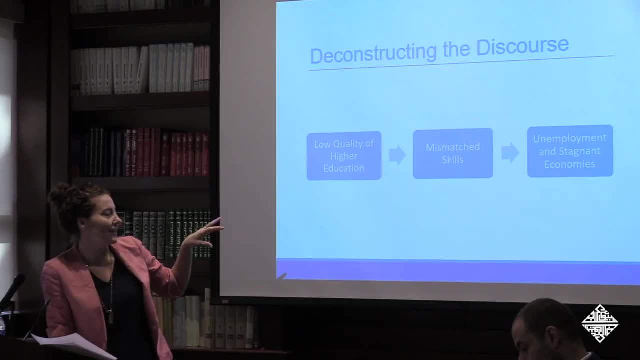 simplistic, I would say so. the first one is really that there is no quality. just take that as a gram, like the quality is well, and what that means is really that that offerings are low, the outputs of the higher education system are poor, and this often it means like: oh the class. 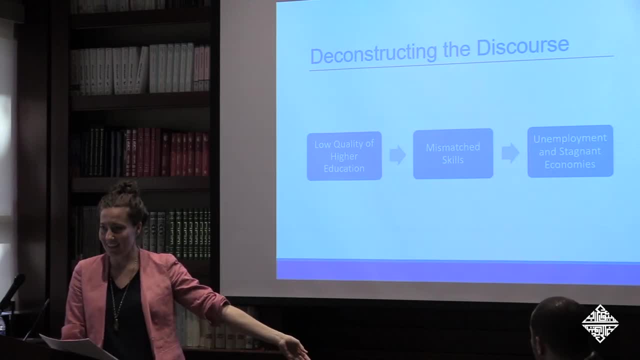 sizes are really really large. students can't find a seat in their lecture hall. there are few resources right a lot of times there. it's a very quantitative measure. it's like okay that, how many books does the library have, etc. what we need to sort of think about what it means to have like low quality students. 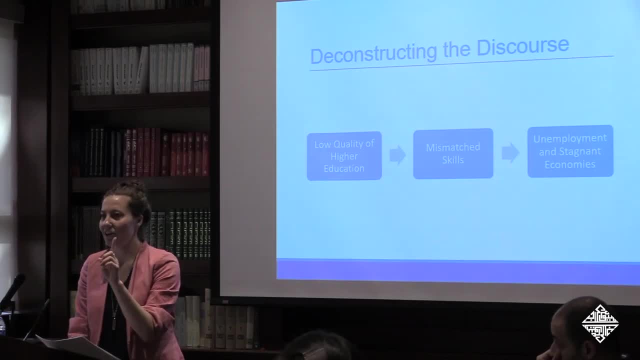 aren't learning very much. oh, that's also. there's a big emphasis on professors. pedagogy is right like: oh, it's all about quality. it's not about quality, it's all about memorization. the students aren't learning how to be critical thinkers. that's a big common theme in this as well. and then we move from that to say: do impart or do. 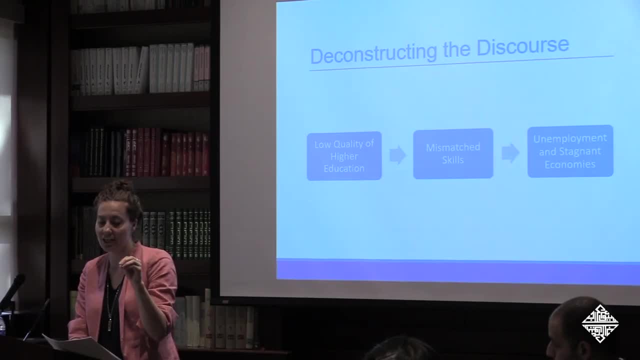 primarily to this low quality output of the higher ed system, that then there is clearly a mismatch between the needs of the labor market and the skills that graduates have, and then, naturally, it is this mismatch that is to be blamed for sluggish economic growth and high rates of unemployment, particularly among youth in the region. 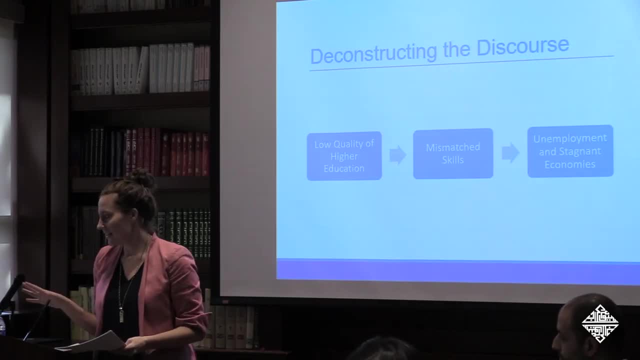 right, and so the one. so one of these critiques, or especially focus on this mismatch, is that, okay, there are too many students who are concentrating in the humanities and Social Sciences. I'm not sure if you guys have heard that one, but it's very common. in 2008 report, the world bank explains that one of its 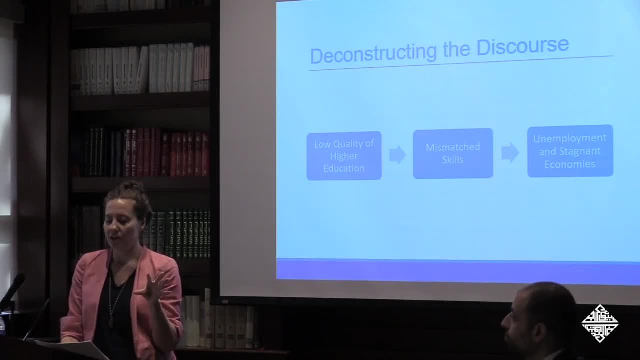 measures of quality is the proportion of all undergraduates of all university majoring in the STEM fields- the science, technology, math and engineering. and this, this is a direct quote. it's underlying assumption is that, quote: scientists and engineers are likely to contribute more to economic growth than our social. 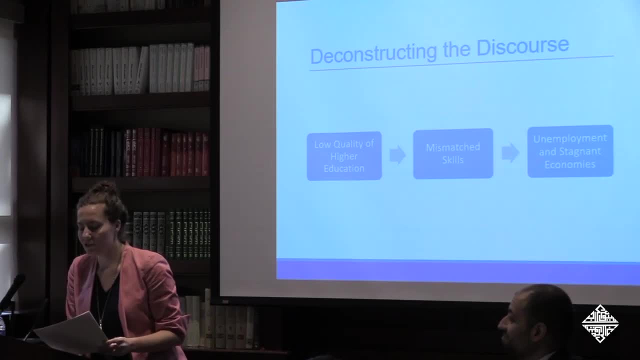 scientists and students of the humanities because of the increasing importance of technological innovation and adaptation in development. and so, to support this claim, they cite a study from 1991, 17 years before the study itself was published and while before the spread of, like computers, the internet, etc. and actually I mean you may take this statement for granted, it might. 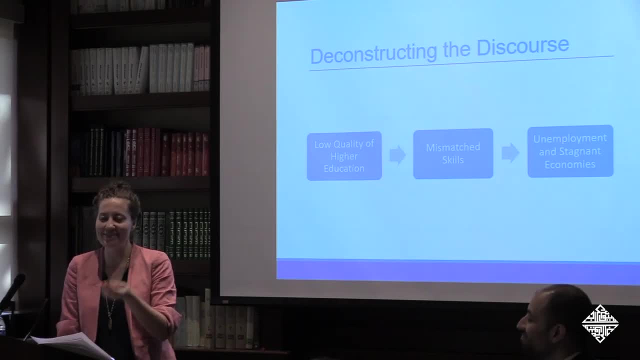 be common in that sort of- I mean I hope not, as masters of you know Arab studies, but the but a lot of the economists are. I mean there's a lot. this is not proven fact. that would say, in fact, there's a lot of really interesting literature in. 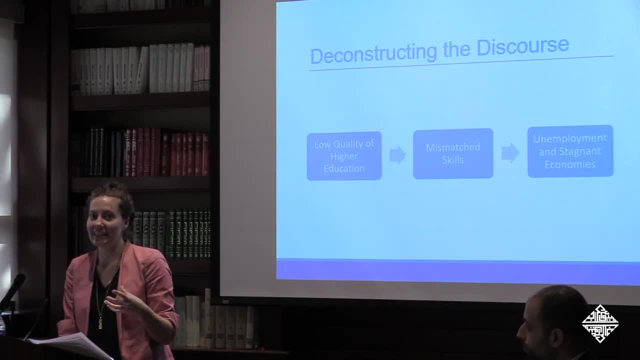 the economics of Education. that's actually arguing. you need people like the social, scientific humanities backgrounds to know how to adapt technologies and change them right, and so this is first of all, not taken likely like as fact. and then the next point that I would just think is the claim: 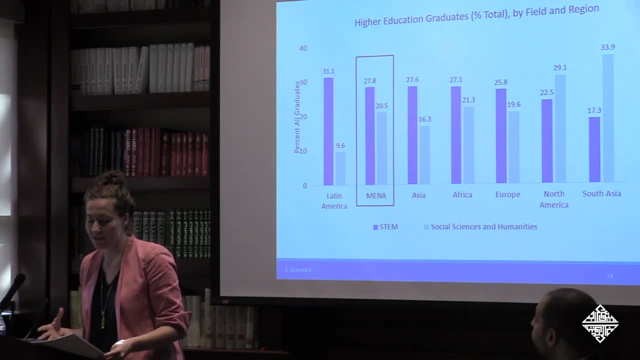 that too many students in the Middle Eastern North Africa- I'm majoring in the Social Sciences- and too few in the sciences and too few in the social sciences and just the freedom community of people and a much larger number of and the STEM fields is also not proven. 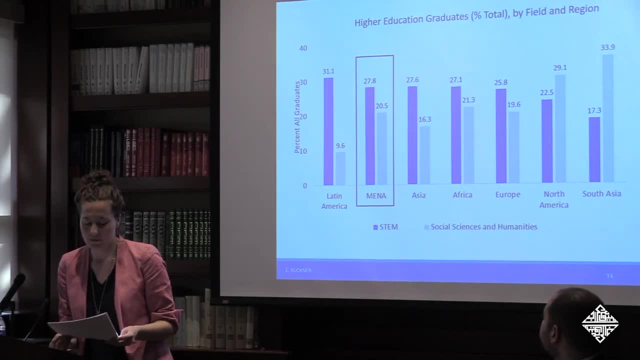 I mean, this is from the most recent data by UNESCO and if you look at this, we see that this is at the regional level. the Middle East and North Africa actually has one of the highest proportions of students graduating with STEM degrees of any world region. 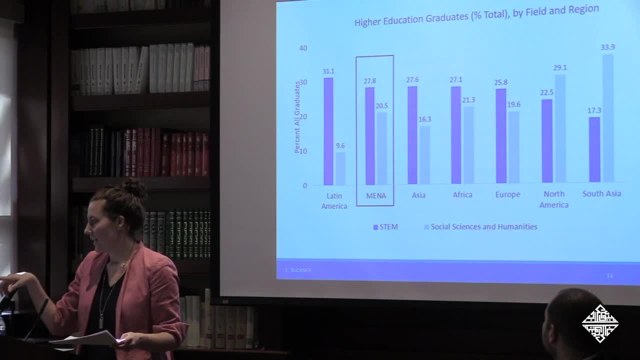 It's actually very close to the global average. It's higher than what's very equivalent to East Asia. Asia here refers to East Asia, where East Asia is seen as a region that is doing things right in terms of economic development right. it's a rapidly growing economy. 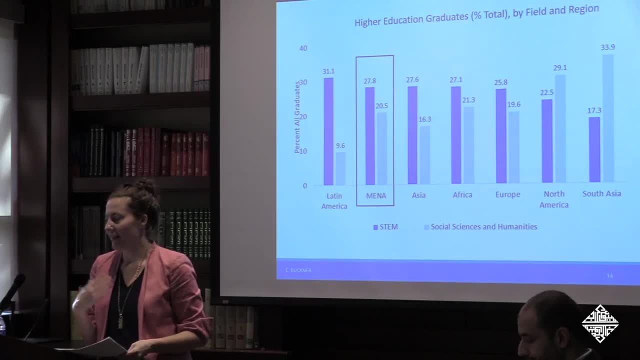 And it's actually higher- we have more in STEM than in Europe and other places. And so, first of all, I just don't take these discourses at face value, because they're very clearly substantiated with actual empirical evidence. And then 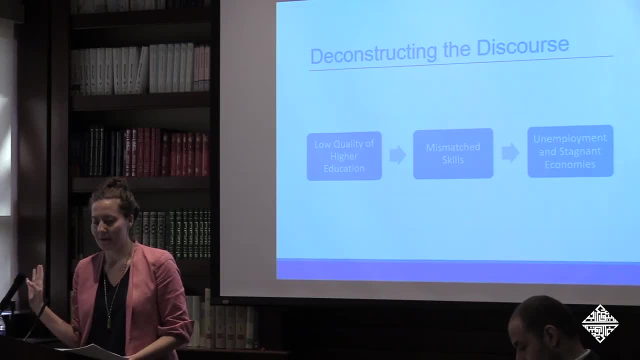 if you move on, then this unemployment and stagnant economy is almost always the thing that's placed on higher education right. It's this low quality and this mismatch that leads to unemployment, And unemployment is the real crisis, because- and this is often rooted in you know- 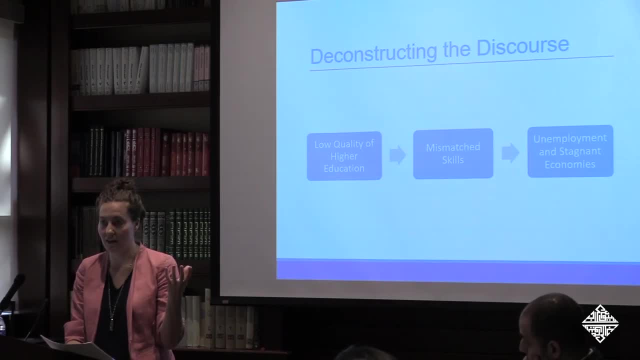 sort of concerns about the destabilizing effect of young people, particularly young men, right And so. the 2002 Arab Human Development Report refers to unemployment as the scourge of joblessness which affects Arab countries more seriously than any other developing region. 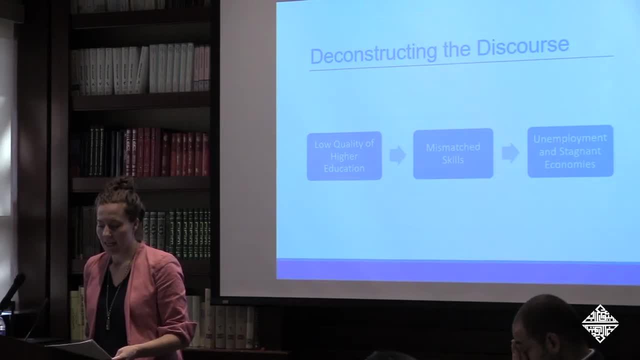 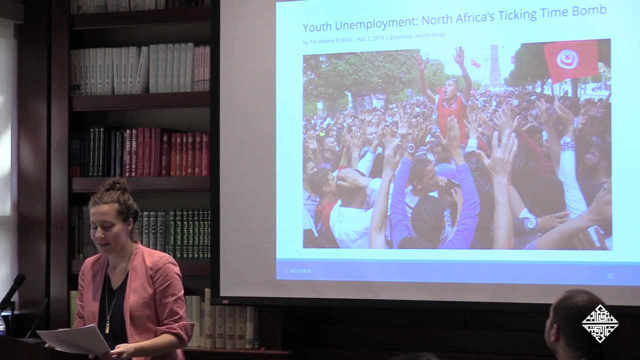 And it points to high youth unemployment rates as sort of like the natural sort of as a crisis It's called, you know, like a ticking time bomb and other sort of destabilizing consequences, And actually this is almost always blamed on higher ed. 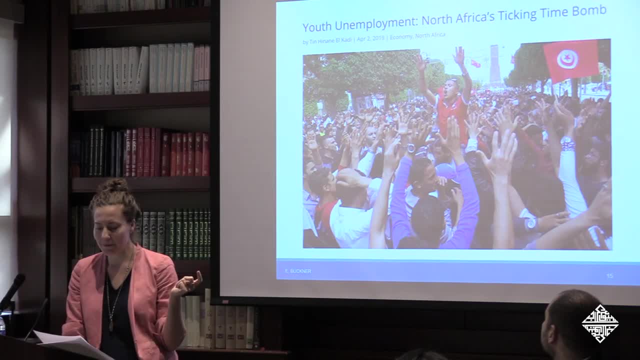 for example, one report by the World Bank says there are no proper signals sent to higher education establishments in terms of which skills are in demand and which skills are not in demand, And so, as a result, the graduates can't find jobs. 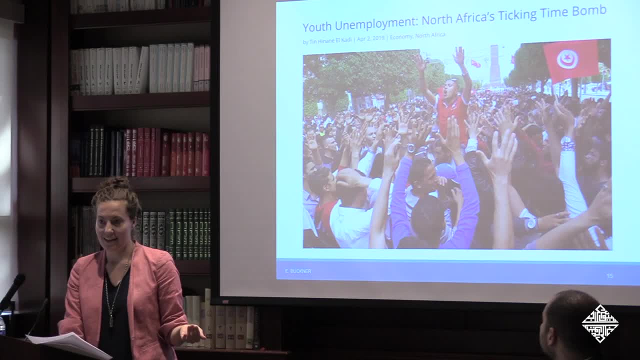 And then they actually call for like better data so that families can do a better job of informing students and parents which degrees are actually in demand, et cetera. But if you know anything about how admissions work, like that is really ridiculous, because many students don't choose their own degree right. 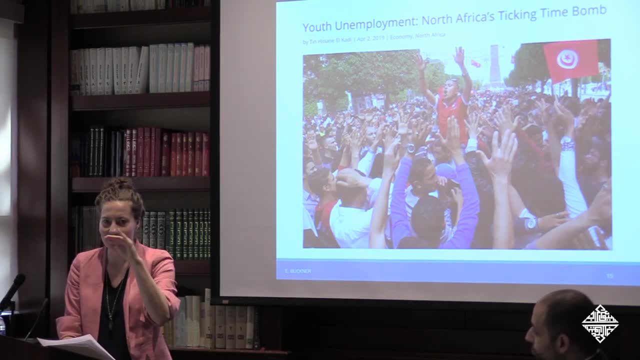 They only get to study what they have a sort of you know based on their score. they're sort of slotted into a particular degree program, And so these, so my point around these are like the technical literature that I summarize in here- paints a very linear. 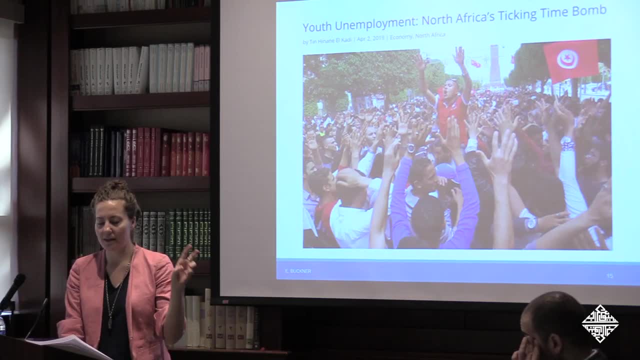 very simplistic equation between these low quality, misaligned incentives and then clearly causing high rates of unemployment and stagnant, stagnant economic growth. and so this is, I mean largely because the lens is one of human capital theory that just assumes that the ultimate goal is employment and that if we have high unemployment then it must be because we 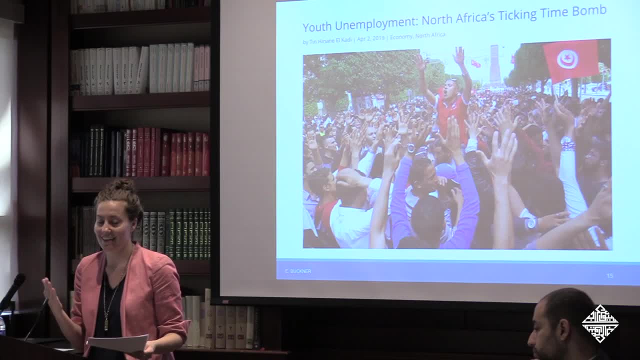 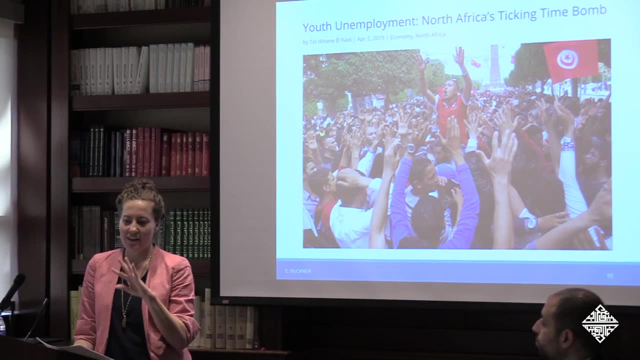 have a failing higher education system. it's sort of that backward causality that I really take issue with, and so, moving on from this, like: so the crisis is very clear, right, the the crisis rhetoric has been set up for decades, and so, given this all consuming crisis, right, you have governments that are actively 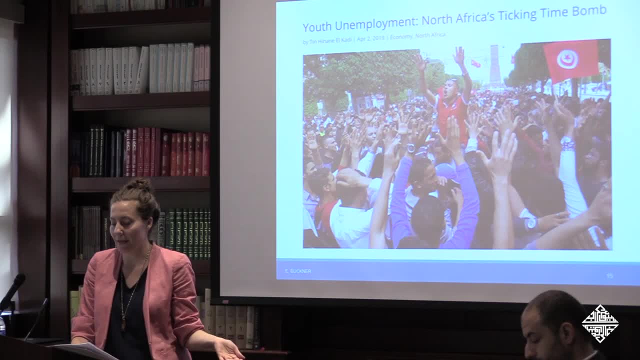 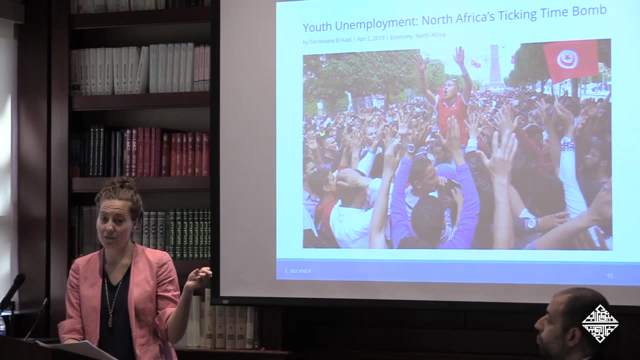 trying to address the higher education quality in in many ways, right to the extent that they can, and so some scholars have actually argued that this crisis rhetoric is useful in a political sense, because it's trying to create constituents and motivate different interest groups to push for a reform, and 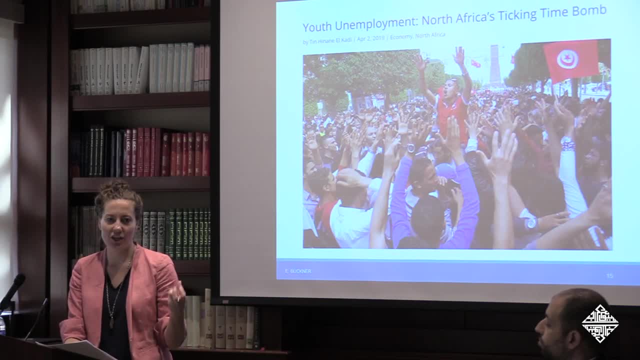 so. So Egypt and Morocco have used a crisis rhetoric to try to bring together a consensus on reforming higher education And then, when these consensus committees often stall, development agencies, particularly the World Bank, has played a very influential role in pushing reform. So throughout the world, not just in the Arab world. 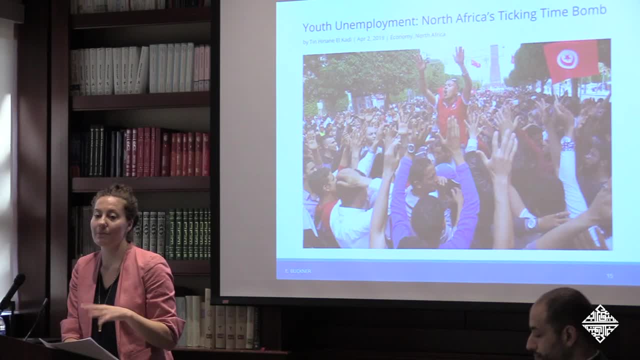 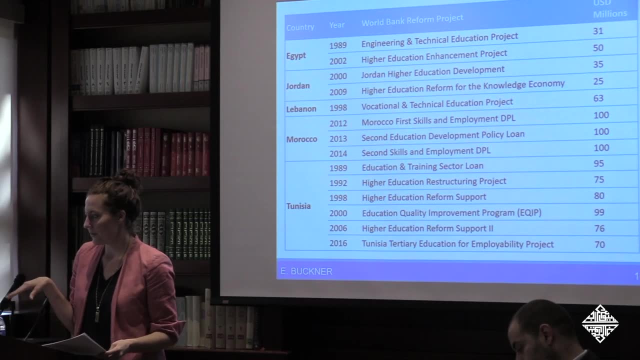 the World Bank is the largest funder of higher education reform throughout the world. They really have to tackle it, And so in my book I just look at what is the World Bank doing in higher ed, And they're really funding large-scale reform. 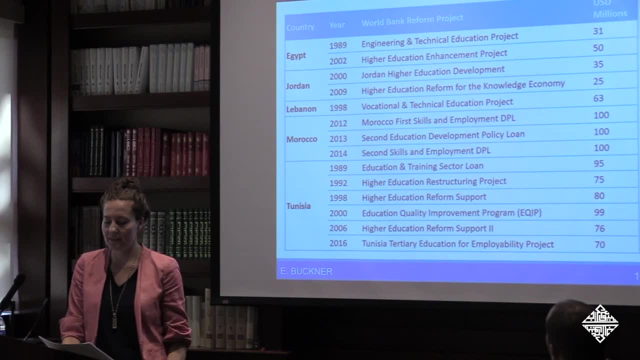 in many cases, that's government-initiated, government-led at least, And this is happening in Egypt, Jordan, Morocco, Tunisia, And they're adopting very generic approaches. They include like: let's expand private higher ed, Let's create quality assurance. 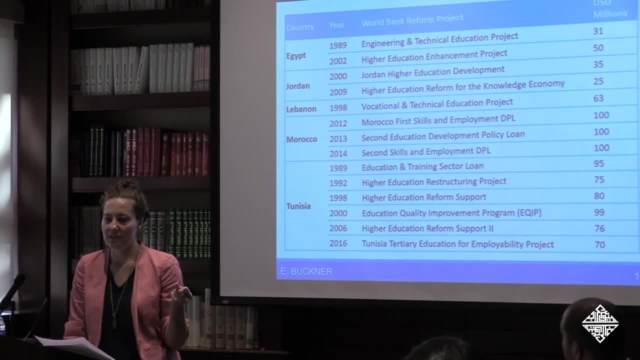 And in some cases, like in North Africa, this was done by mapping degree reform onto the Bologna reforms that were being undertaken in Europe as well, And so the result of this: this outsized role that these agencies are playing means that they have very technical approaches, so that these 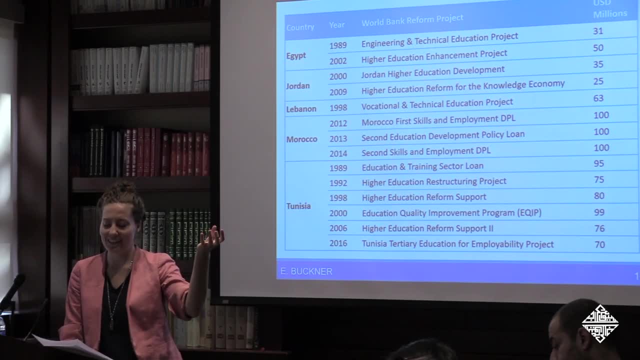 reforms. They're like: OK, let's add in, Let's create a new quality assurance agency, a new bureau, Let's create an accreditation council tower degrees accredited, Or let's sort of have new minimum standards, for example. And so essentially my main point here: 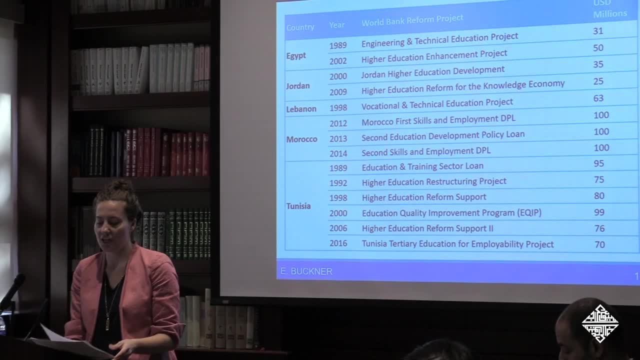 is since the 90s the World Bank has really funded numerous higher education reform projects that are generating resources to reform higher ed in the sort of middle income countries of their region. But what's going on in the Arab Gulf is very different. 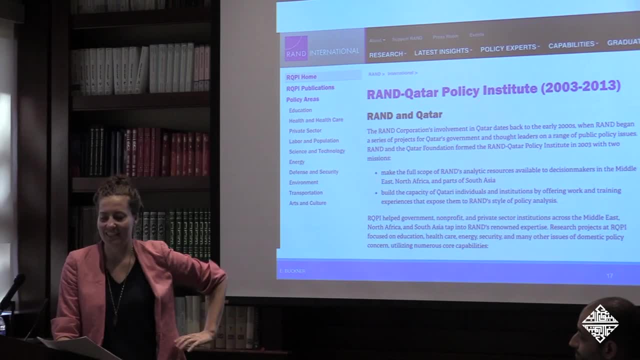 So I also look at sort of what's going on in the GCC And obviously, rather than relying on World Bank projects to secure external funding and be able to have high profile major restructuring, the UAE and Qatar have taken a very different approach. But what I point out in the book is: it's not that different. 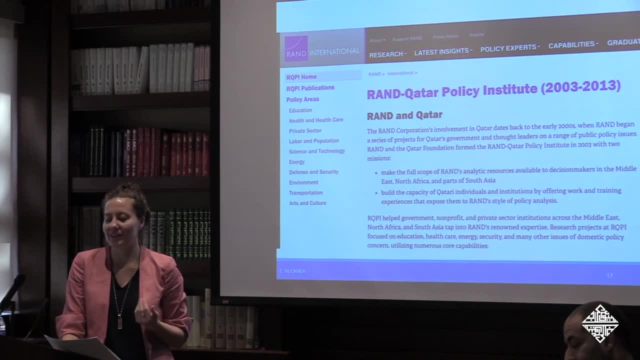 Right. They've also brought in external consultants to align their higher education systems to what we call the global best practices Right. So in the UAE, they established the Commission for Academic Accreditation, which is seen as like a best practice in the region. 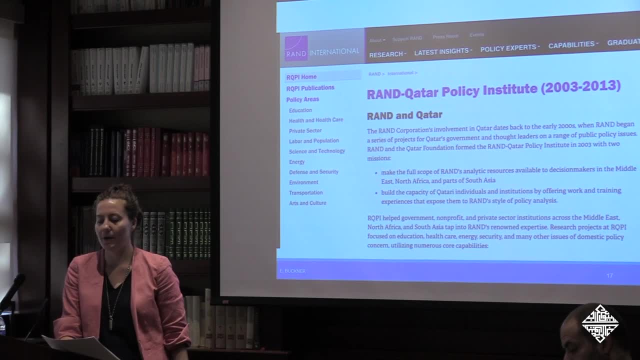 because it's a fully independent body that's supposed to license both the public and the private universities and accredit their academic programs. And then, almost more than nearly any other country, there's Qatar, which has, I think, put its faith in its external technical experts. 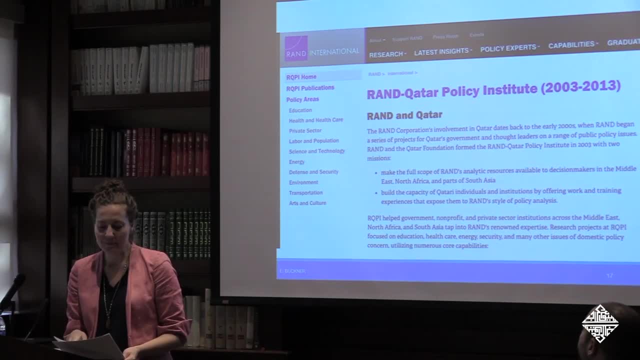 to reform its education system. So I'm sure many of you know about this, But RAND's work in Qatar was not only at the K-12 level, It was also reforming Qatar University Right. So in 2001,, the Supreme Education Council 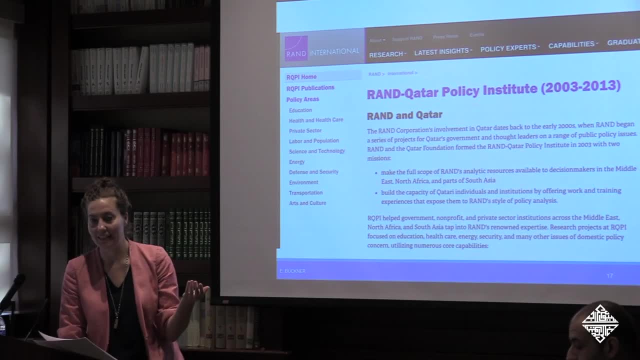 commissioned RAND Corporation, which is an international think tank based in, to advise and oversee its major requirements, And so, if you look at what they suggested, they were largely reflected. the fact that they're located in the United States Right That a lot of their reform models. 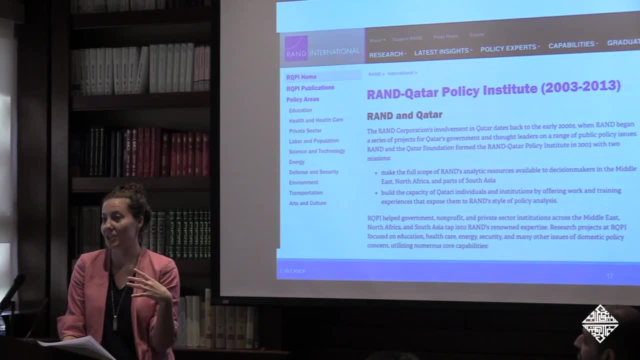 are very similar to the ones that we have dominated education policy in the US, such as introducing independent schools which are sort of like charter schools in the US system and publishing a school report card. Again, that very, you know, important. 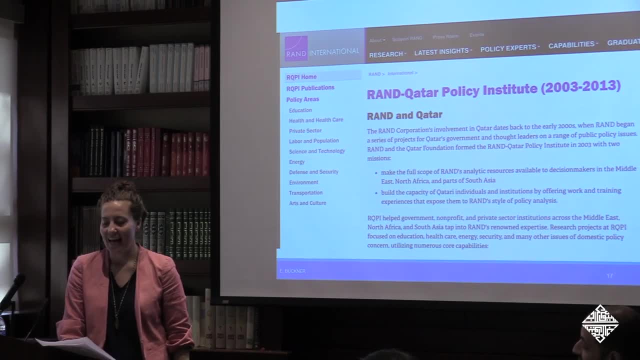 It's a very American idea of what it means to assess quality And then also switching the language of instruction and science to English, Right. And so then, when you look at the reform of the university, so the administration of the university had to make a decision. 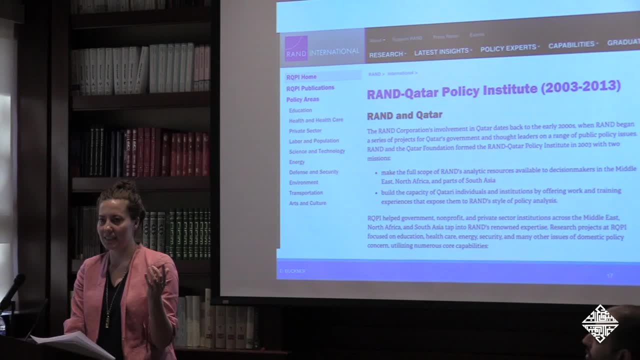 They wanted to sort of reform the university very quickly to become what they call high quality, Where I would say that in this, If you want a simple definition of high quality, then rigorous is a good one. Quality often is being mapped onto like rigor. 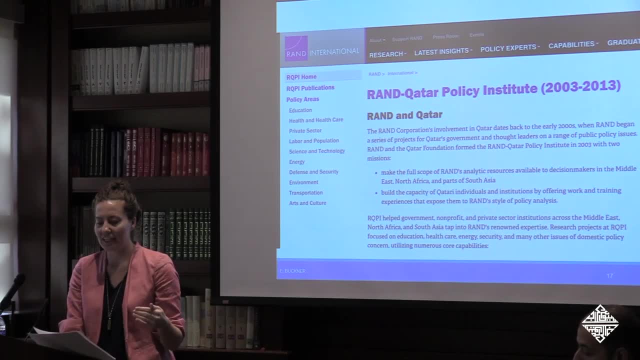 Right, So let's have higher standards essentially, And so, when we think of quality in that way, in the book that the brand wrote afterwards called The Reform of Qatar University, they explained that they were really faced with a choice. One was preserving the status quo. 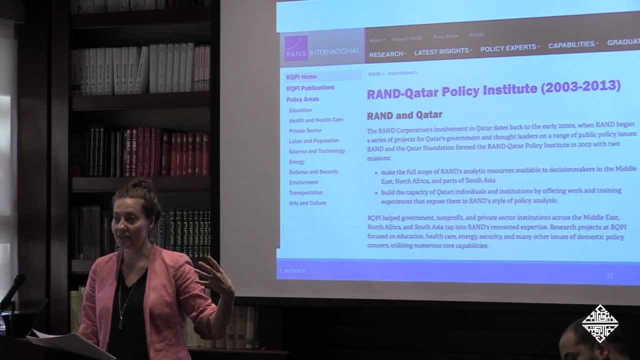 in which a university education was available to all nationals, as the sort of free public university, national university, Or, literally, this is posed as a dichotomy- upholding academic standards. That is the way it's phrased: Either all or upholding the standards. 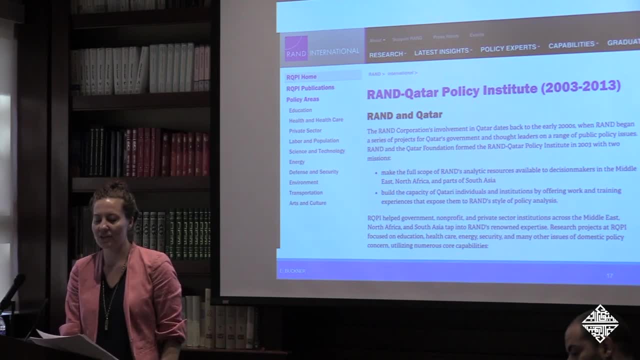 And so the administration decided that Qatar University would uphold its new standards and aim to serve only average and above average students Right While expanding the preparatory foundation program to sort of compensate for the higher level of language skills and whatnot. And so the key recommendations they made: 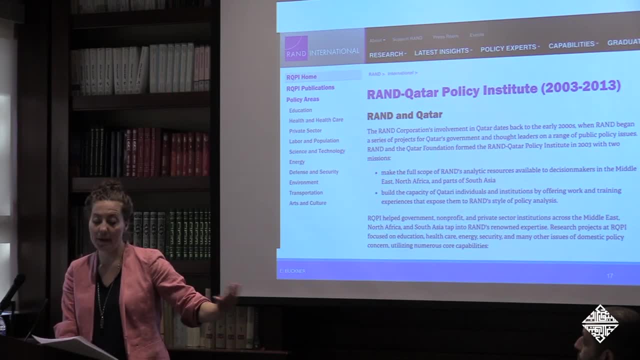 were: let's standardize admissions requirements, Let's set minimum standards for retention, Let's have higher academic regulations, et cetera. And so what I noticed from these is they really focus entirely on students. It's all about student preparation. It's all about student preparation. 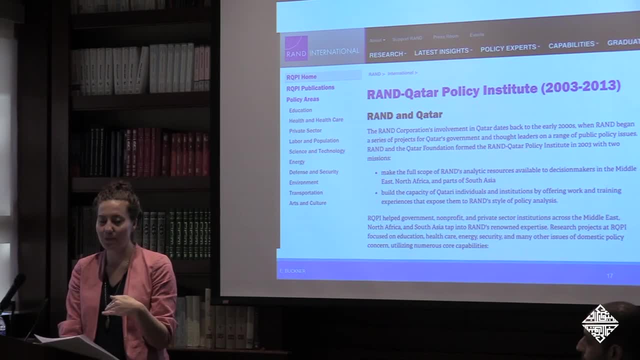 to get into the university. They're not addressing students' supports for learning once they're in at all, And they're not really addressing what's going on in the classroom either, And so the point that I would make is that upholding high academic standards sounds good. 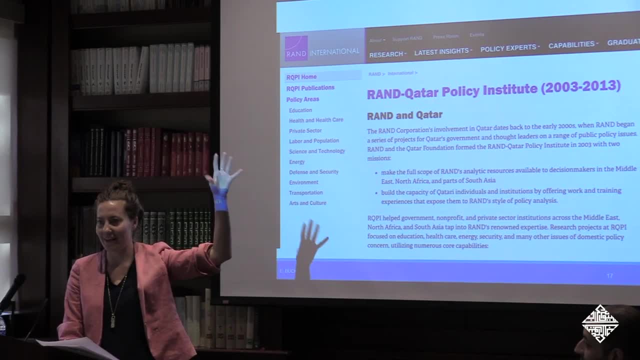 We believe in that. That's banners. We put that on our banners in high school. It's like high standards for all, But it sounds like we're going to have to do this. It sounds like perfectly legitimate policy And it sounds like a good thing. 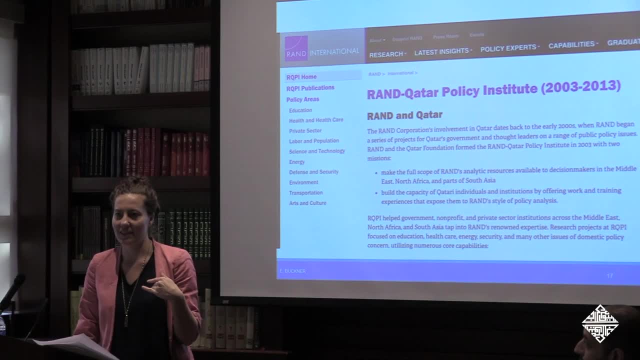 And that's sort of the way in which these discourses are. sometimes they become so pervasive and unquestioned is because they sound good, right, But in reality what they did was they excluded a lot of students And as the only place you could go to university. 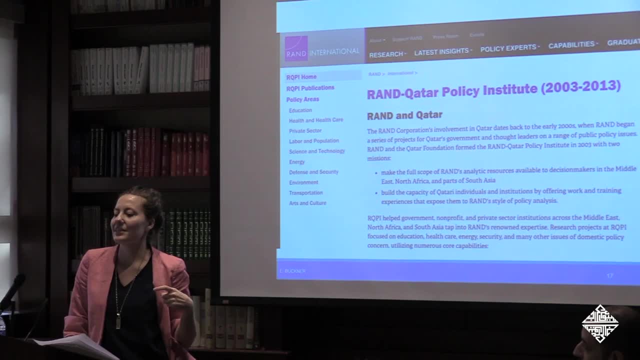 as a citizen. many families found that their students literally didn't have a place in the university system at all, That they couldn't access it, And that disrupted the existing norms and the expectations of families, And so I did interviews. They are asking, and one of my respondents was explaining. 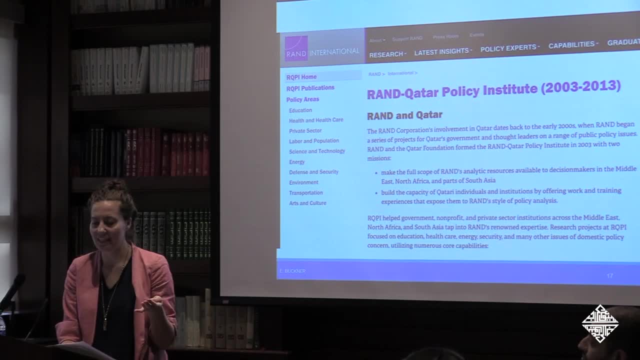 well, they revamped Qatar University between 2003 and 2006.. And the plan was, to quote, transform the institution. But what it resulted in is that families found that they didn't have a place in this new system, And so there was resistance. 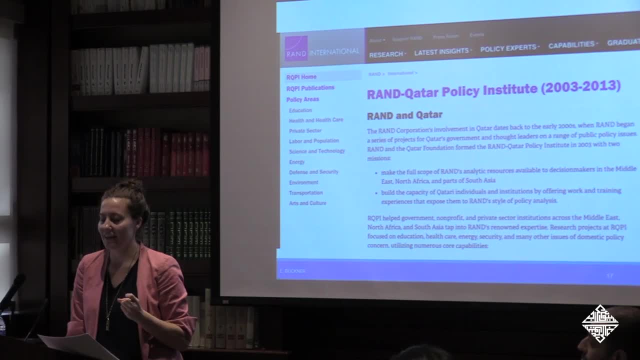 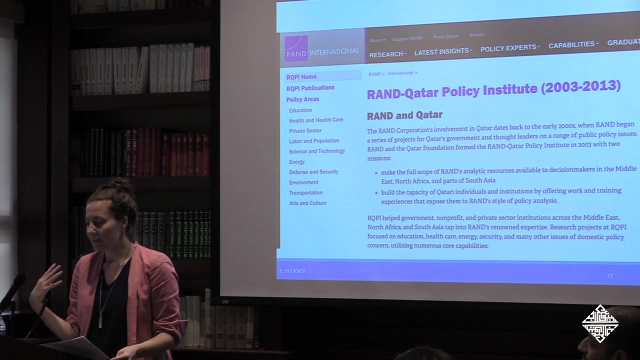 There was complaints And the country's leadership realized that they disrupted society too much. It was too much for society to absorb Because, at the end of the day, the main audience for reform is citizens. And so now, from the outside, compared to that, 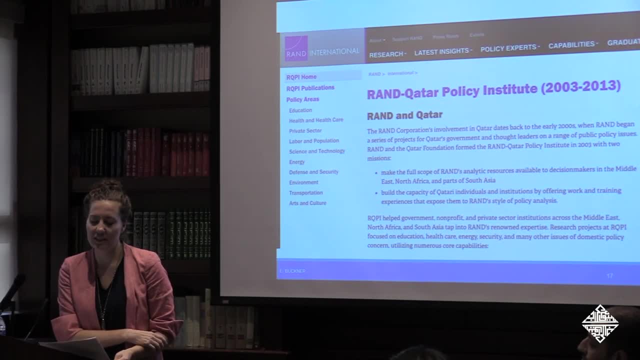 we really think of this. So in 2013, the Qatar Foundation formally ended its contract with RAND And this policy institute closed And we really in some ways see that And I see this as a model of what not to do. 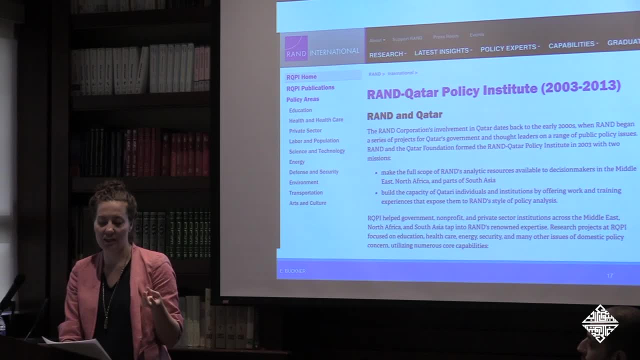 You can't really bring in external consultants to institute rapid change overnight and in their wake leave national citizens feeling like they had no place in this new system. And when I think about quality generally in higher ed, I often think that we all want high quality. 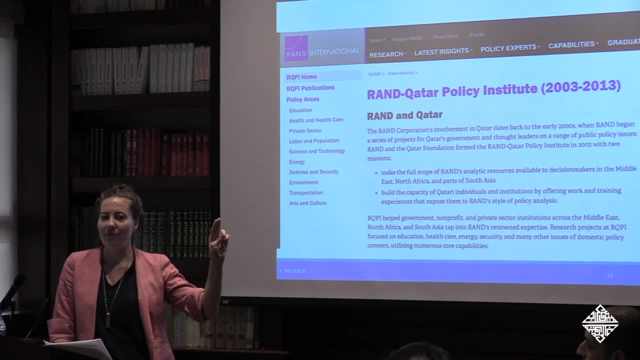 We all want prestige, But only to the extent that it doesn't exclude us. Nobody wants so high quality that they no longer get to go to You know X, Y institution, right, Or they don't get the access to the degree. 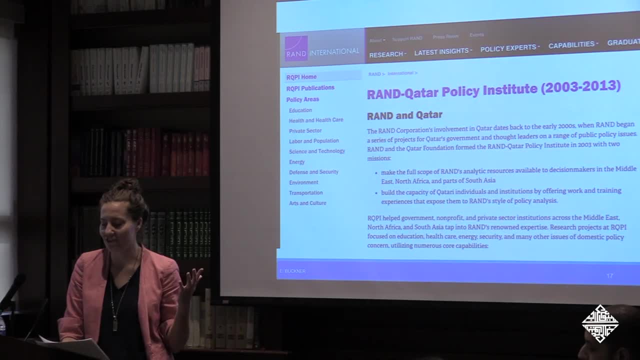 And I think that's a natural understanding. The resistance is natural, And so I don't think of these large scale quality assurance reforms as state projects in many ways that are aimed at securing legitimacy from a skeptical public that has been told its higher education system is in crisis and of low quality at home. 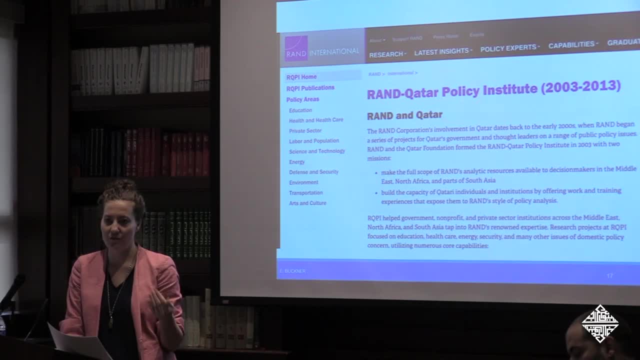 and then also abroad, in this knowledge, to recruit foreign capital and whatnot, foreign investment. And so the reality is, it can be very delegitimizing to acknowledge that the public higher education system is failing because these systems, the universities, have played such an important nation building. 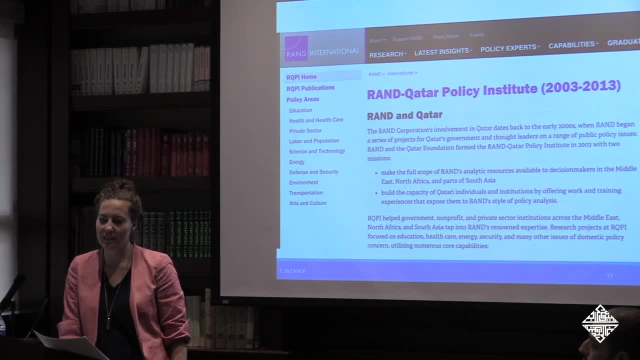 role for so long, And so, in the countries, this can often be massaged and done through major government-led reforms that are being supported by the World Bank, And so they're both securing finances. They're also signaling state investment in quality and a desire to reform. 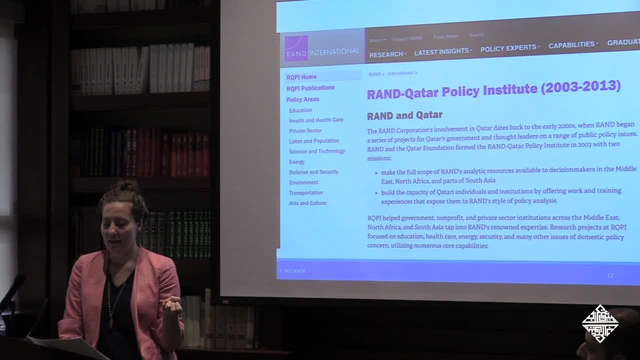 And then if you look at the case in North Africa, it makes a lot of sense that governments wanted to rapidly align to the new European system that was adopted in the early 2000s- the Bologna reforms- Because in many ways the citizens 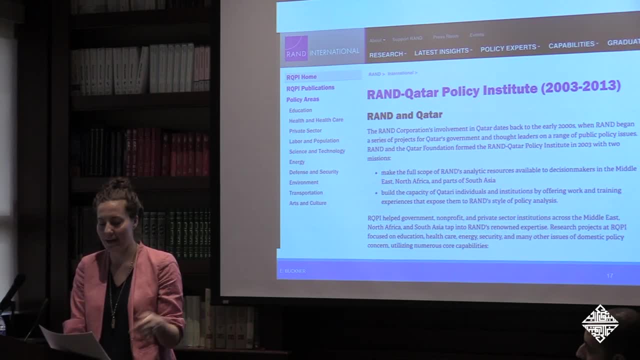 are interested in making sure that they can study abroad. in Europe, That's a natural progression for many upper middle income families in the region, And so, in contrast, in their Gulf states, quality assurance is not, of course, resource generating, But it has drawn up foreign consultants and think tanks. 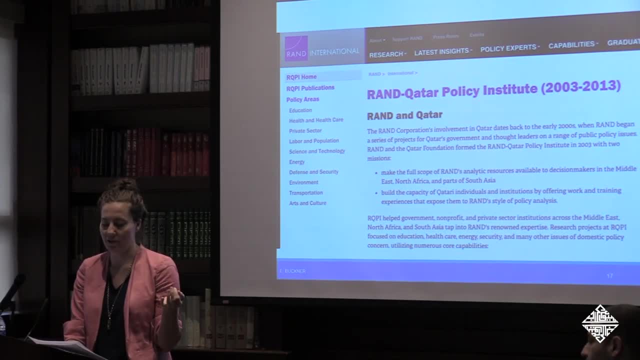 to align these Gulf systems to best practices in the US and the UK, And so, despite their differences though, the approaches to quality really look to external and foreign international models as blueprints for success, And it results in this sort of implicit encoding of quality. 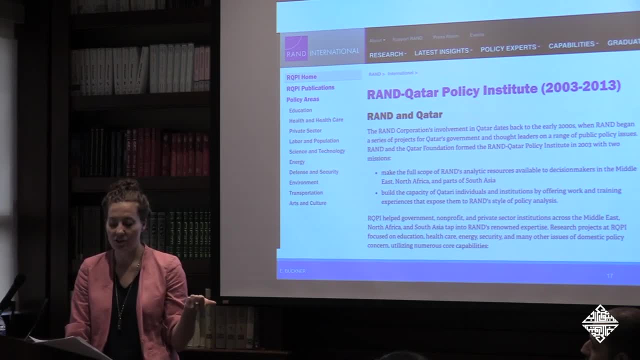 as foreign in ways that often don't really reflect the values of the state, And so it's really interesting to see how these reforms are going to play out in the future, And I think one of the things that's really interesting about these reforms is that they're 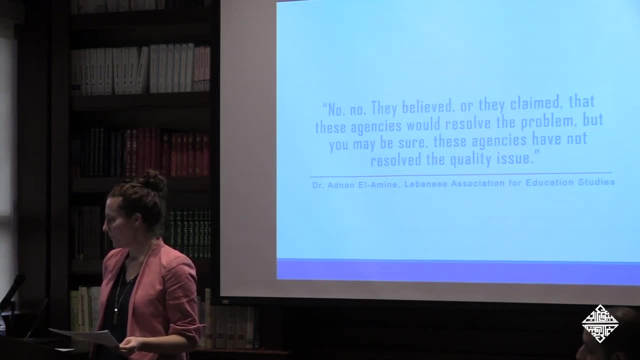 very much based on the ideas that often sidestep national policy processes. It really disregards local perspectives on quality or the interests of affected stakeholders who are really going to be affected by these reforms. And so, despite all of this huge movement to stamp quality on higher ed and these reforms, they've 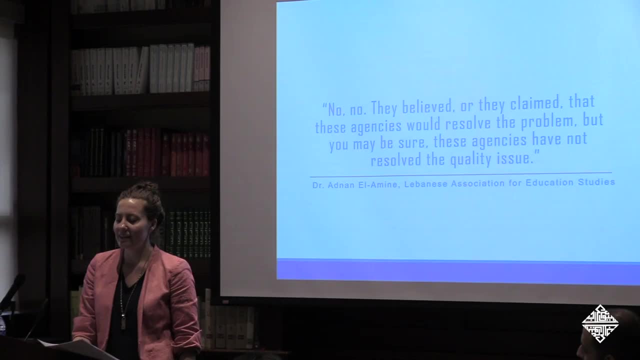 really been focused on the idea of quality And he was like no, no, They believed or they claimed that these agencies would resolve the problem, but you may be sure they have not resolved the quality issue. And in my book I really talk a lot. 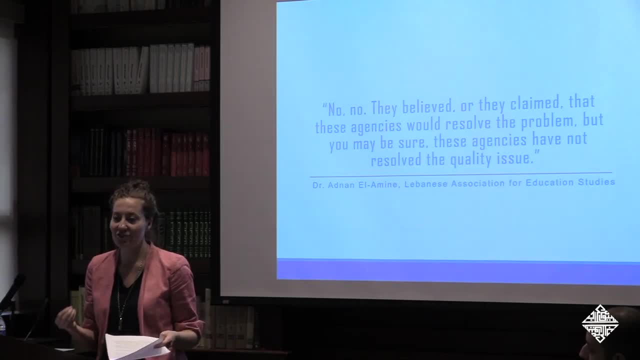 about the structural issues, Like undermining this desire are very real structural issues throughout the region. So, for example, when I was in the Gulf in UAE, one of the practices that many private universities are doing are national accreditations for their engineering programs. 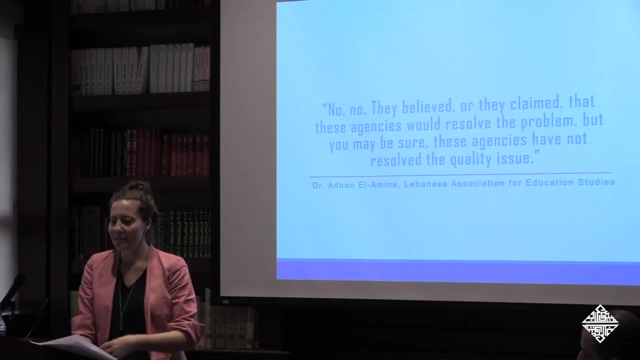 and like that, And I was talking to a faculty member and he was explaining that these are very time intensive processes. right, You have to submit all of your syllabi and you have your CVs and you have to show student work. 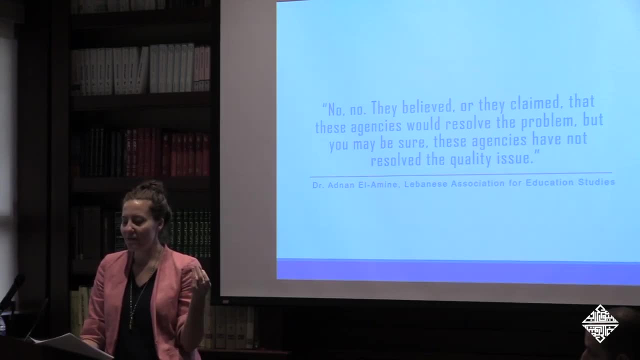 And they're very time intensive And he was like: well, the faculty have very little reason to participate in these because they actually operate in a situation where they aren't even with their. So they were. contracts are very unstable in many of the private universities. 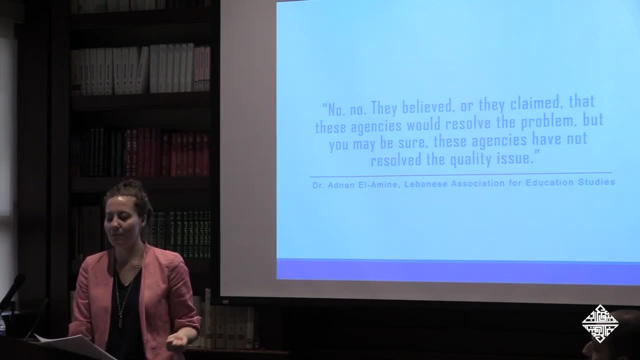 And so he's like. he says, why would we even worry about this? Students will be here longer than we are. At any point the university administration can cancel your contract and you're going to have to leave the country, And he felt like that really undermined his investment. 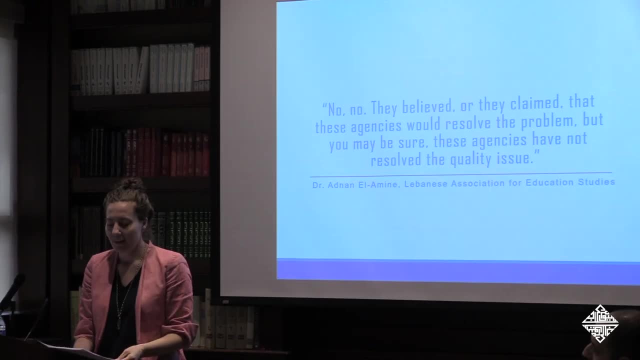 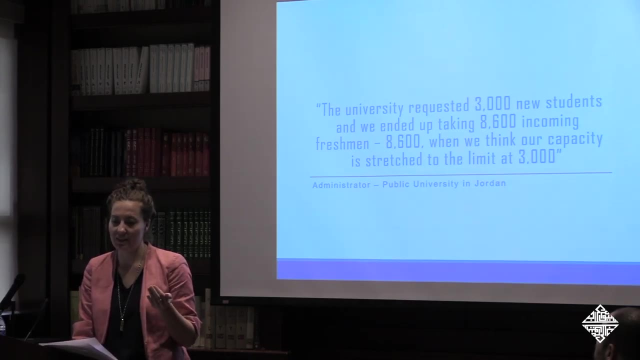 in building up the institution And then, for example, what happens in the middle income countries. I would say in most of those I visited, it's really a pressure for access. That is the major issue. It's one of the major structural constraints. 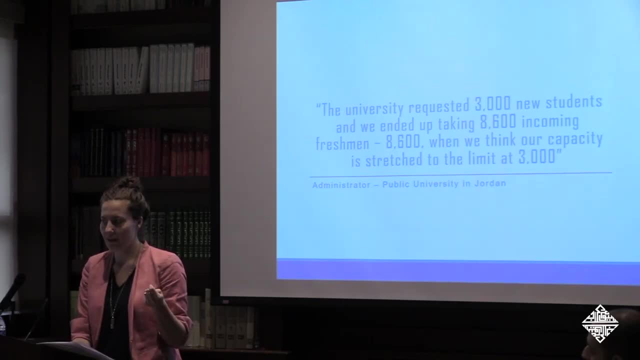 So, for example, when I was in Jordan in 2013,, I was speaking with the vice president of the university And he was saying: the government of Jordan created a unified quality assurance council. that was actually very innovative in a way, because it was going to apply the exact same standards. 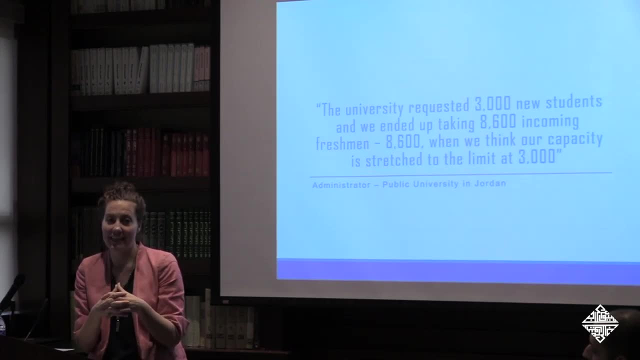 to both the public and the private institutions, which was new and seen as a good practice, But in reality they couldn't uphold those standards in the public system because of these pressures for access, And so, even though you're supposed to have a certain number of student-faculty ratio, 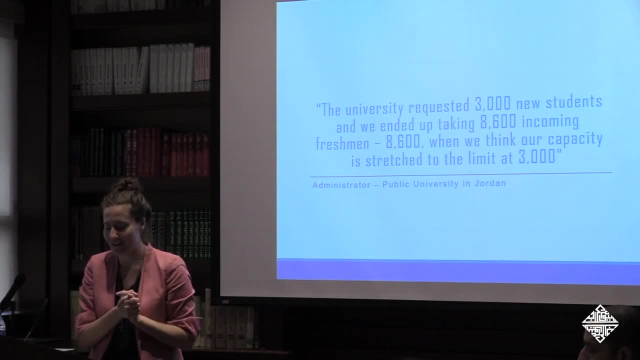 that's often how it's measured, like 30 students per one faculty. he said he was explaining. you tell the government, the unified admissions council, exactly how many students you think that you can take, but they don't respect it. 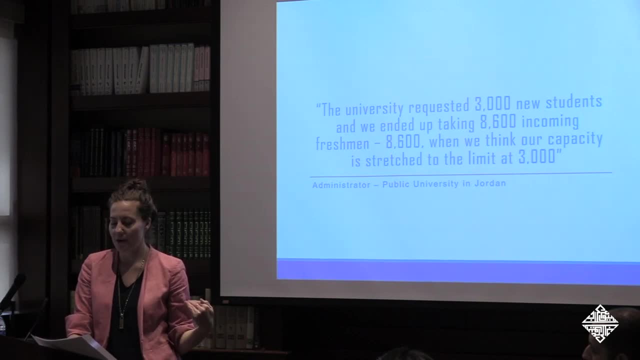 He said, yeah, Yeah, Usually you get double or triple that number. The university requested 3,000 new students and we ended up taking 8,600 incoming freshmen- 8,600, when we think our capacity is already stretched to the limit. 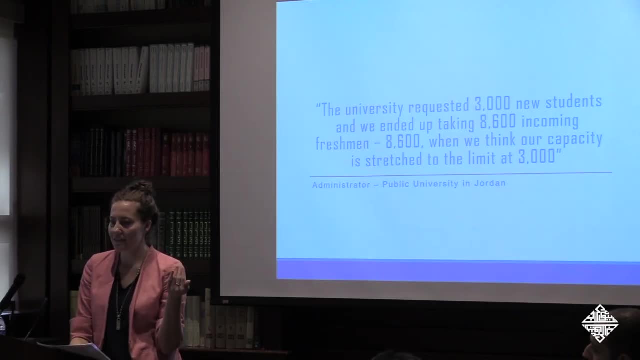 at 3,000.. And that's really I mean. that's why I think these technical solutions are really hard. It's the same government that's upholding the same state in general, that's upholding the quality assurance requirements and the need to meet students' and families' demand for access. 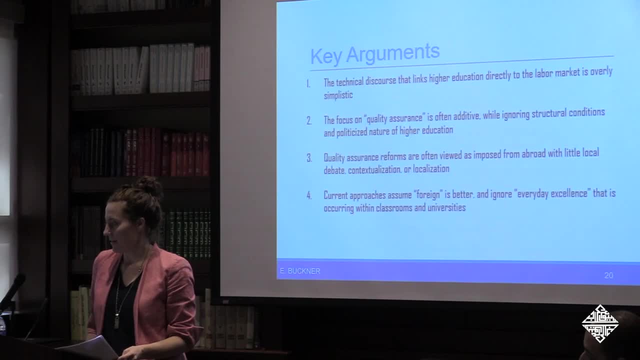 And so broadly. my argument- and I'll just wrap up here- is that these technical reforms that are seeking to assure quality are really missing a number of fundamental points, And the first is that there are, in many cases, technical that are ignoring the broader social and political. 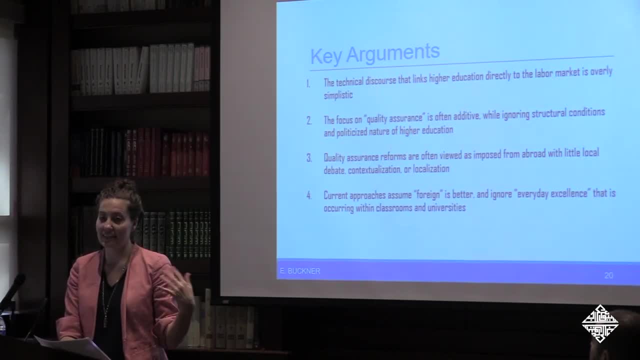 purposes of higher education, as a marker of status and, as in many cases, a position of good. You don't just want to go to university, You want to go to a particular university program, and it's not only for the employment outcomes. 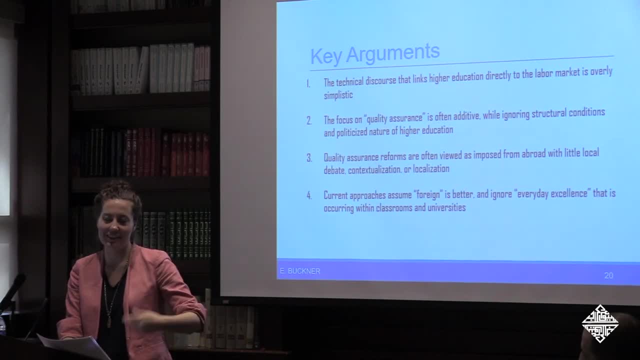 It's also many people that I've talked to want to study one thing, but their parents want them to study something else for a status reason, And so, and then I really, from an educational perspective, the point that I really like to emphasize- 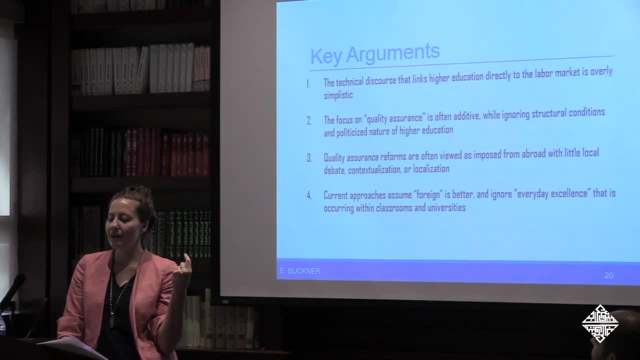 is that when we assume quality, when we think of quality that can be distilled into very measurable and quantifiable indicators, we're overlooking the fact that teaching and learning is relational. Students are learning in relation to one another and their professors, and also with their own sort. 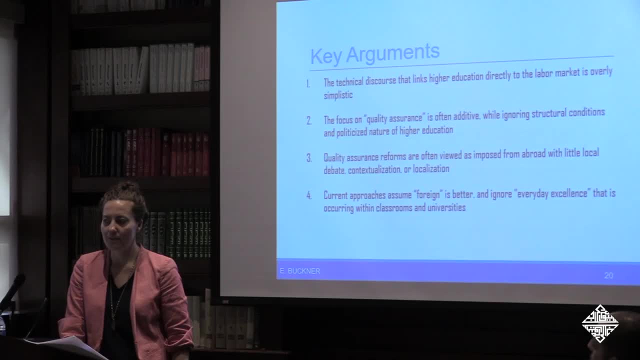 of visions of their own futures, And so we're really missing out on that. these, you know, the class size or the library volumes are not a good measure of the quality of relations, and that we're also not focusing on sort of that. what 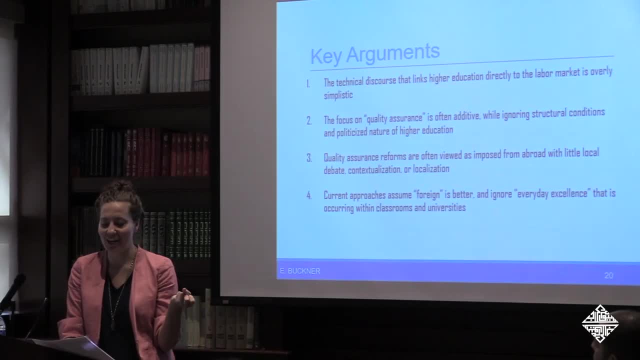 is teaching and learning and what is going on in the classroom Right, And I really argue. I believe strongly that the professors and the students in the region are as intelligent and creative and hardworking as anywhere in the world, And the professors are teaching the best and the brightest. 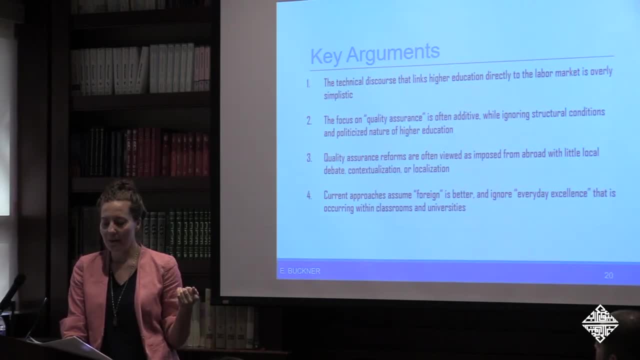 students in their nations And we are the real casualty of the crisis. rhetoric is this form of everyday excellence that's already going on right, Where teachers are working overtime to sort of navigate in really difficult circumstances to teach, and in good ways. 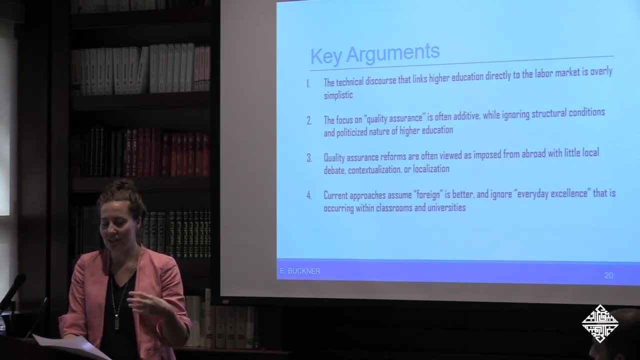 And I. so what I try and do. one of the things I try and do is really like reframe these conversations on higher education that are happening. you know, in think tanks and development agencies and donors that one of the most harmful and pervasive stereotypes 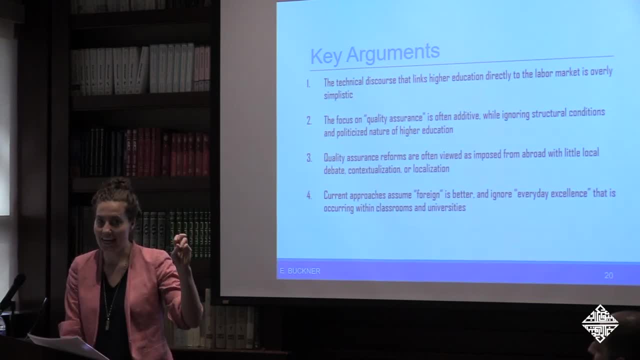 is that the region's higher education systems are sort of lacking, are, like, fundamentally lacking, And there's this sense of inferiority that's perpetuating, Right, It's perpetuated by a deficit orientation which continues to view non-Western societies as 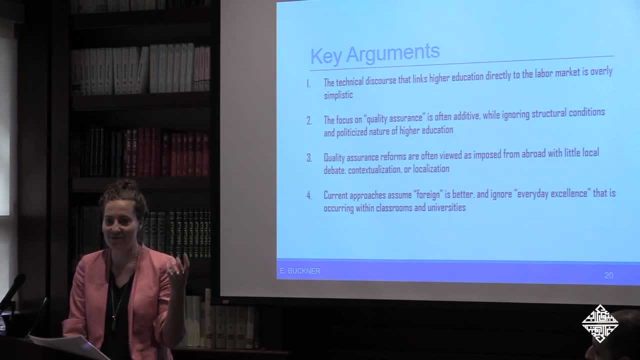 and this is not just in the Arab world, this is everywhere. I mean, this is like sort of higher education. everywhere We view any non-Western society as like lacking in capacity, lacking in knowledge, largely because they have fewer resources. And we continue to reify European and North American. 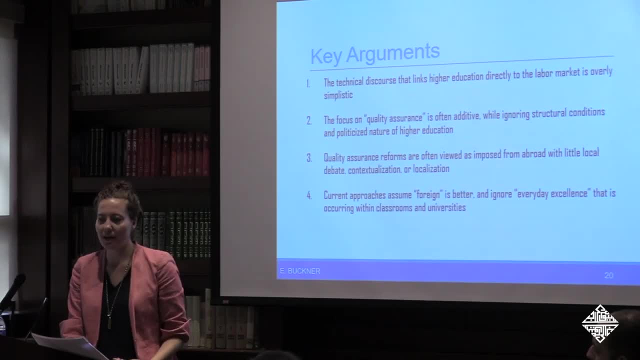 universities as like the models for reform, And so I argue that we need to really rethink these conversations. We need to, you know, start from the premise that there's a long history of indigenous scholarship and intellectual tradition that continues, and that universities have always played really. 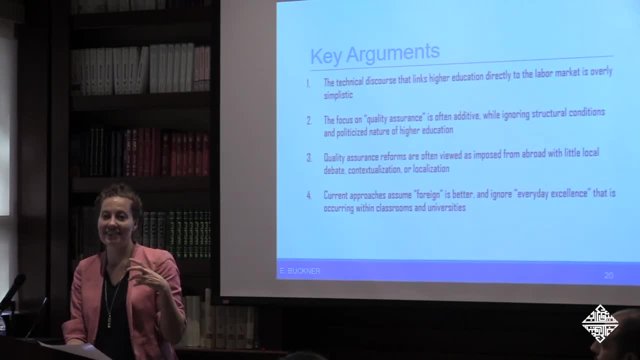 important roles, not just in labor market preparation but in building societies, And there are critical sites for citizenship development and protest. that is ongoing today. So I won't stop with that, But I will say: like, how would conversations about higher education reform and the Arab world? 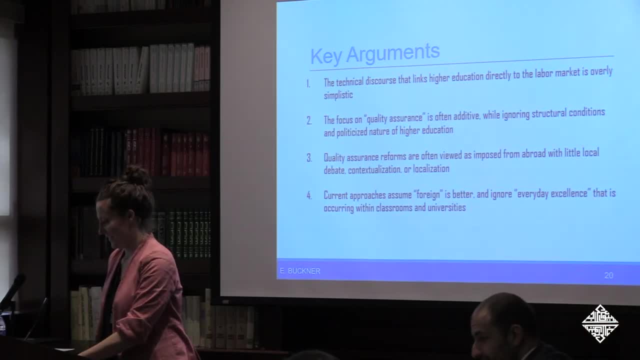 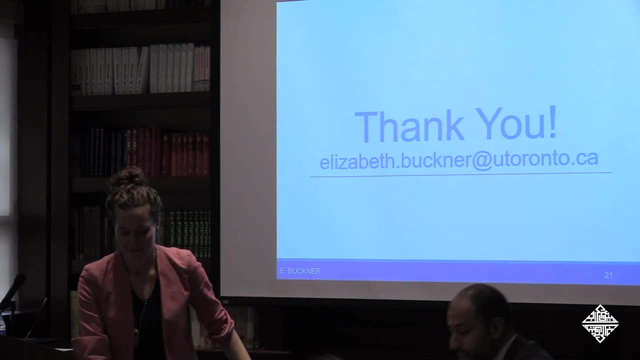 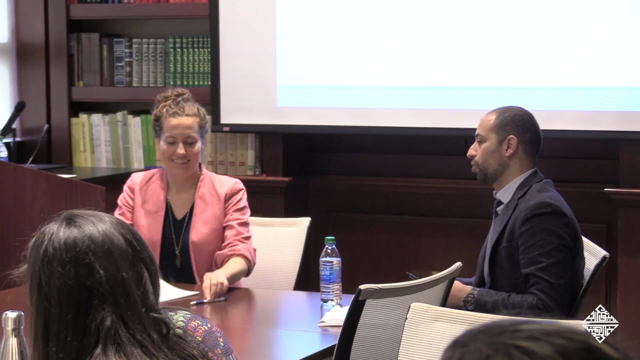 change if that's where we started, Thank you. Thank you so much. So we have some time for questions discussion. I thought maybe I'd ask the first question about sort of the. a lot of the problems you identified here are very much related to kind of state reform. 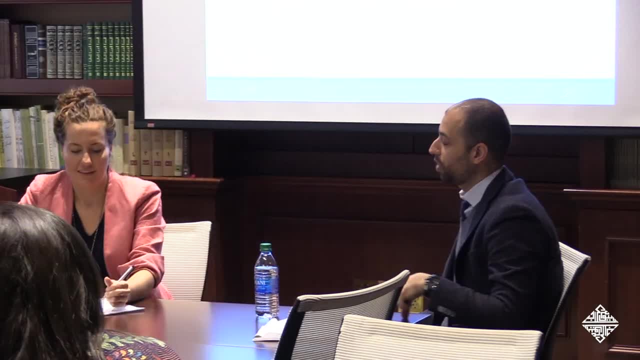 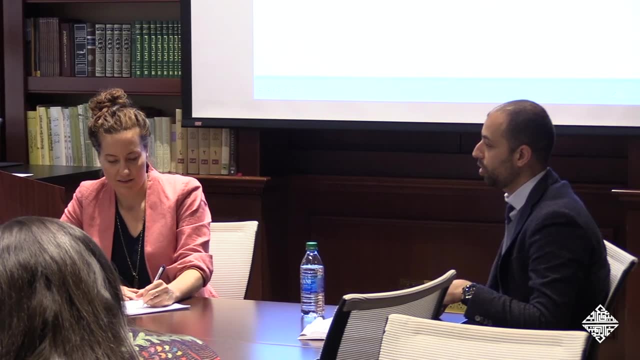 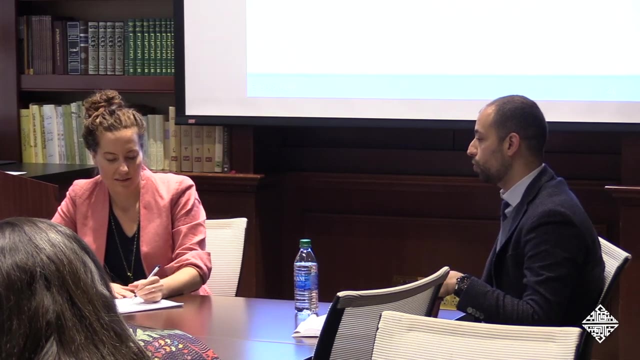 state-led reforms. So how does privatization change And kind of play into whether it's actually addressing any of those questions or issues in a more efficient way or kind of dealing with problems that may be more beyond the purview of the state, specifically because there's a lot of kind? 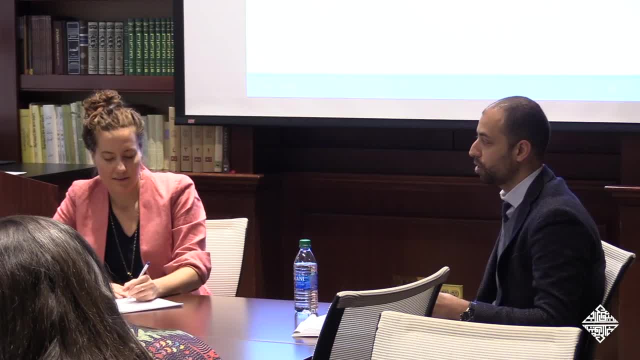 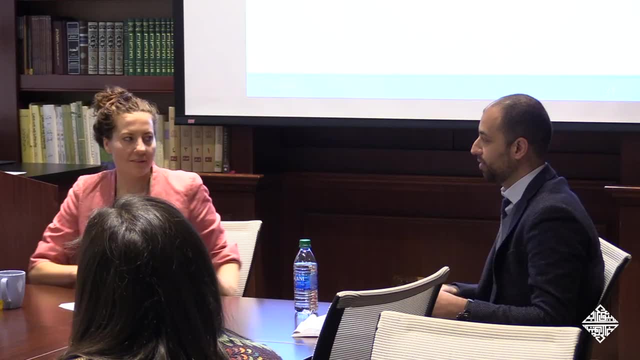 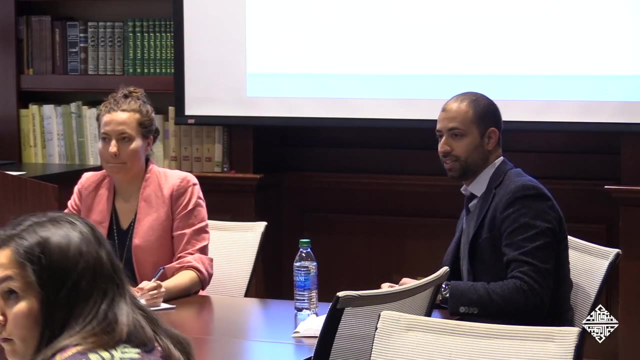 of underlying political objectives that the state is trying to accomplish, that maybe privatization may or may not be thinking along the same terms. Should I take that? Sure, Why don't we go around and maybe take a few more questions? Yeah, Yes. 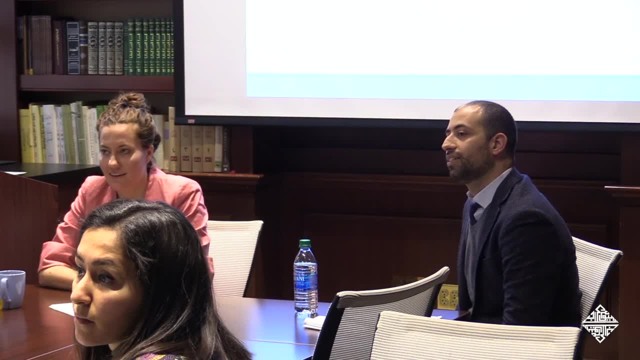 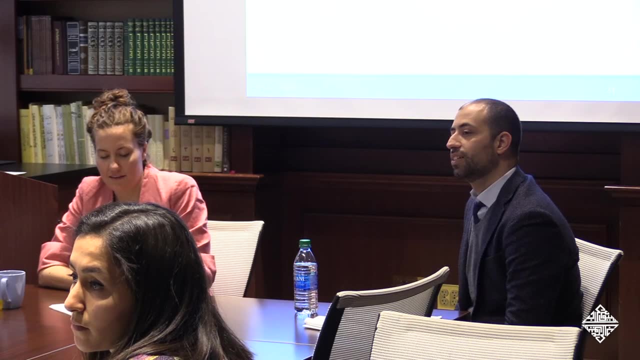 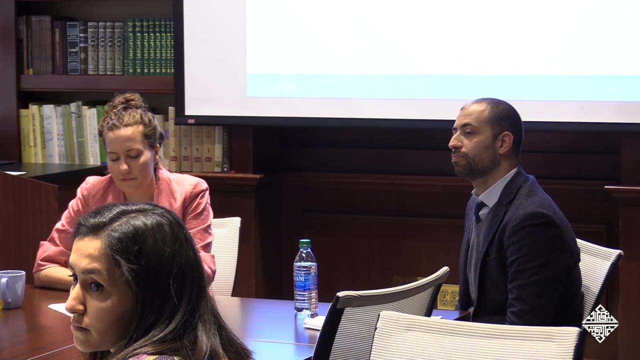 Have you done any research about what Arab students look, how they look at Western universities, Because a lot of Arab students like myself have left their countries to seek education here, for example, because we've found problems within our own systems or because it has to do a lot with social mobility. 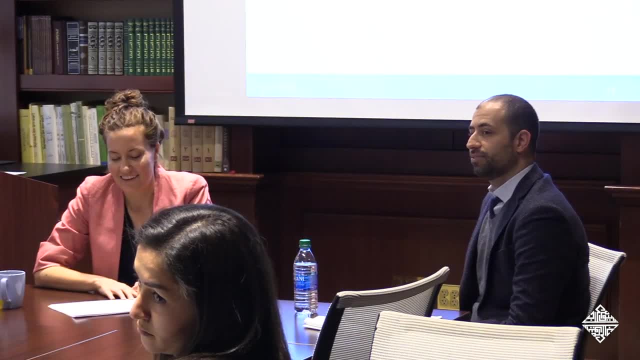 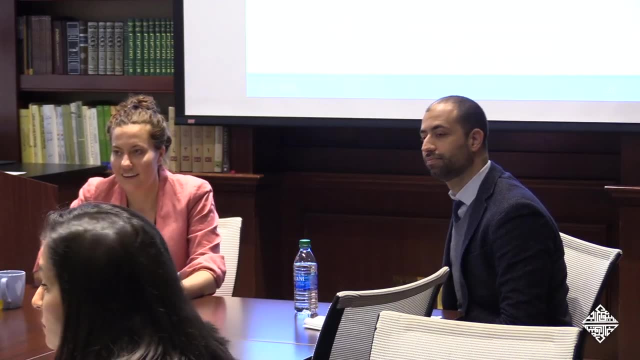 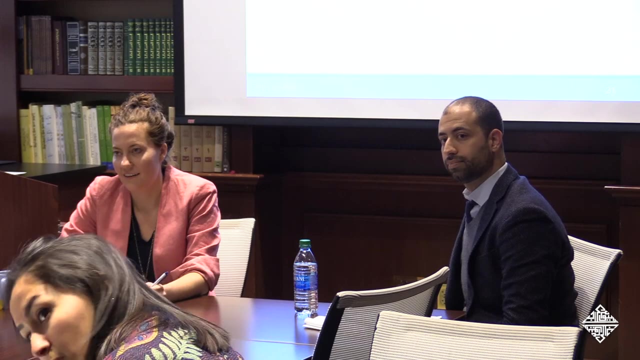 If you could talk more about the other way around. Yeah, Yeah, I don't know if this has been an overview and a sort of generalized view of the region, if you're preparing to look at individual countries, But if you are, I'm just wondering. 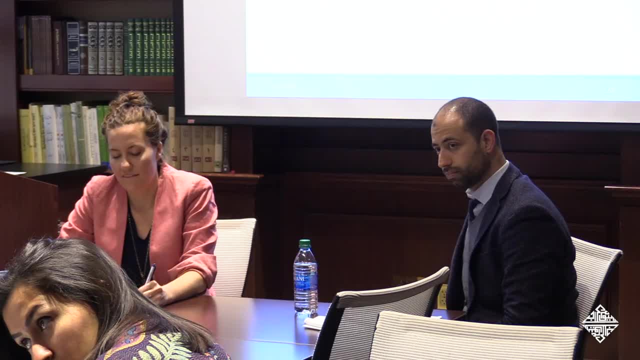 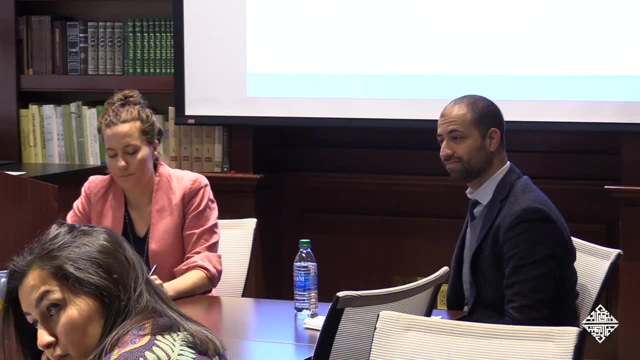 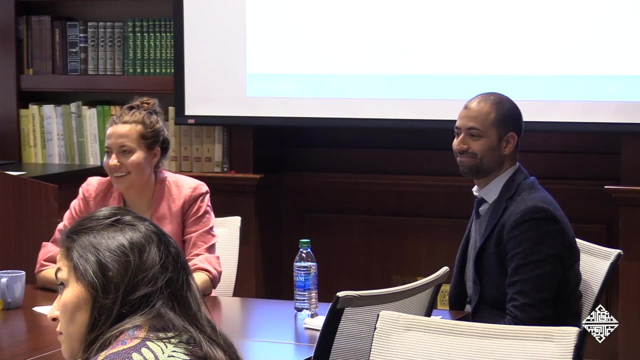 with regard to Palestine. how do you see that as exceptional and how do you see that as within this whole group of your analysis? Mm-hmm, And we'll do one more for this round. Also, thank you for your presentation, Since you've worked in the Gulf states. 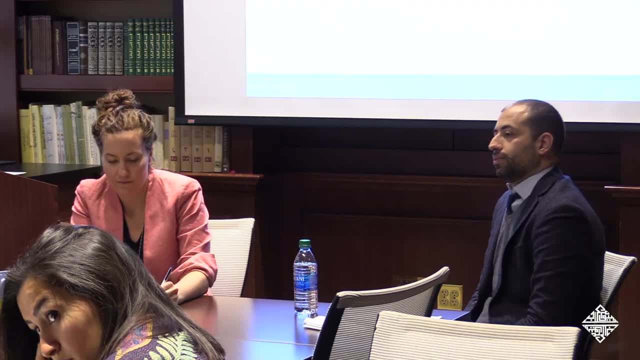 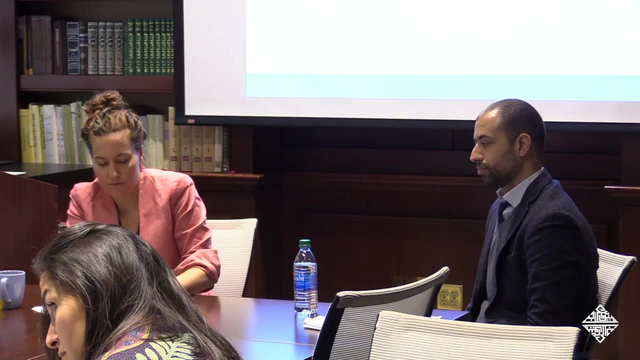 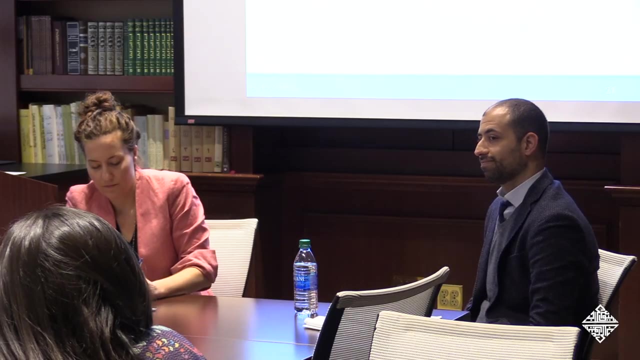 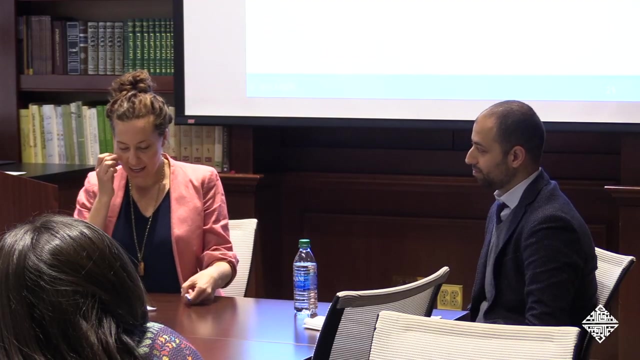 did you also look at teachers and pedagogy in terms of are they being prepared to work in these Western models Since internationalization is happening? how are local professors dealing with that? Yeah, Yeah, Yeah, OK, Great questions. Thank you all. 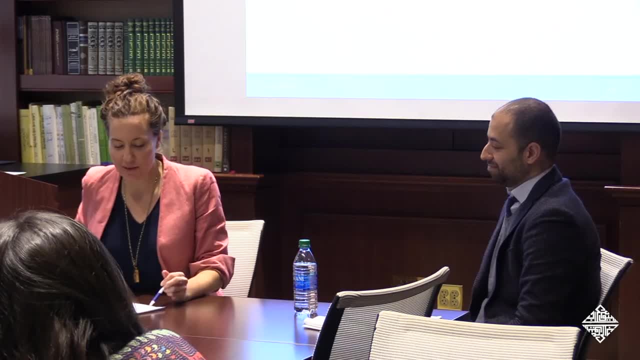 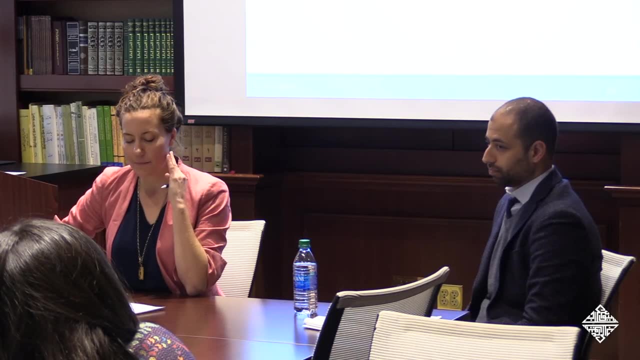 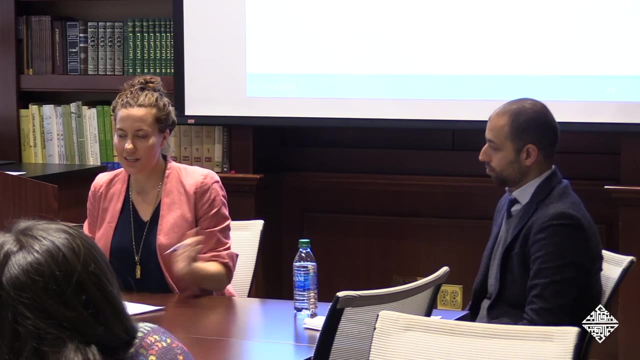 Well, OK, Very different ones. I guess I'll start with the individual. So I don't look at Palestine in, I just, but in my thinking I, yeah, I don't. I mean, there's a bunch of countries I obviously don't look at. 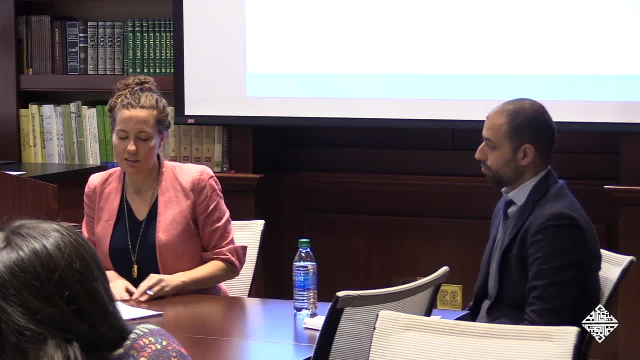 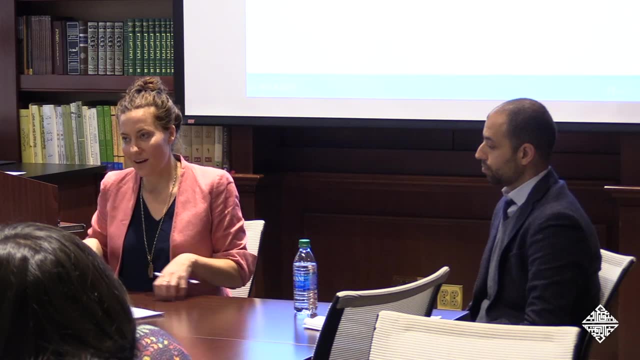 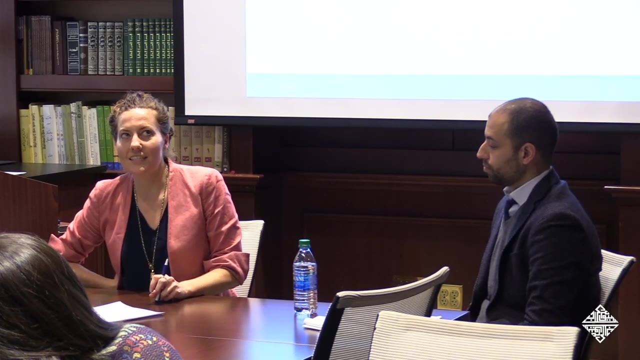 I don't really look at any of the countries that are currently like in conflict settings, Honestly, And that's I mean there's so much more complicated even than what I am doing. But also I do think that to the extent that 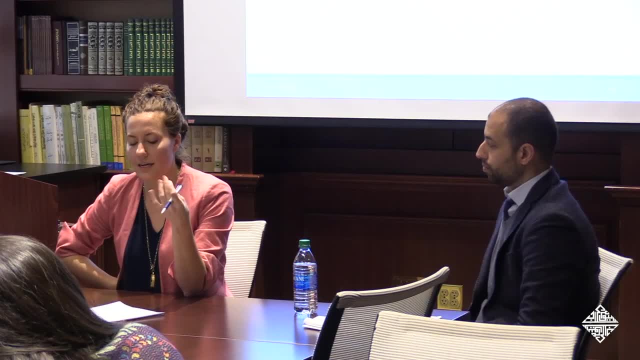 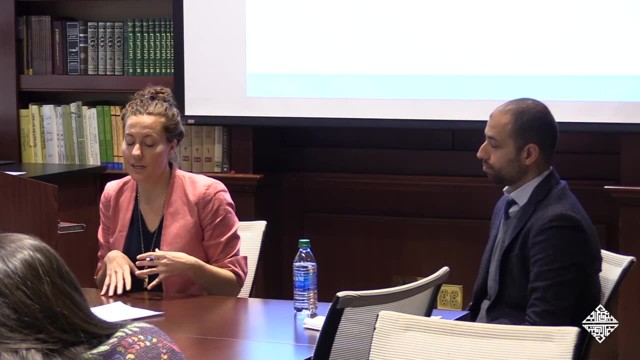 I think that one of the arguments I do think about is that in countries that have been more fragmented, either because of conflict or other, or like the state has generally been weaker, they do tend to have more privatization, And that's not just in the Arab world. that sort of 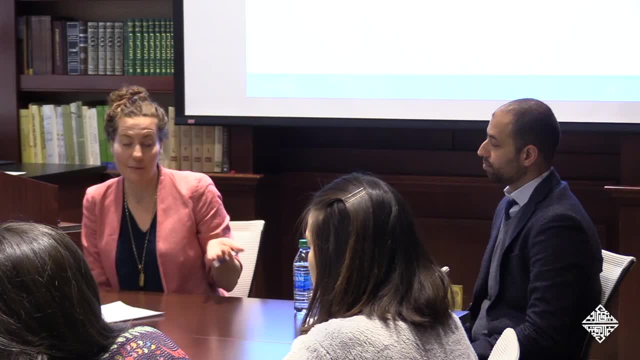 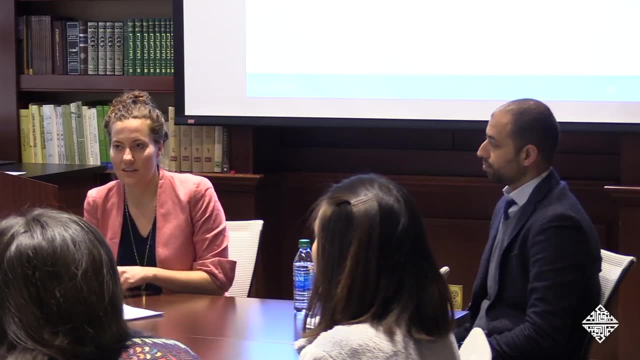 we see that in many places, And so that's the case in Lebanon, you know, where there's really only one public university And then and so in Palestine, there, you know, the universities are all considered private universities in some ways. 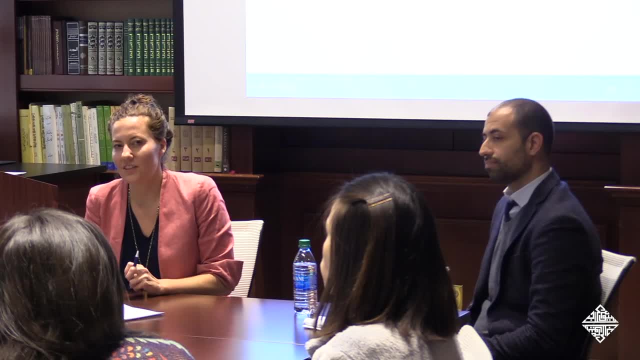 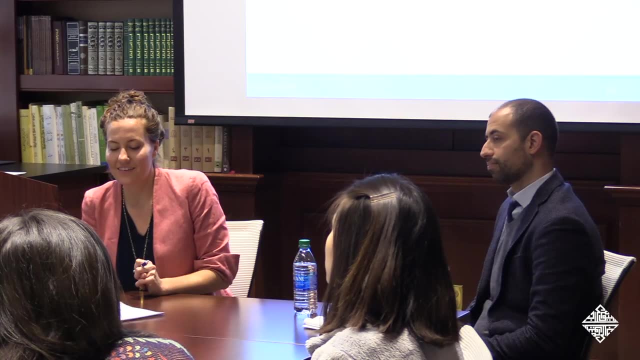 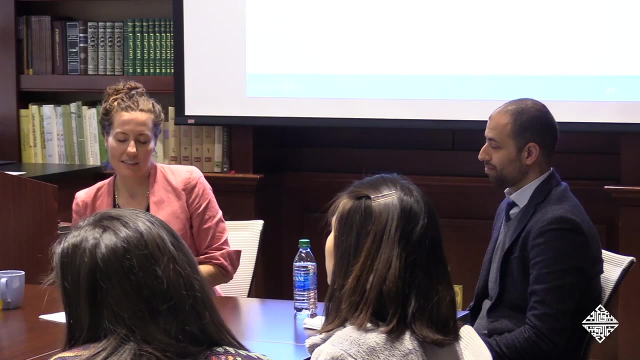 OK, So no, I just don't look at them, But I so, in terms of privatization, I think I, I think it's a really interesting question. Like I study private higher education as a phenomenon that's growing everywhere. in many cases, 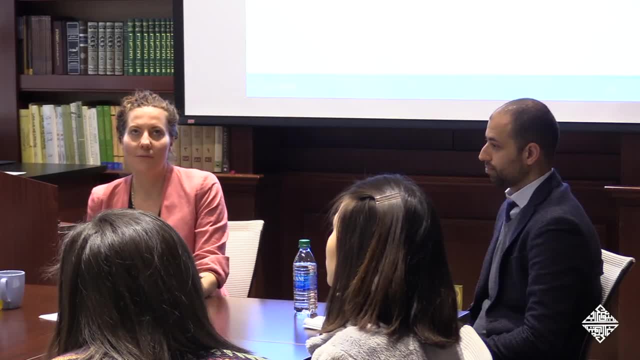 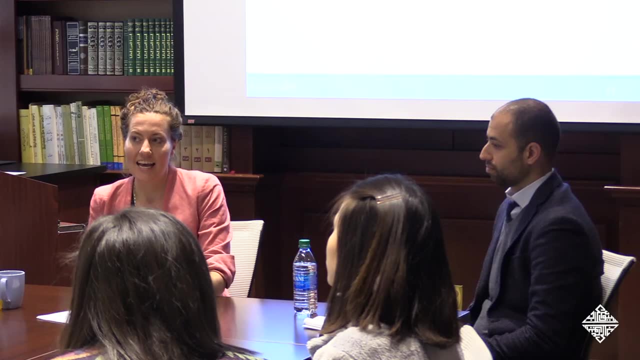 And it is I, but from like a non-ideological stance, like there are advantages to the private universities in many cases- And there are, but they also have they're very contentious, Like I think that's the main point that I really try. 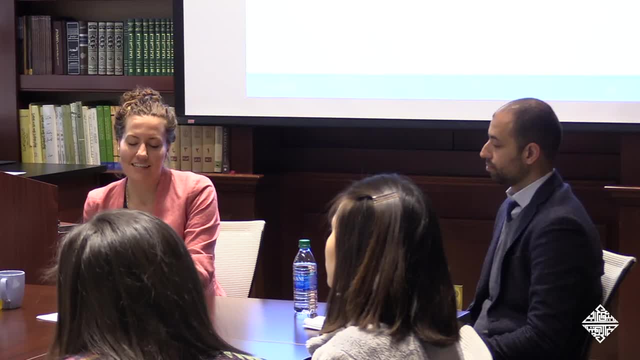 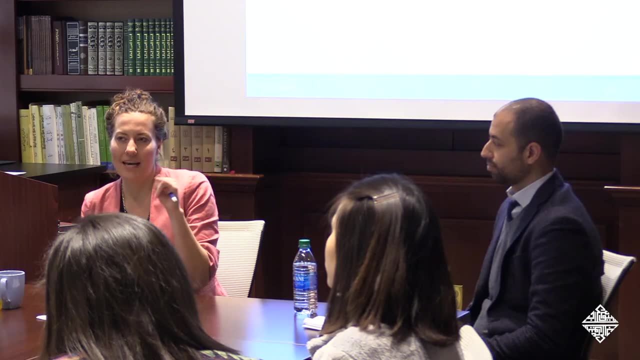 and think about is that the, the private higher ed, is seen as an apolitical solution To all of the problems with the bureaucracy and the. you know, mismanagement or the way in which the public universities like who's on the board is very political. 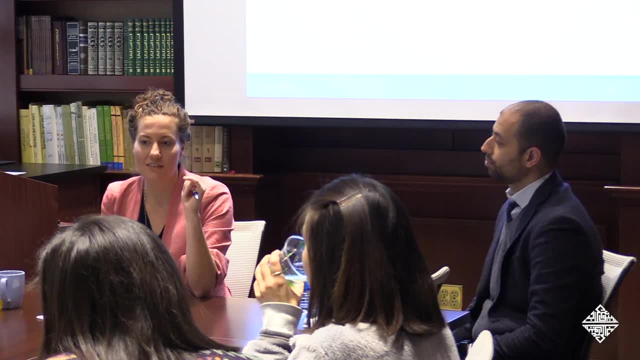 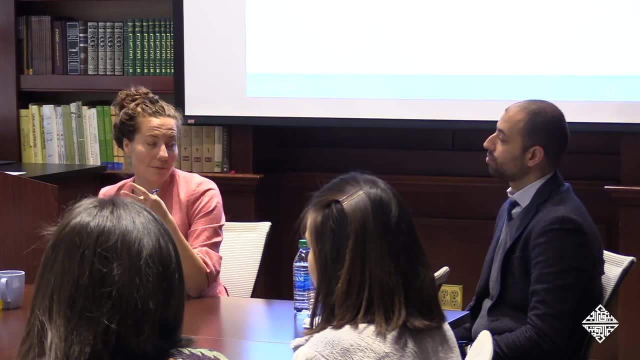 and these other sort of the, the political dynamics are seen as very messy And so private higher ed is sort of used as a way of solving these problems. It's like more efficient and like outside I mean. in fact I would argue that the 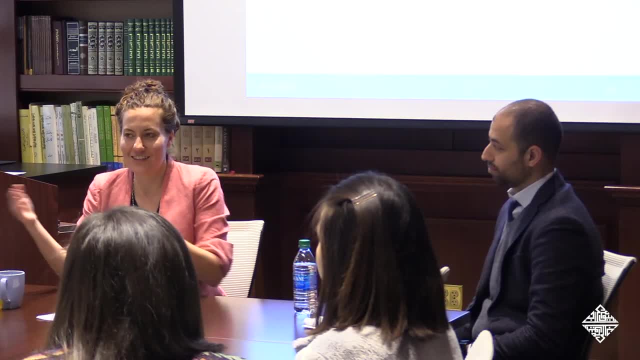 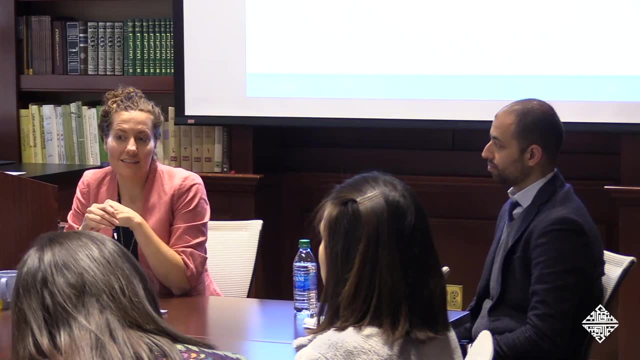 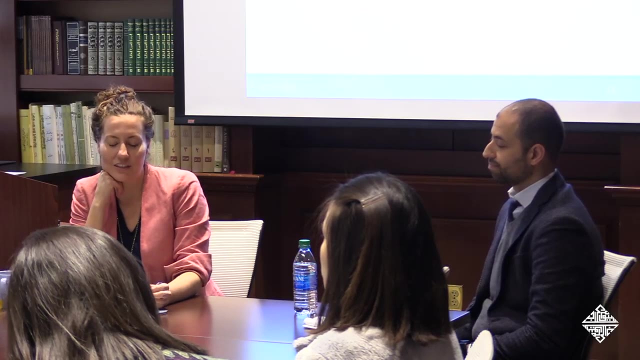 where private, who gets the contract to open a new private university and how they get all run in and what the policies are governing, whether they can be for profit or not. all of that is actually very political and implicated in sort of the state processes. 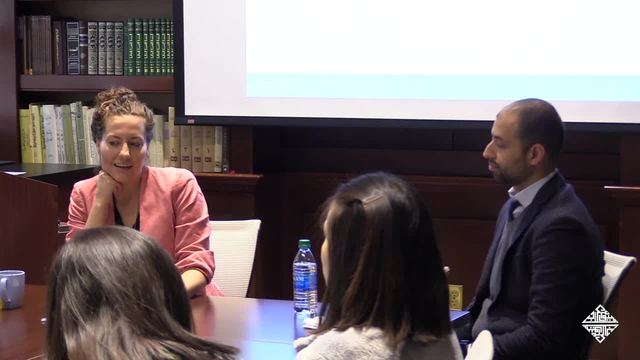 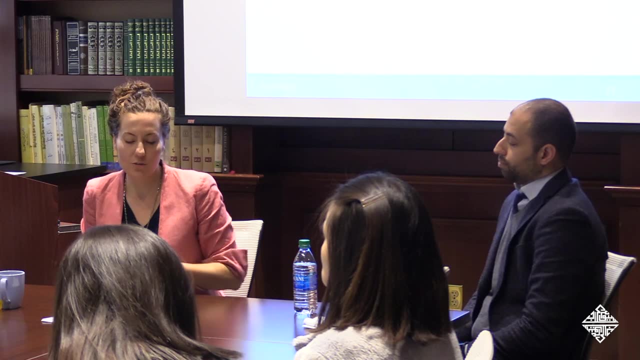 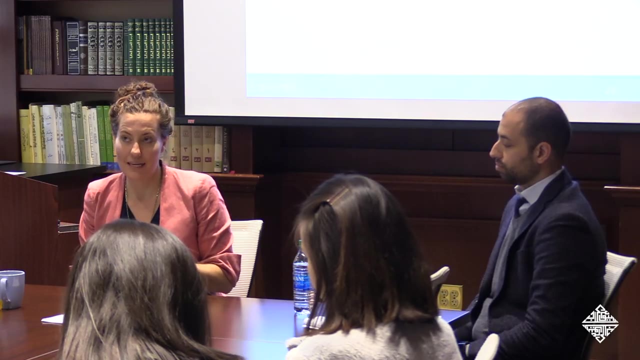 But I think, if you look at who but the, what we know for sure is that private universities do tend to be tuition. they tend to be much more expensive than the public universities. That's without a doubt, And tuition dependent, often for profit. 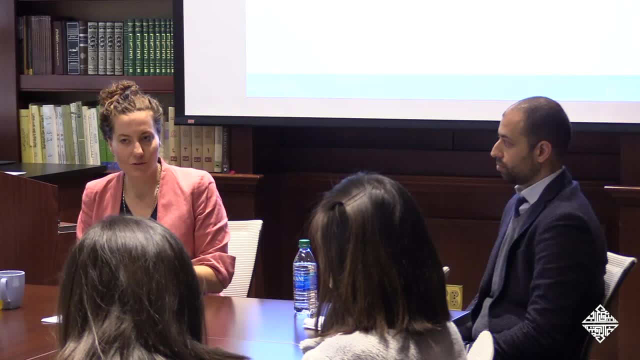 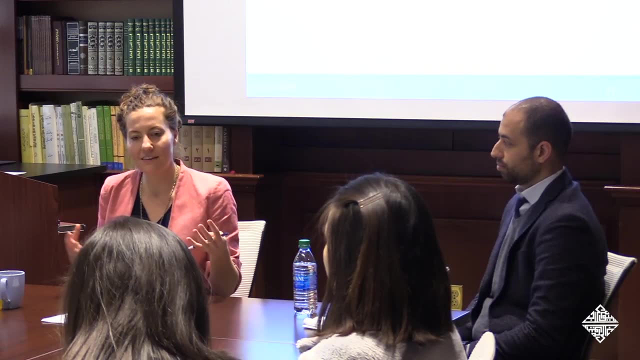 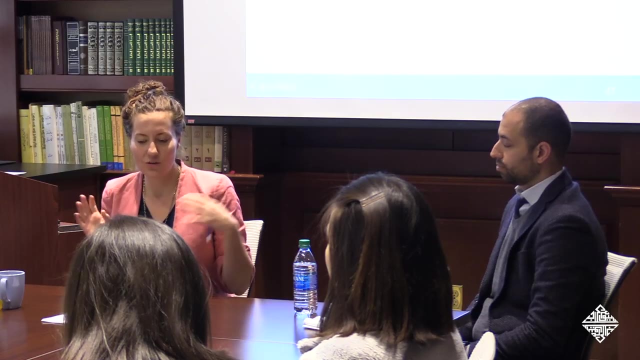 And so it's actually like you know. lots of entrepreneurs are pushing for more private universities because they can actually make money off of them and that they've thrived in countries where different groups are not well served. So Jordan has many and growing private universities. 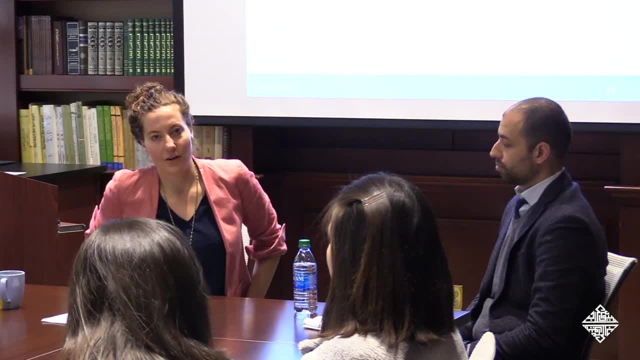 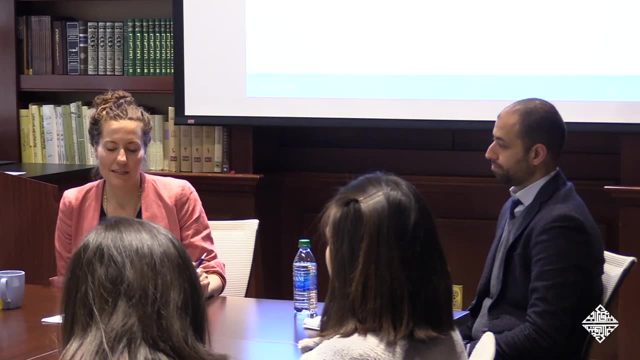 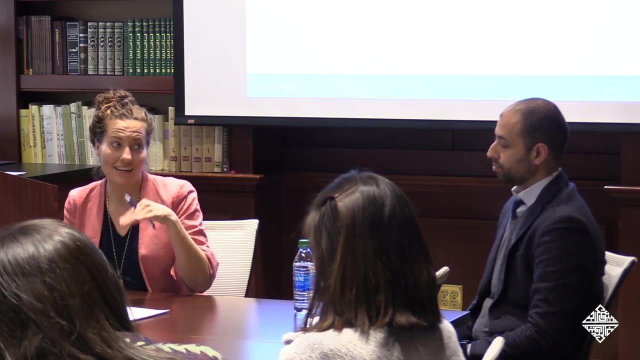 that are serving the Palestinians who aren't, you know, don't have as equal access in the public universities And then, but in many of the sort of North African countries where free access to public higher education has been sort of embedded in constitutions, 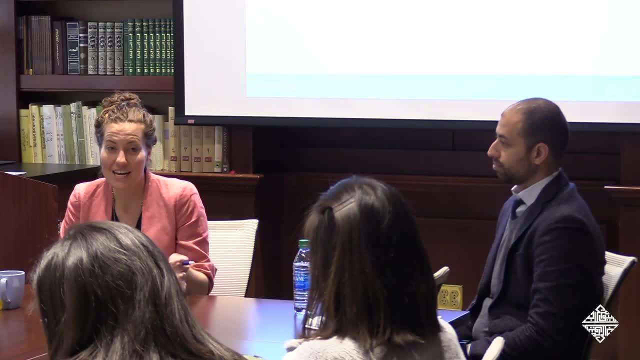 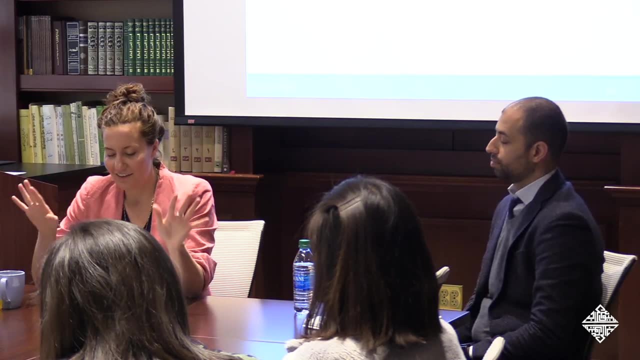 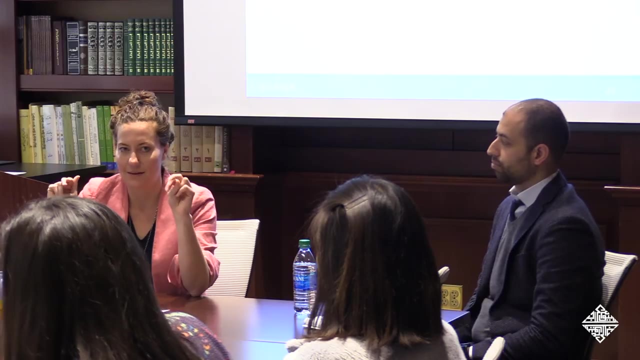 it's been much more controversial. Like it is growing, it does exist, But for example, when I was in, like Tunisia has had, like has been not, did not want you know, sees private universities as sort of the second class or the lower universities. 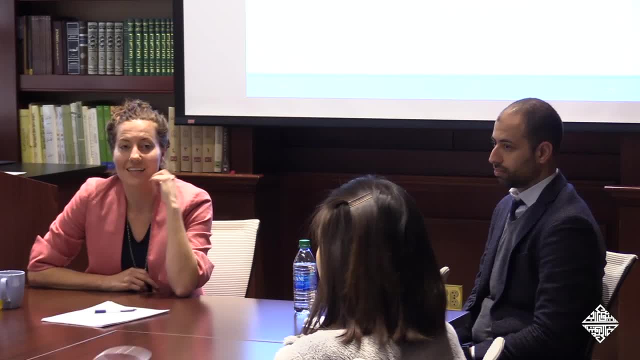 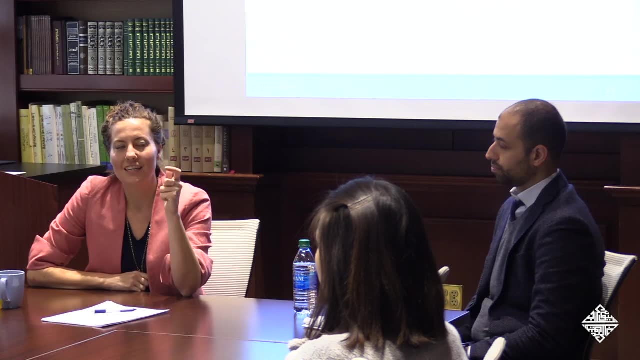 And so the people going to those are actually in many cases like Sub-Saharan Africans who are coming to Tunisia to study in French And then so people really see them as like the second class education, And so that's where they're growing versus like. 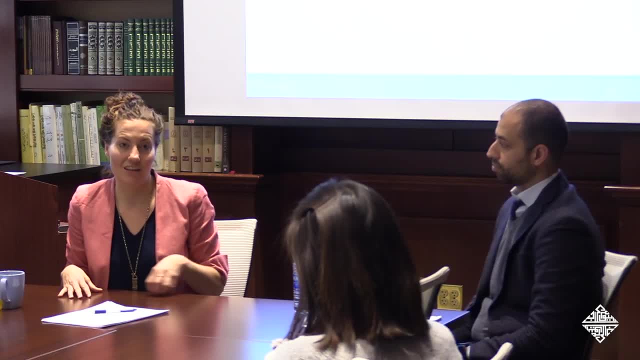 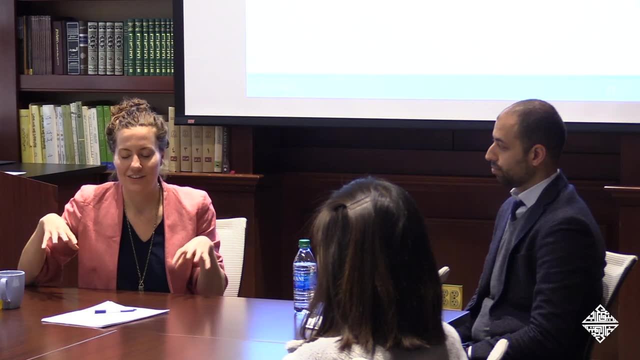 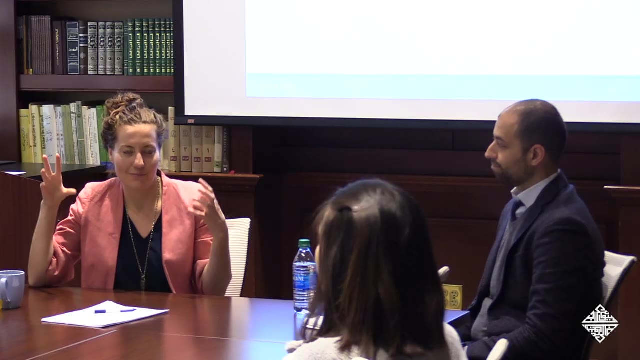 and in the Gulf there are many, many private universities that are serving the non-citizen resident populations. So I think in, I think in the big picture, that's where they're really growing is in the places where there has, where the state has a harder time, sort of pushing back. 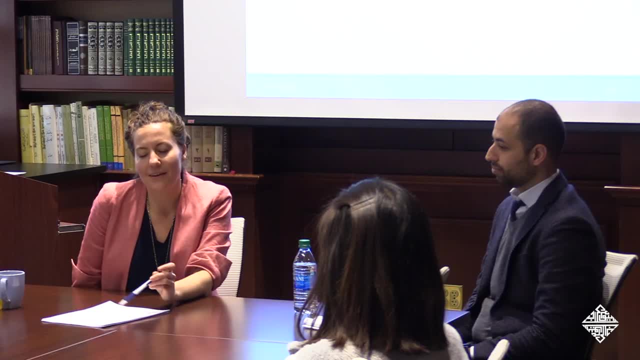 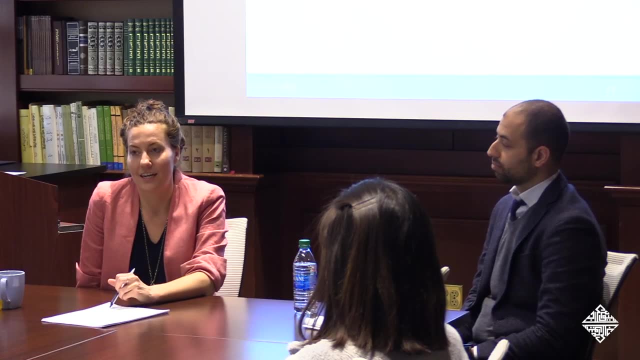 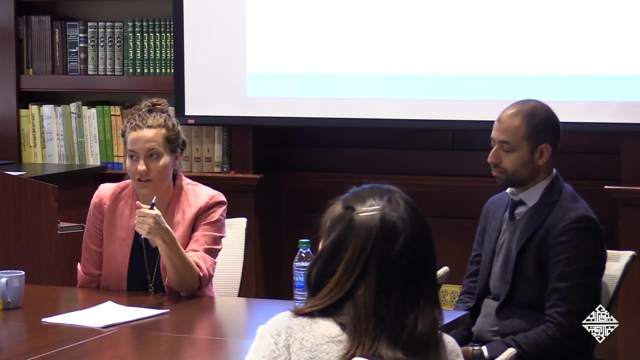 So but yeah, I think it. and the other point I would say is, like many of them thrive by offering programs in English that were like having programs that are accredited, that by international associations, that sort of then legitimate, legitimize the degree or offer sort of options. 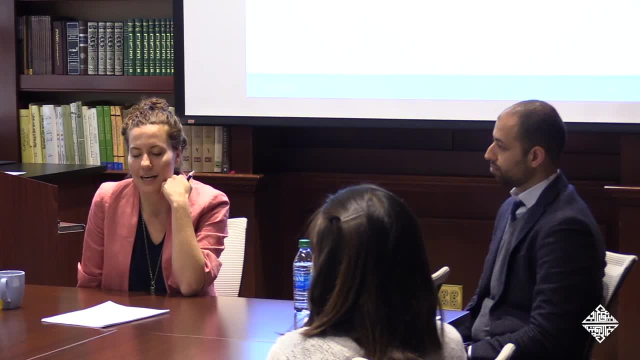 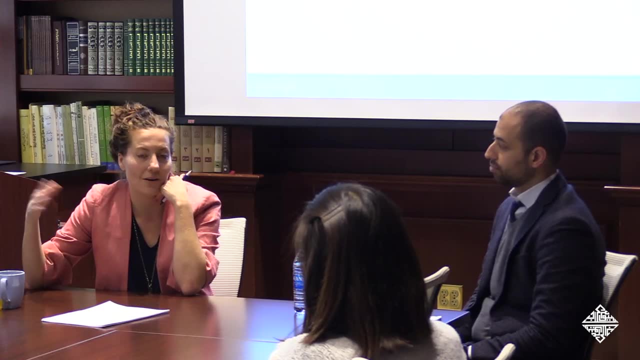 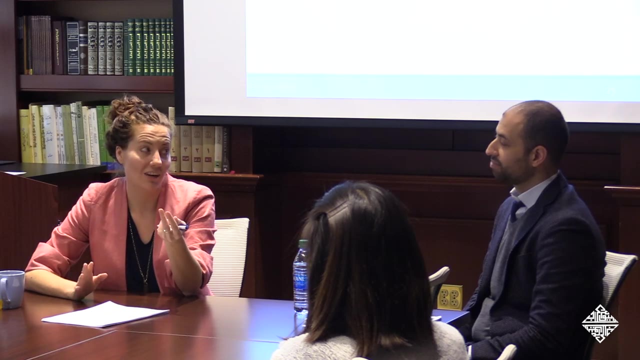 for late, subsequent employment elsewhere, And I know that's not so. in some ways I think they are also growing to serve the ambitions of upper middle class families that want sort of opportunity and mobility or a degree in English, And so that's also sort of where they're thriving. 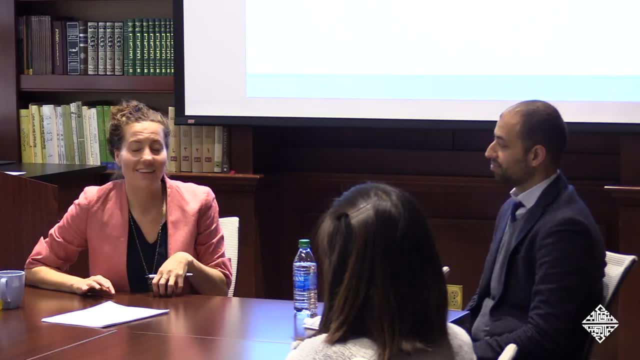 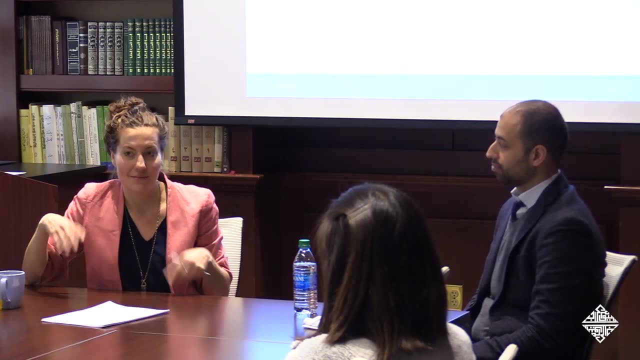 And the problem. there's nothing wrong with that, other than, like with everything, I think, when we, when that leads to a lack of investment in the public system, that's when it's a problem. It's about when, and you know. 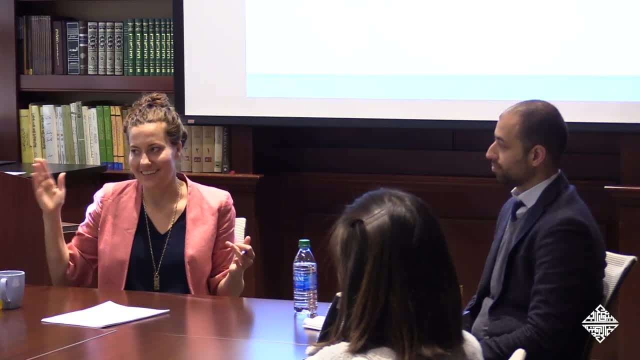 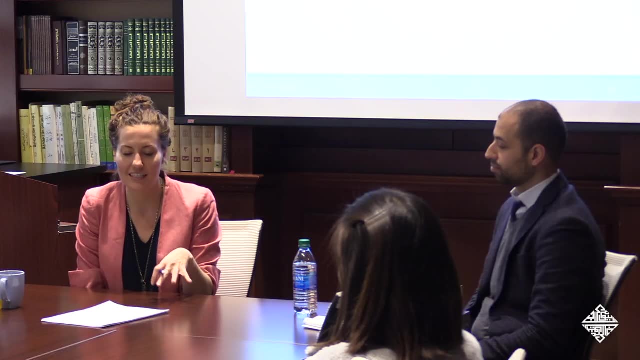 that's something that US faces as well, as the private tuition is growing rapidly and states are less and less likely to sort of support their public state universities, And so this is sort of one of the things I argue is that we actually can learn, you know. 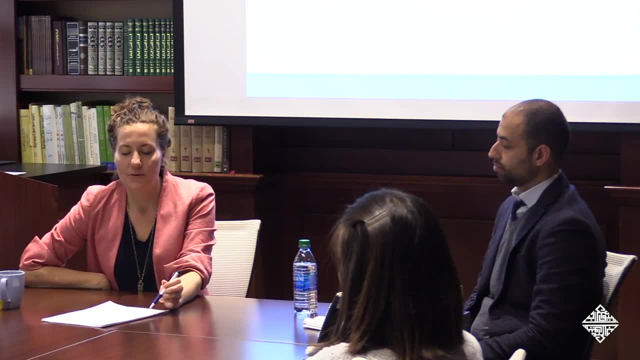 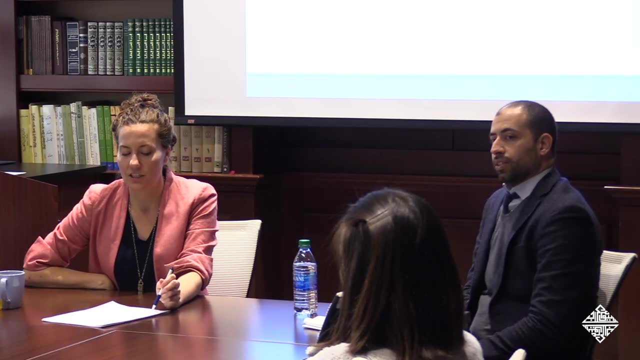 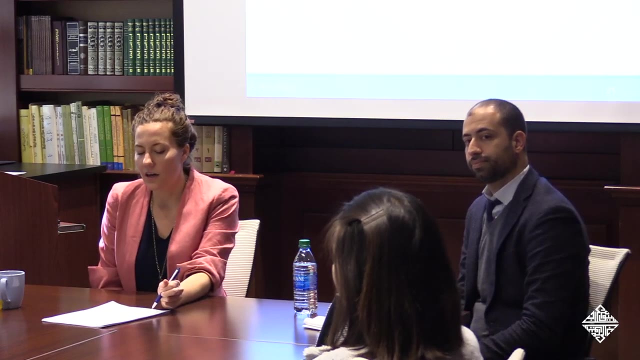 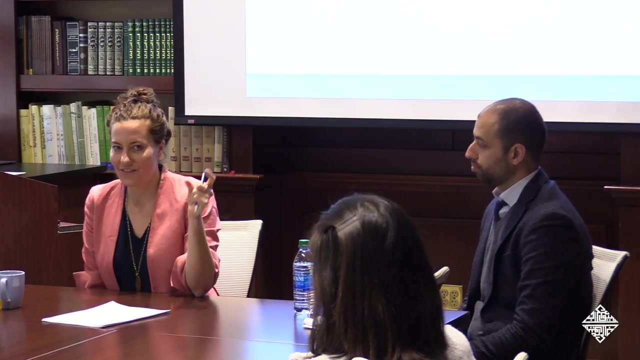 we can learn a lot from each other. So then, okay, yes, I definitely have talked to students and and I actually think that the- I mean I think that I understand that universities, especially elite universities of the world, are really special places in many cases. 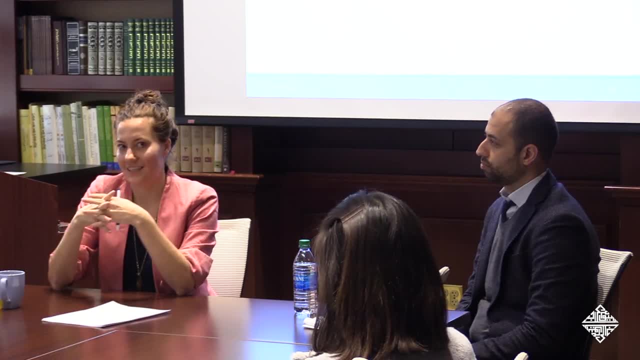 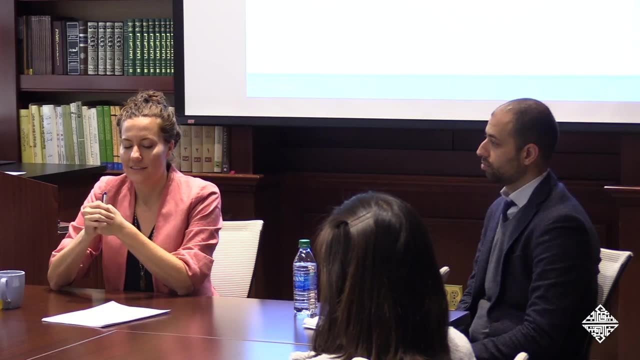 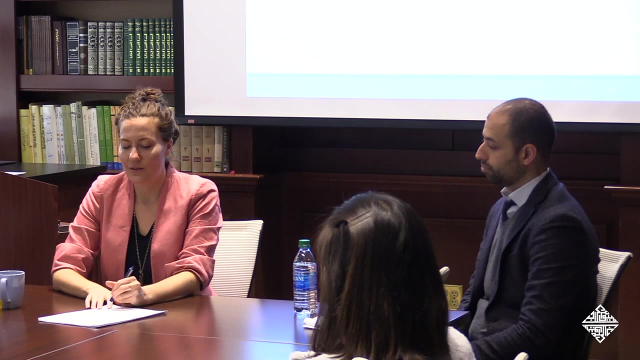 You know we really have tremendous resources on a campus like Georgetown and that they are held up as very elite and like and do promise really good quality and you get really excellent quality at many of these universities. And so it's not. it's not. 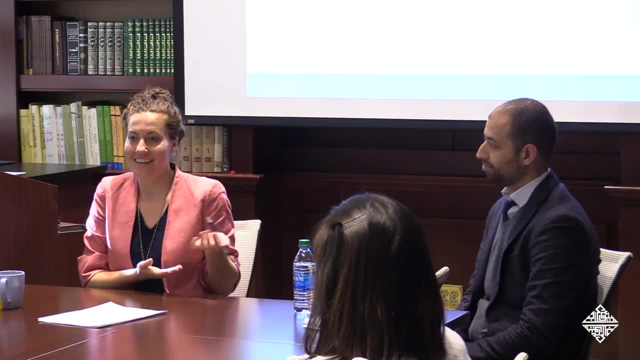 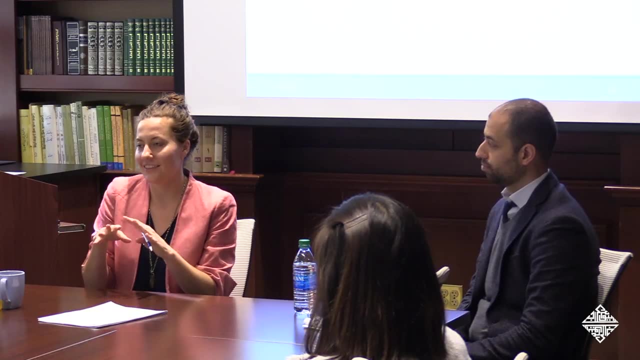 you know, unexpected. Like I work in Canada now and even like the elite Canadians look to the US system, even though Canada has great universities, you know the most elite also look to like the Ivy League institutions as well, And so it's like not surprising. 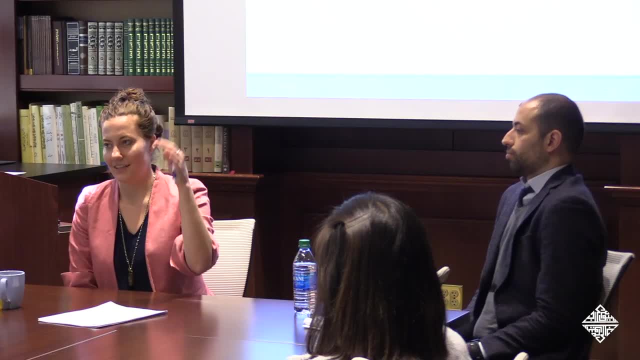 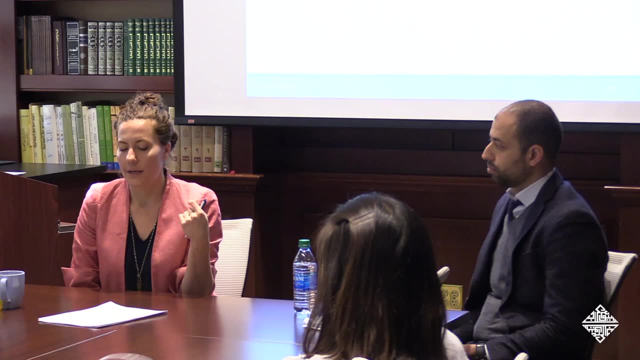 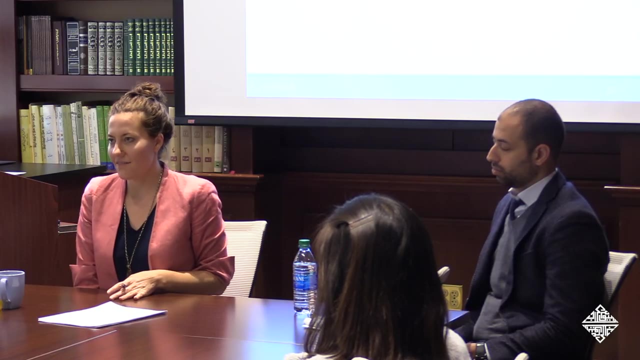 that sort of elites all around the world look to these sort of particular models to as sources of opportunity, And I am very sympathetic to the fact that you know young people want opportunity. In fact I actually that's the way I think of internationalization generally. 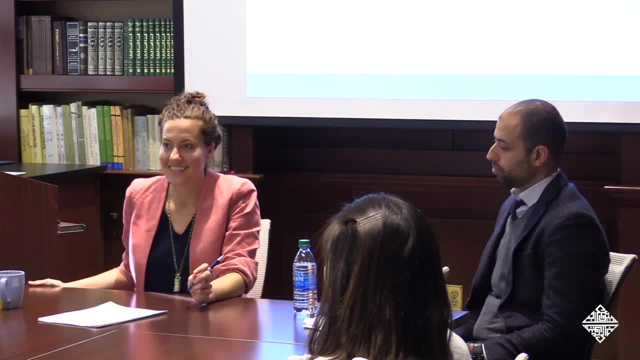 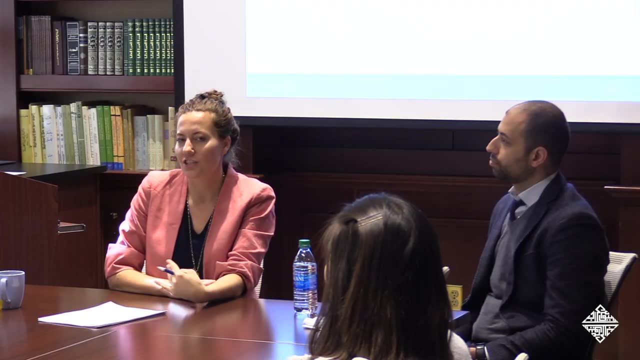 is that it is seen as a very good thing, and it is seen when it promises sort of opportunity. When you think of it like that, like a lot of internationalization efforts, like scholarships abroad or you know a degree in English that will then open up a pathway to. 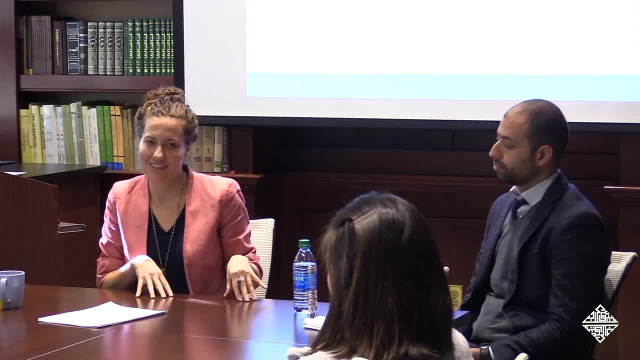 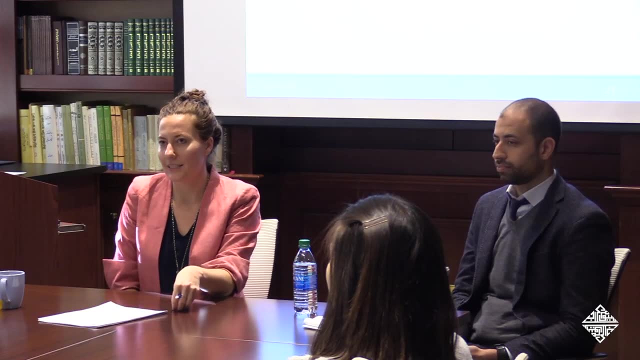 like the German Jordanian University. you know you do two years in outside Oman and then you get a pathway to go to Germany and study and get your degree there. There's, like lots of these pathway programs, that sort of promise, future opportunity that are very desirable. 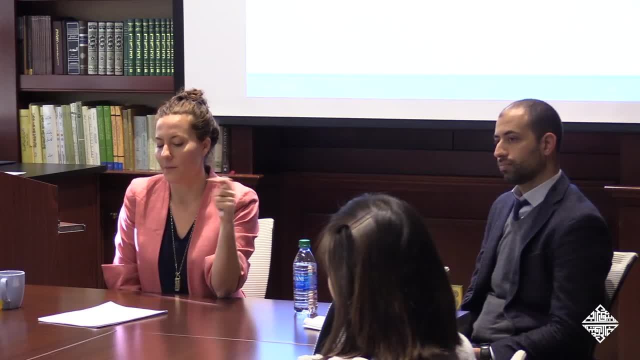 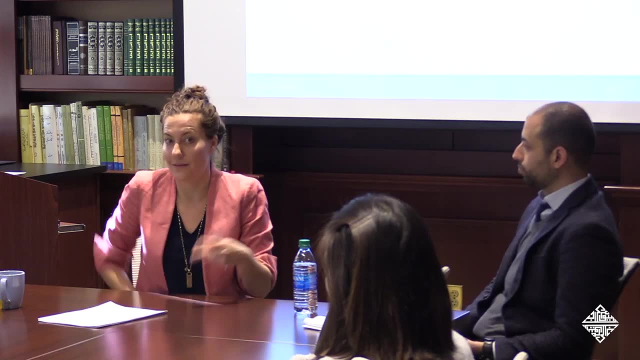 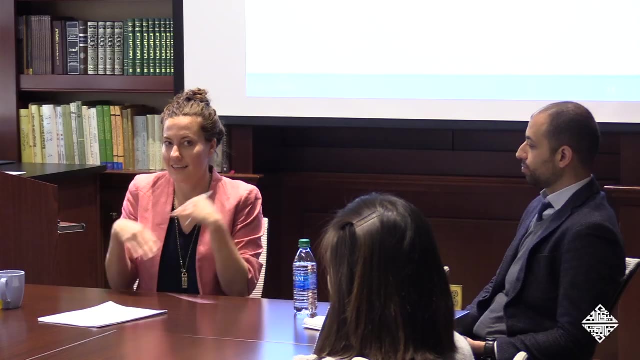 And that when they were just framed as like opportunity, especially opportunity that upper middle class or upper class families are really in the best position to reap the benefits of, because they're already, you know, they received the best sort of secondary education and they have access to that like linguistic. 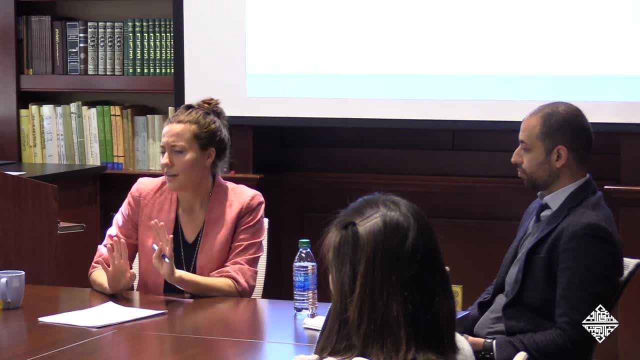 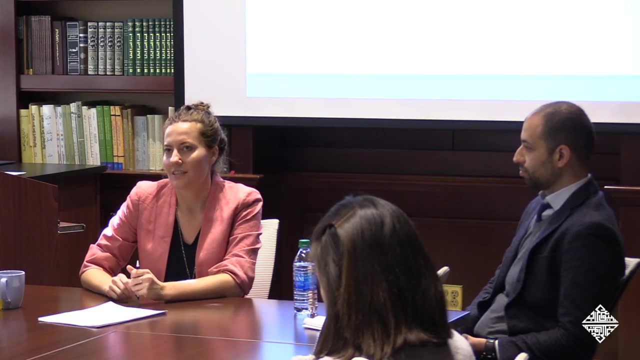 and cultural capital to take advantage, then they're really not contested in many ways. Like people like them and they want them and they want to take advantage of them. It's the when internationalization is most contested is when it's seen as sort of in. 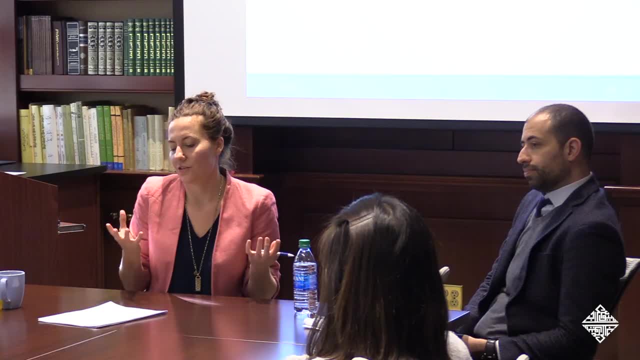 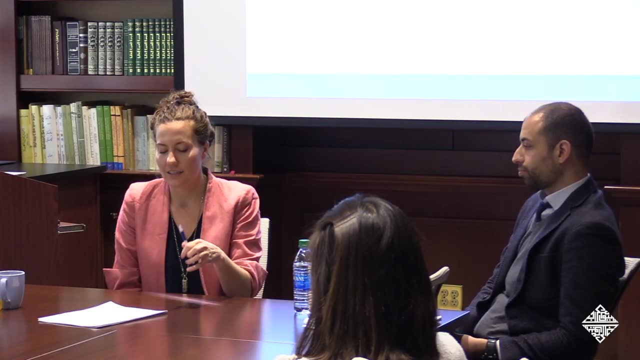 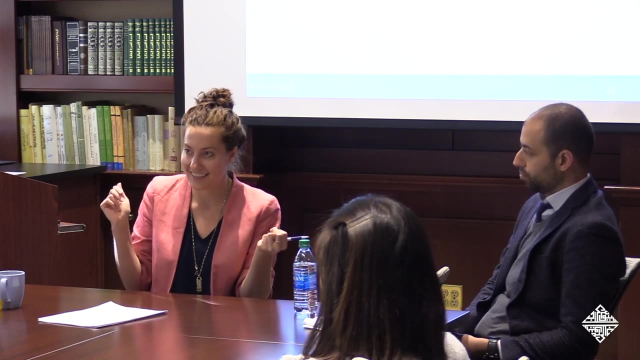 as sort of undermining the role, the national role of the university. And I do think, like with everything, the when there's an under investment in the national institutions and the public institutions and you can just like exit the system, then we 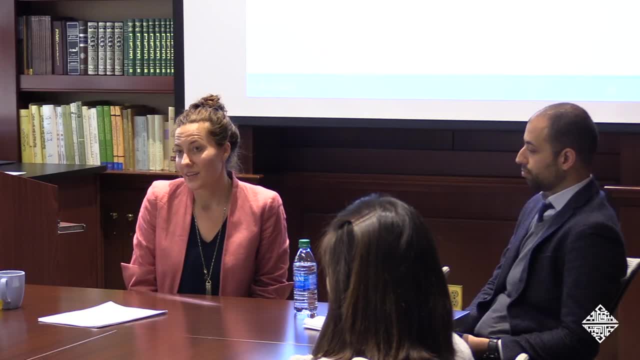 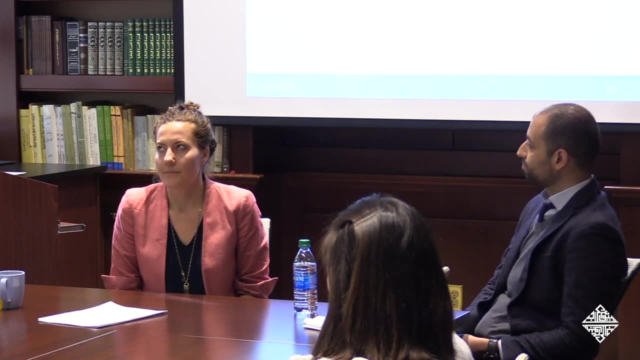 there's less, you know, there's less focus and investment in improving the system, And so I- yeah, I definitely that's how I would say. I mean I also, yeah, definitely- talk to lots of students who I mean. 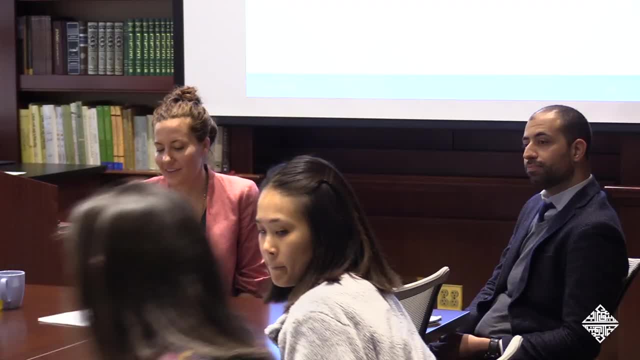 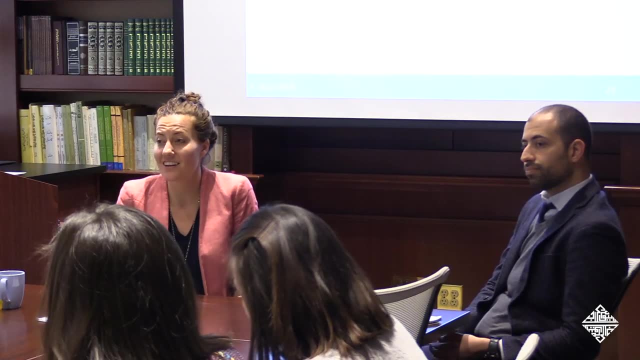 the whole book in. yeah, this book I think a lot about the students as well, But so, yeah, I'm very I understand that perspective, definitely, But I also think that not everyone has those opportunities, you know. and so what about the students who? 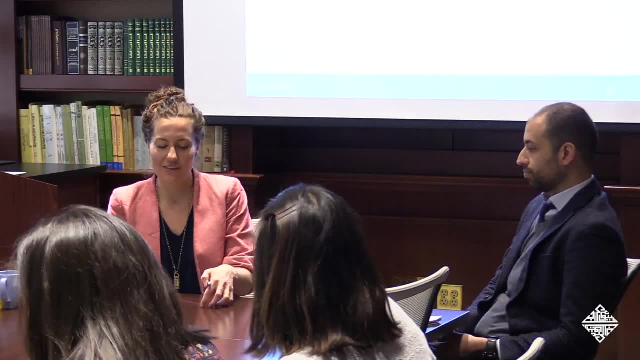 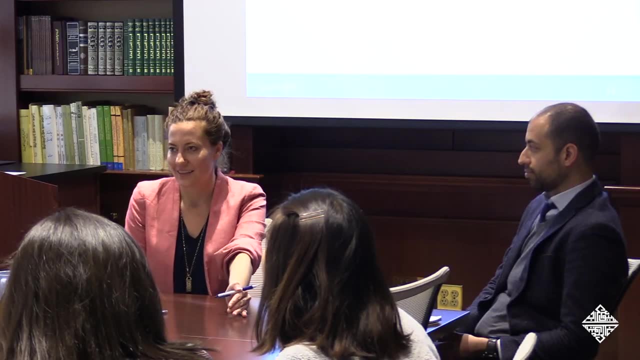 who you know, just going through this system where they're stuck studying in the public, in a public university, in a degree that they didn't want to study and because that's what they've been sort of slotted into and they couldn't do any better. 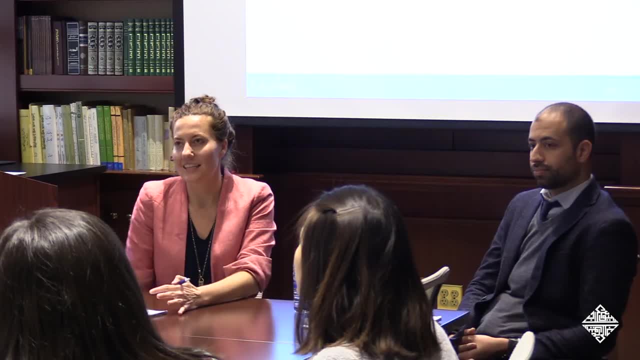 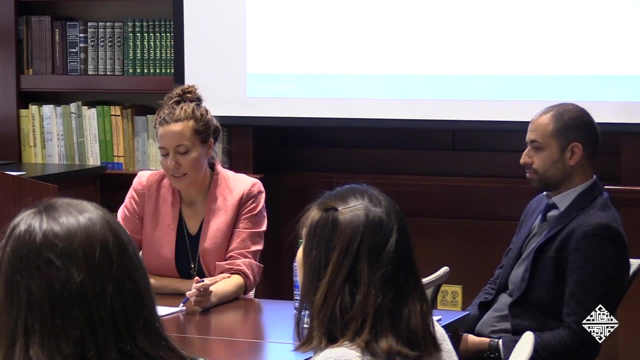 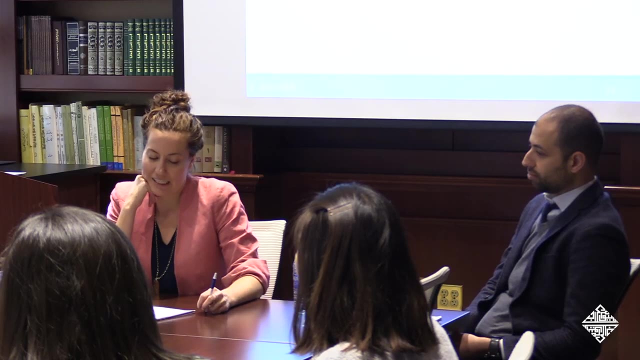 what then are? you know their prospects, And that's actually. and how do they then navigate that system too? So then, oh, the pedagogy question. that's actually really interesting. So in the what's interesting in the UAE: 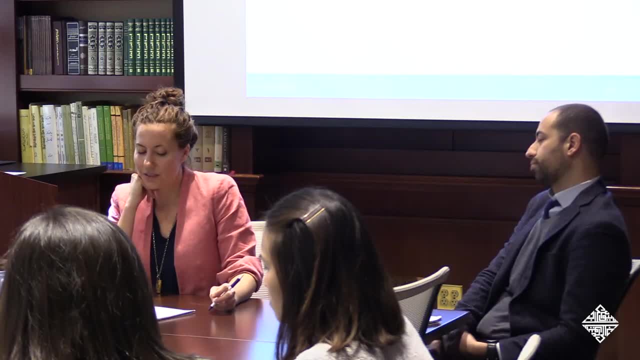 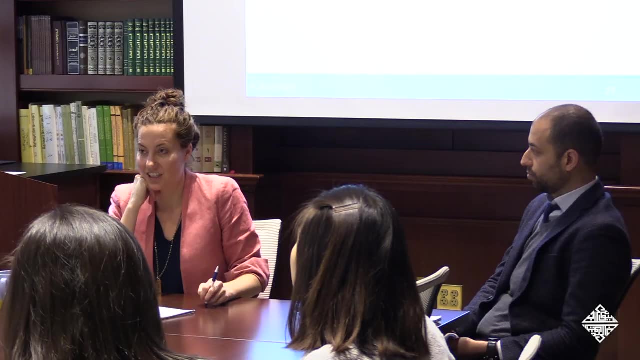 and the and in Qatar too, is that most- I mean very, very, very few- of the professors in the universities are actually citizens. That's one of the I mean like when I was in the UAE, like 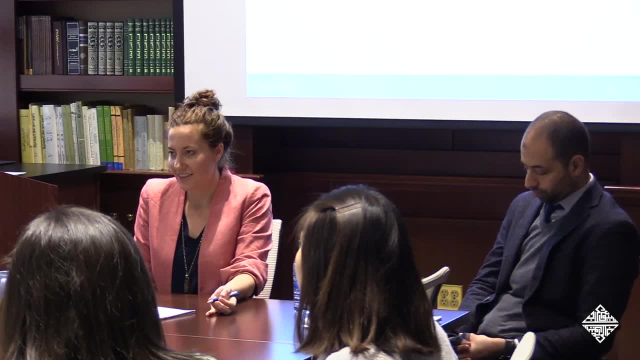 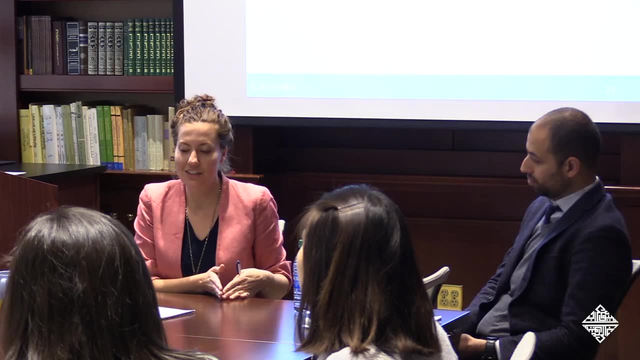 a survey came out of high schoolers in Dubai where they were all like literally the worst professors. I mean, being a university professor was literally ranked as the worst profession among them, which was so funny. As a professor, I was like. 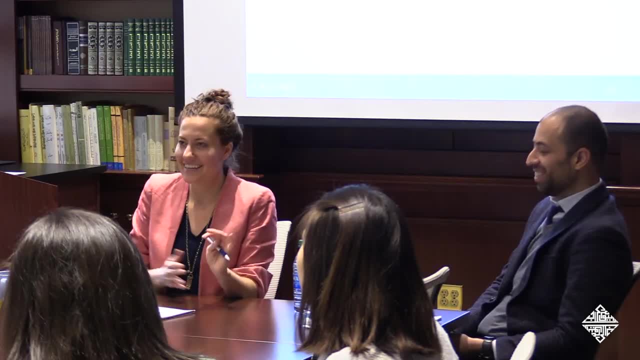 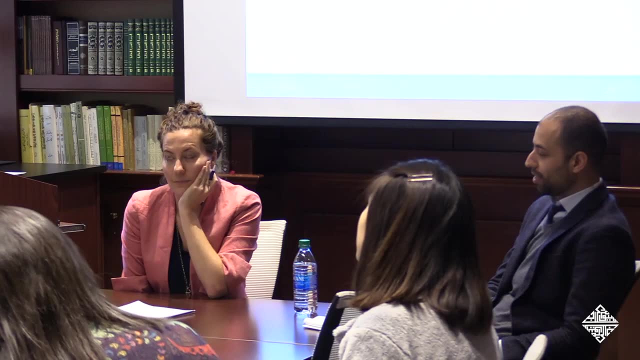 it's not that bad, And so you know it's. you know, but you know they have. so, in fact, most of the professors, even in the public universities, are are like other Arabs, often from other countries. 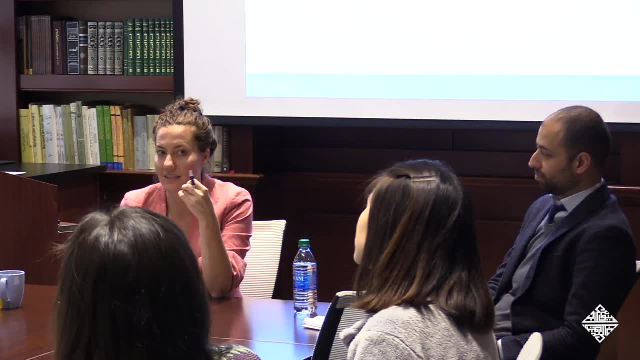 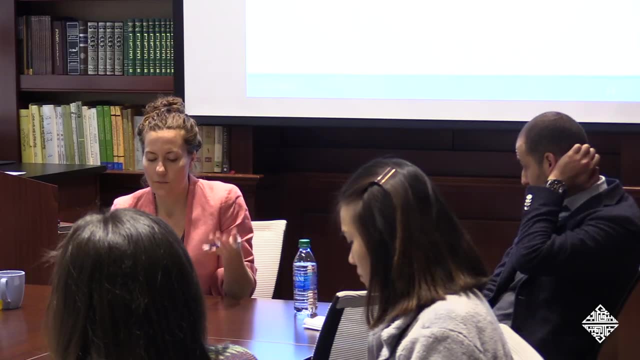 but not national citizens. they have a hard time. I mean, that is growing, I know, in some places, but the so. on one hand it's just like who are the professors? even that and where. 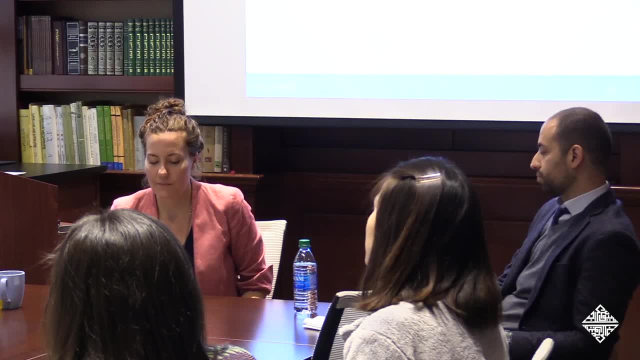 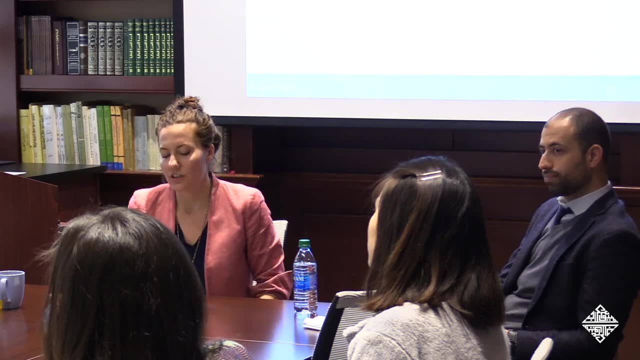 what are their backgrounds and where are they coming from. but you know, and then I would say, well, and that is particularly severe, we know, for males like we, especially in- I study a lot. 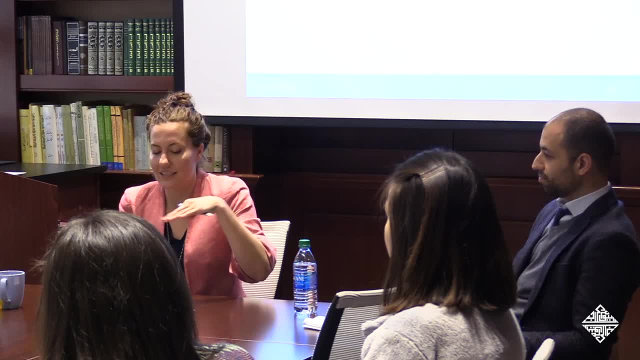 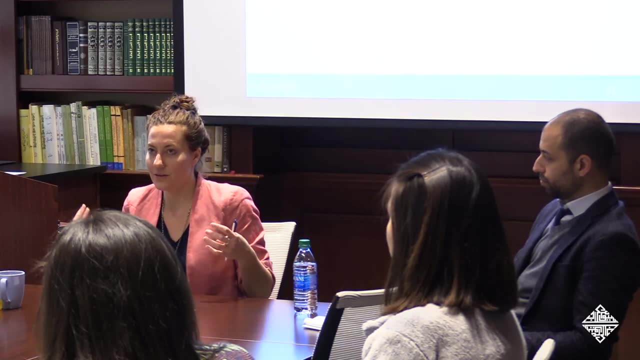 like the teacher labor market, in the pedagogy and in secondary schools, in primary and secondary schools even more so that in there are a lot of females who will go into teaching, but very few males who will, and so then, 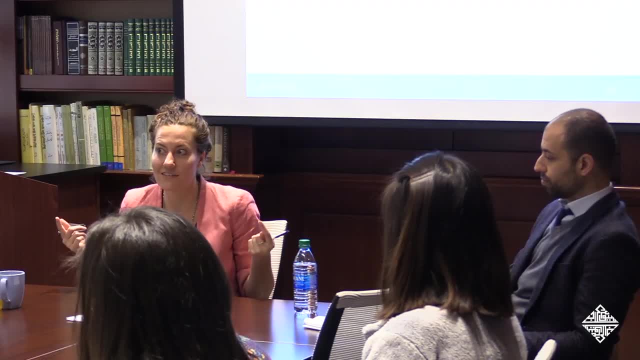 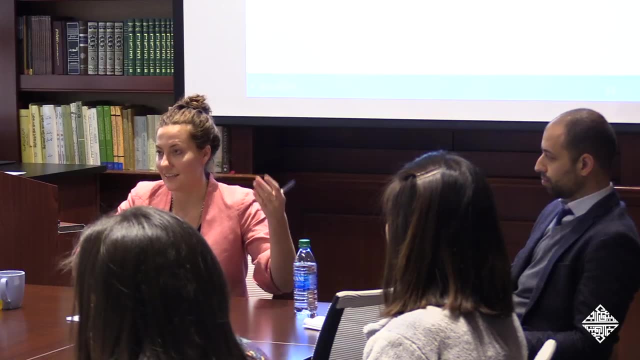 you end up in. you know it creeps me out that there's a lot of educational implications that you don't always think about when, like, the girls are being educated by their citizens and the boys are all being taught by non-citizens. 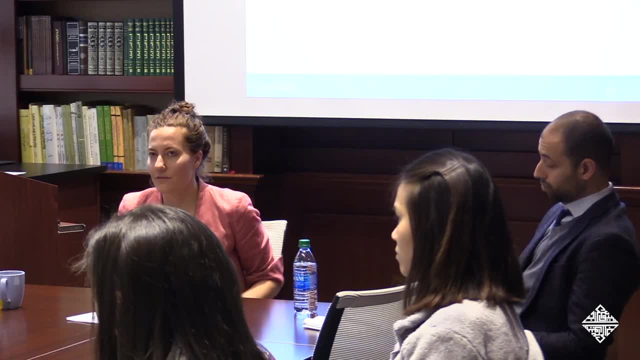 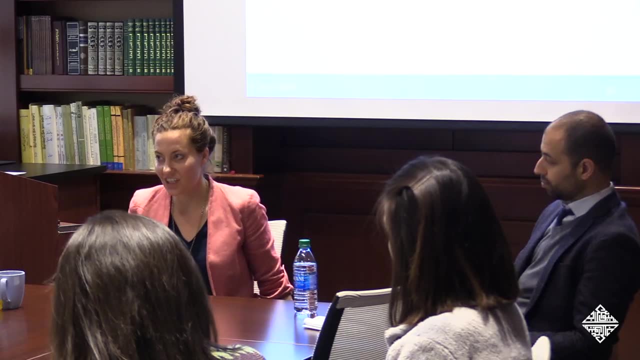 and so there's actually a lot of people who are looking at sort of why. you know, women in general are going to succeeding in education, graduating from going to university at much higher rates than women, and there's. 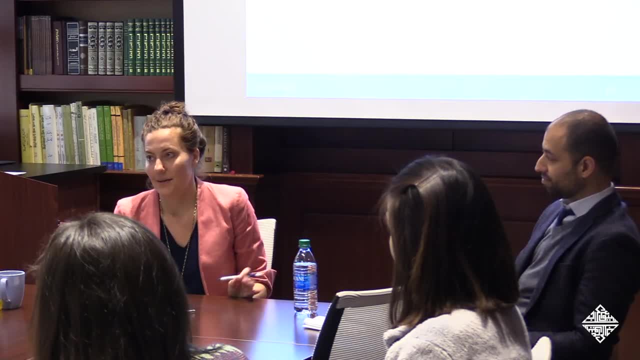 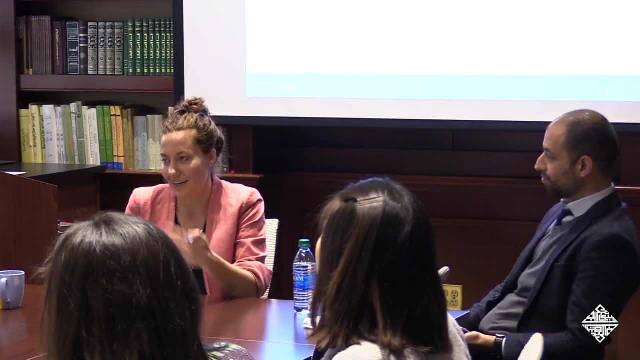 it's actually very complicated why that is, but I I think, from my understanding, like most of the professors are still sort of trained abroad. I mean, you know, offering PhDs is actually pretty new to some of the universities. 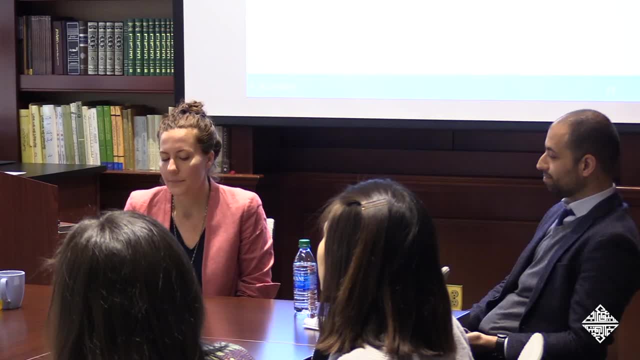 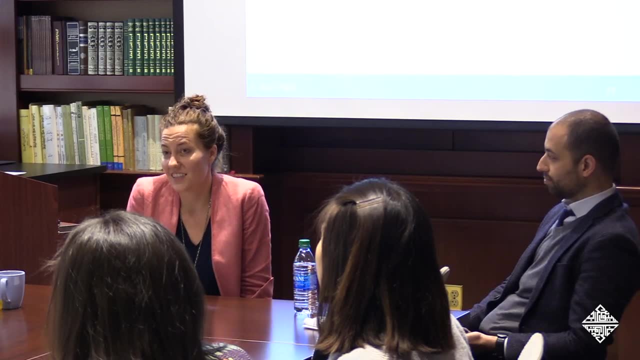 and some still don't so. but yeah, one of the things when I was in Qatar, the my interviews highlighted was that Qatar has invested a lot of money in trying to educate homegrown researchers, as they call them. 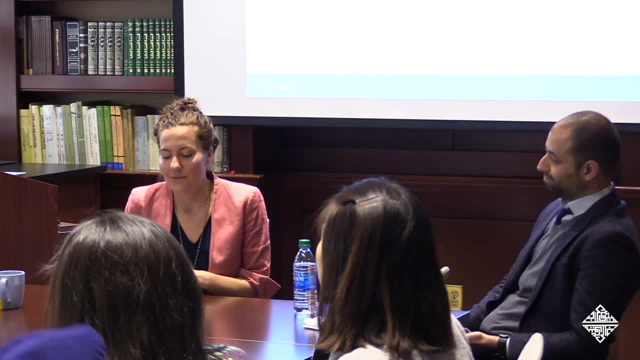 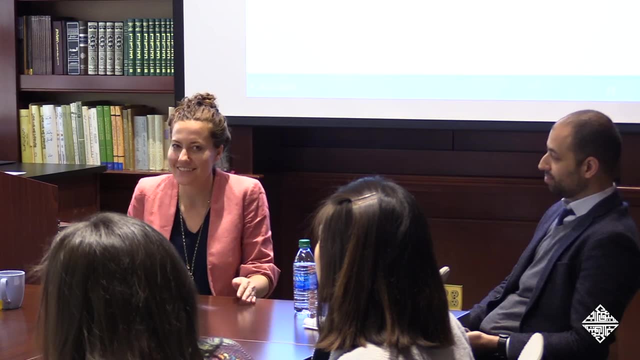 sort of they. I yeah, I did an interview with someone. he was like you know what? they spent so much money and they they've. he was like they've succeeded. it's like okay, it's not hundreds. 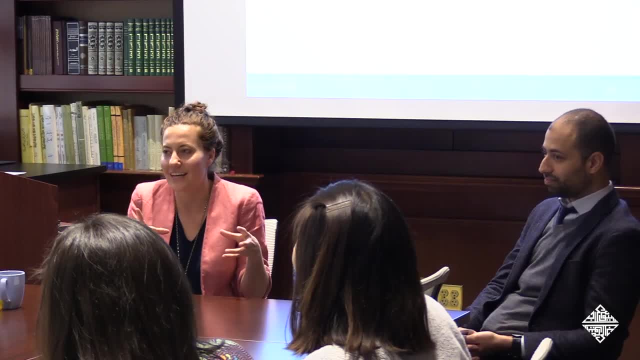 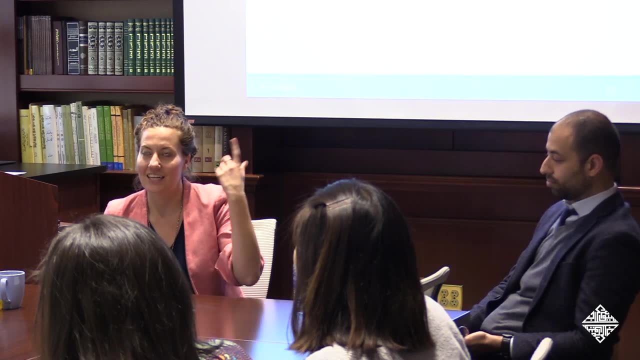 it's not even you know it's. he's like it's not thousands, it's not even hundreds, but we have like a dozen now, like a dozen scholars who are doing educational research in Qatar and 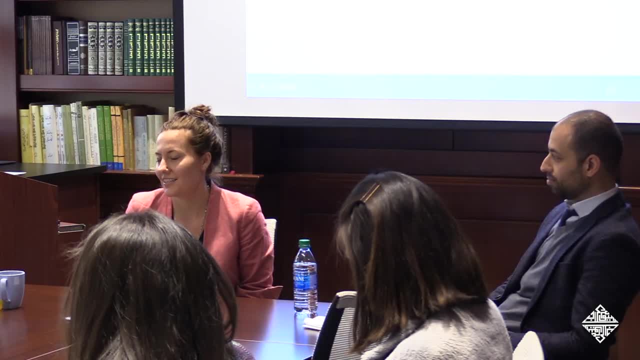 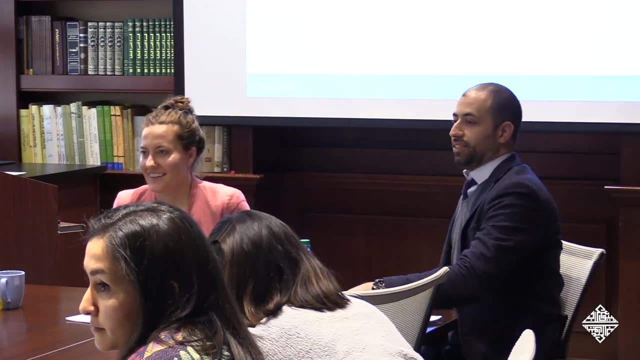 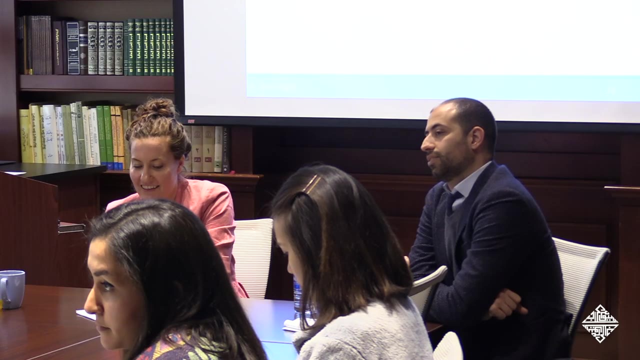 educate and to even do a PhD and then come back and be trained as a researcher. so they were proud of that. Yeah, I wanted to ask you a question about the private and public divide in Jordanian universities, just because I know in public. 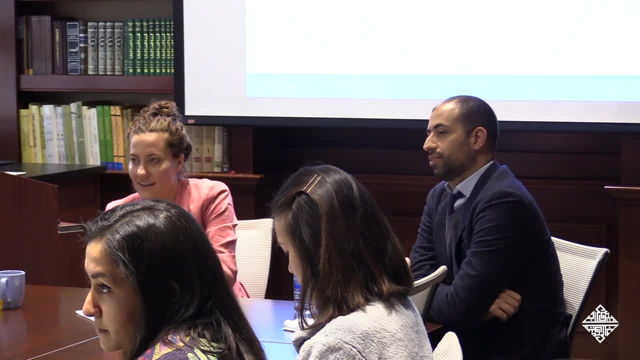 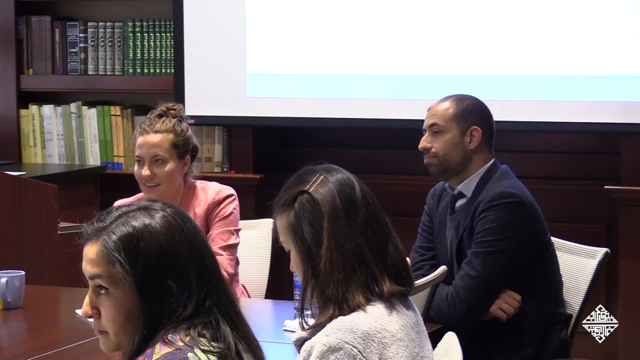 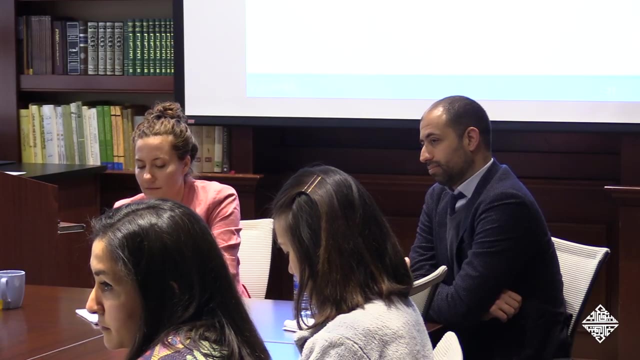 universities. there are also like internal systems for the like, the parallel system, and the international system, which, as a result, you have another opportunity to enroll in a public university if you pay more money. So I was wondering what. 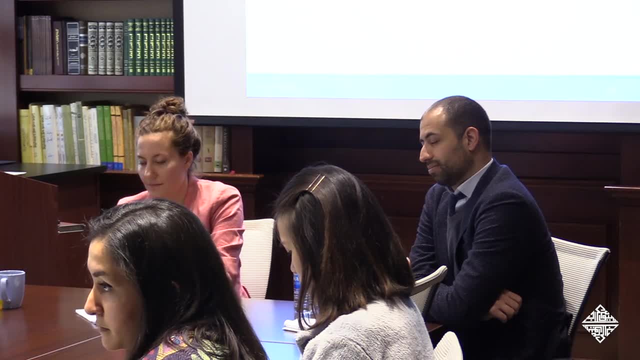 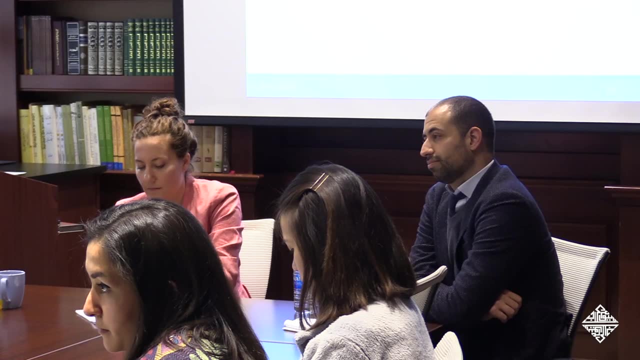 like, has there been kind of like, what's the conversation around that Like, is that a coping mechanism for, like demand of access? but then, like, if we're thinking of access, who can actually access this and who can afford it? 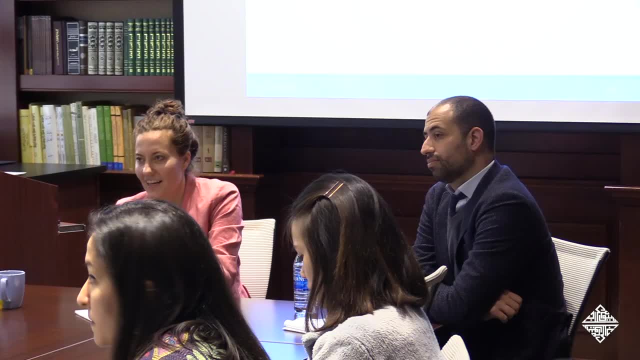 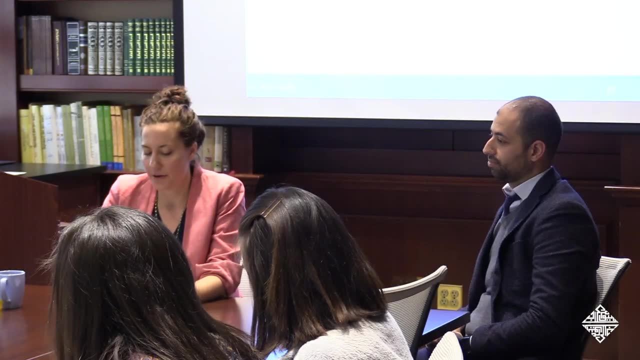 or is it kind of a manifestation of privatization in public universities as well? Thanks, That's a great question. So that exists, the parallel tracks. I would say so in higher education. a lot of people call that the privatization. 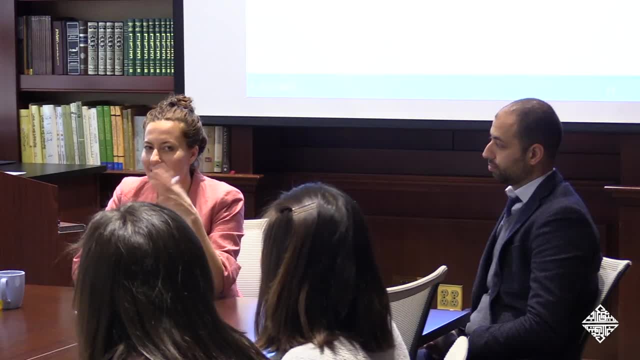 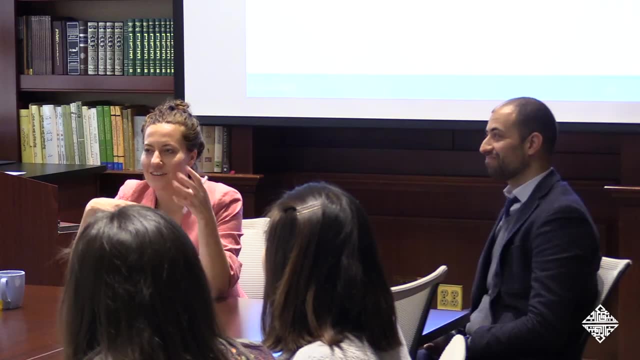 of the public system, or, and that's what you know- if you're more critical of it, that's what they call it. If you're sort of an economist, they call it cost-sharing, so that you know you're just increasing. 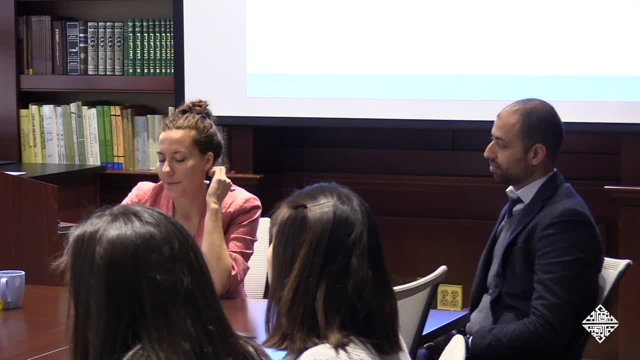 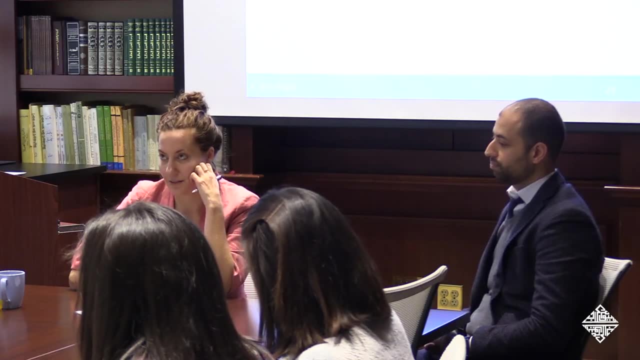 the individual's private financing contributions to the public system, and that is the model. yes, but it's not only in Jordan, it's in. I mean, Egypt has had a parallel system and Syria instituted one. that is, that was seen as. 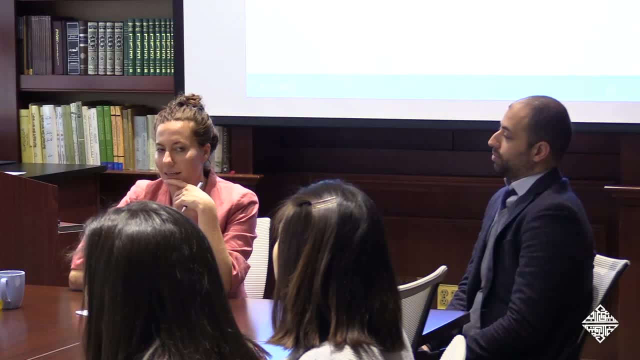 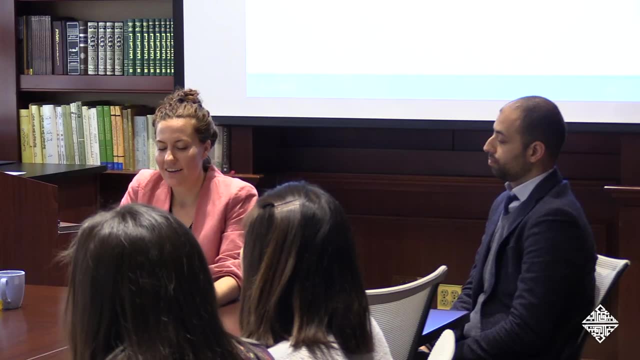 like you know, in many cases like a good model because it was bringing in more revenue and it was, you know, getting when I was there. I'm trying to remember where- I think it was in Jordan- I was doing. 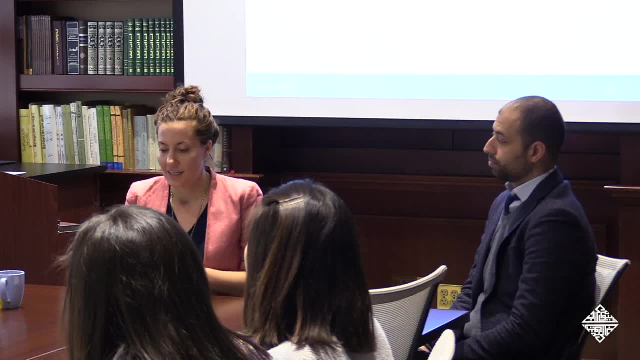 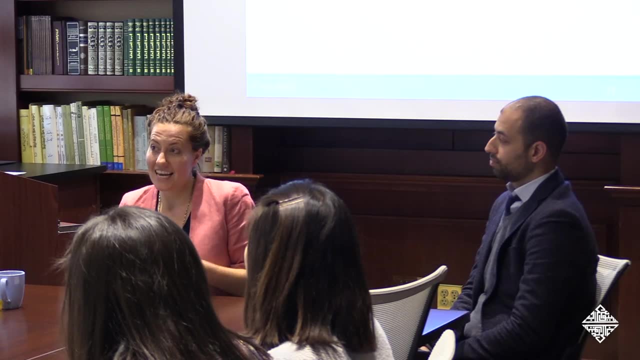 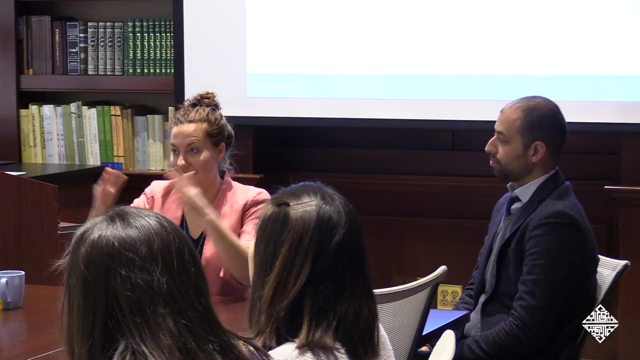 some of this research where people were very students in some cases, like you know, just wrong that you and I would be in the same classroom but paying different amounts for the same, like opportunity to learn literally in the same space and the same degree. 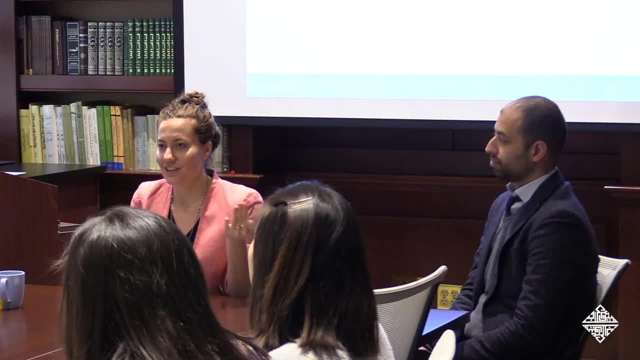 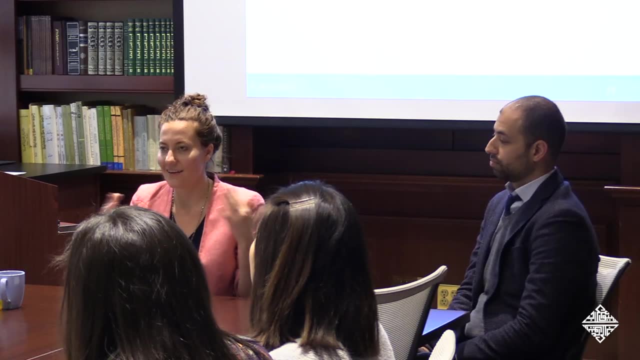 like. but whereas, like if you are American and you're used to the financial aid system here- students are always paying different amounts based on like sort of their family need, and so for me it was quite a different interpretation. 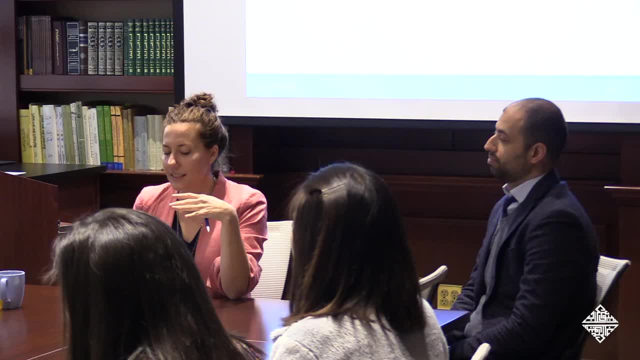 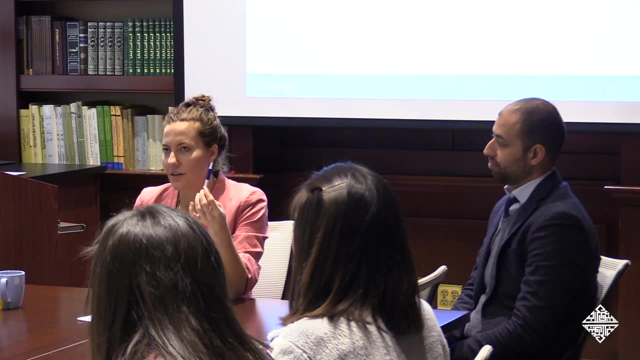 of you know as sort of a wrong thing that, but it is. I mean, I think that it makes sense when you think about sort of the interests involved, like the. it's still cheaper than going to some of the private universities. 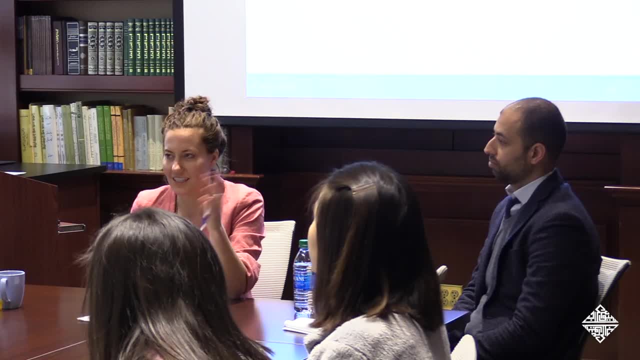 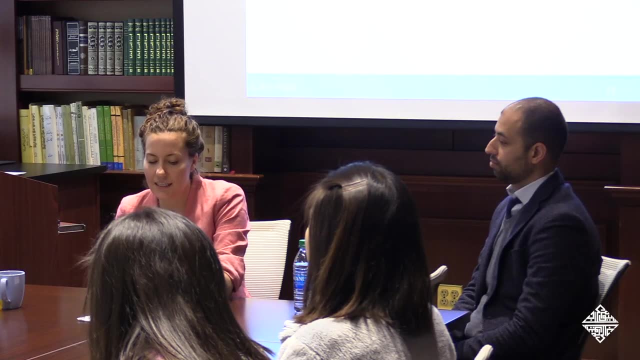 right, It's still. it's like three times as much the tuition I think in apparel in three to six times as much as going to the if you, if you're in the subsidized public system. but it's a lot of different. 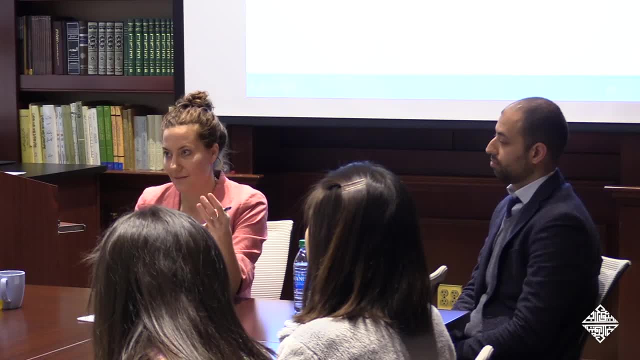 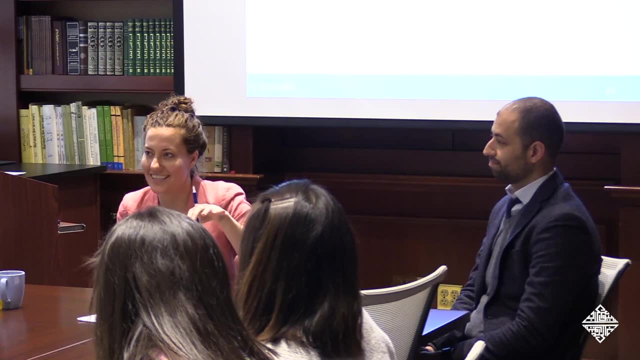 I think, in terms of, you know, specificity, and so it's a. it's a different kind of thing, I think, but it's, I think it's the same thing with you know, with the you know. 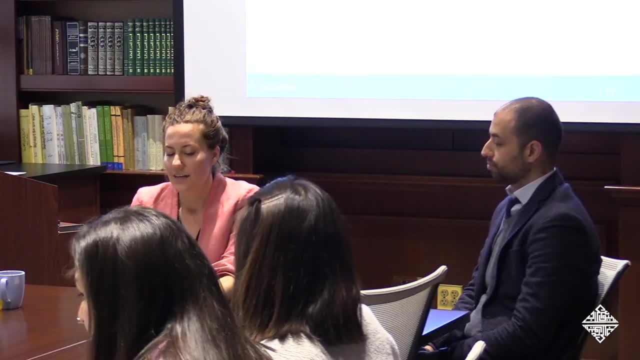 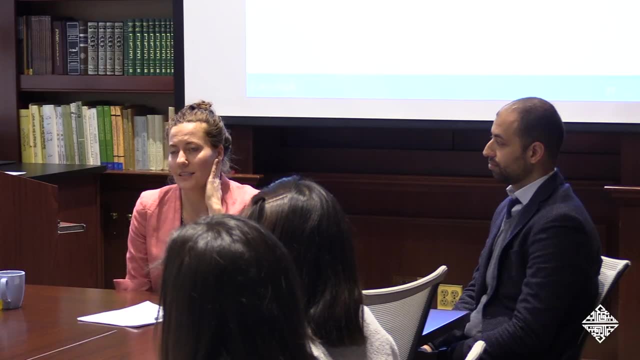 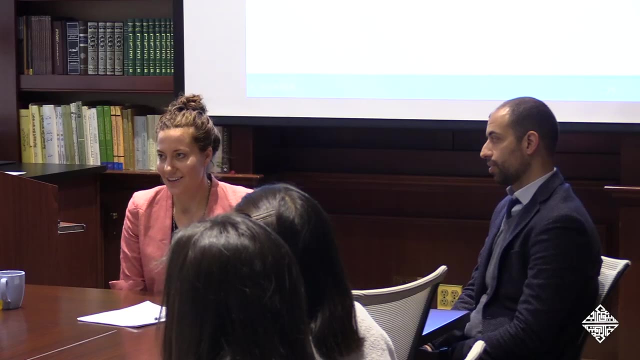 the health care, you know the health care, and so it's- I think you know the same thing with the. you know the, you know the medical- that they actually their scores were not that much lower. You know, in many cases they were just marginally lower. 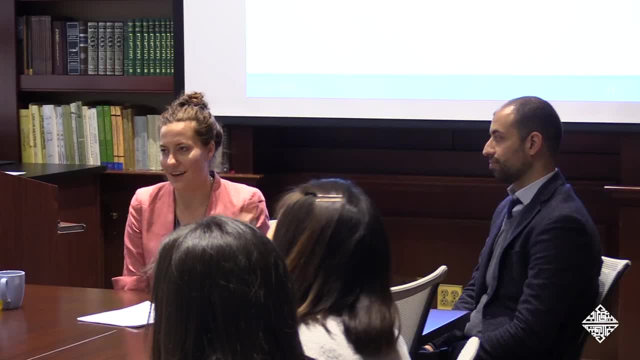 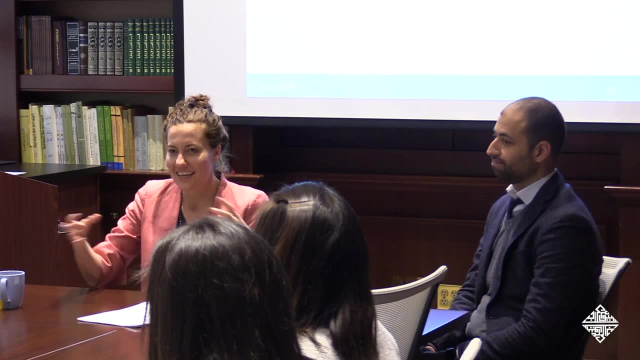 and they would point to students on scholarships and other programs that had much lower. you know, students from rural areas getting preferential treatment at lower scores, et cetera. There's like it's very contentious there but who gets access to, who gets to sit for this program? 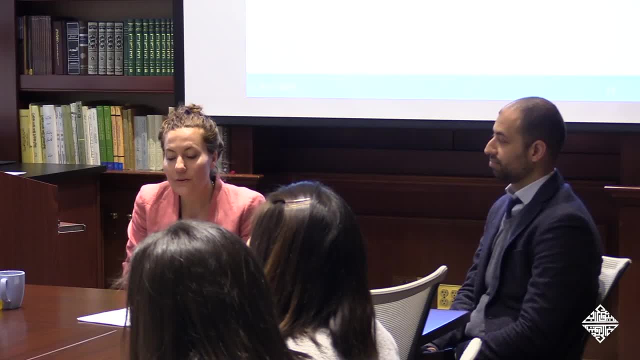 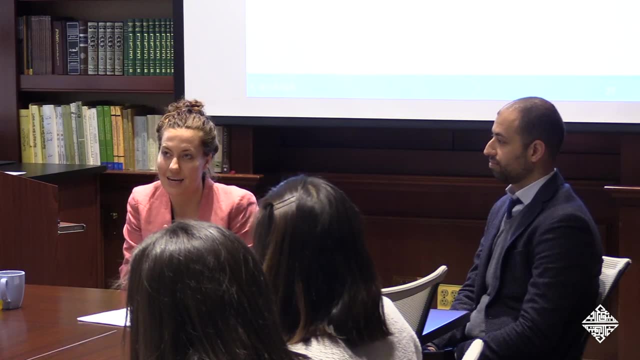 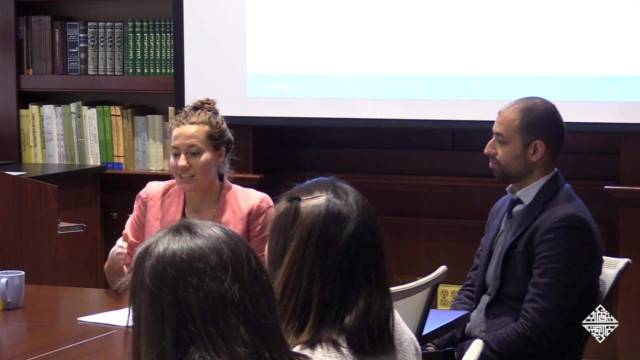 based on their background, And so I do think it is. yeah, I think these programs have emerged and are sort of thriving in these particular places because they are serving so many different demands, Like demand for this prestigious program from the families to a little bit more money. 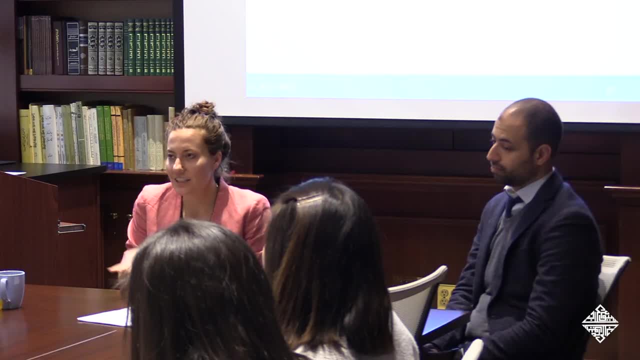 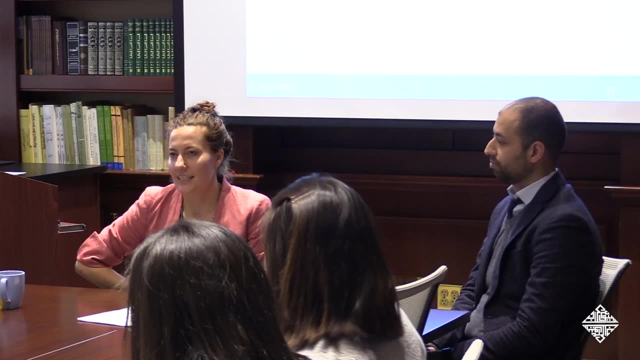 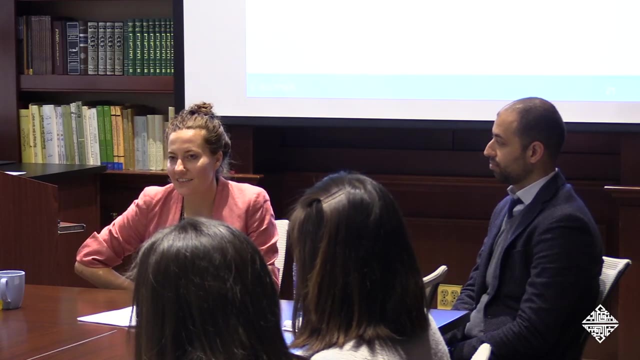 for the public universities And they're still cheaper than sort of you know, a purely private institution in many cases. And yet those are not, you know, taking off in North Africa, because it's harder to even like. there are protests even at the thought. 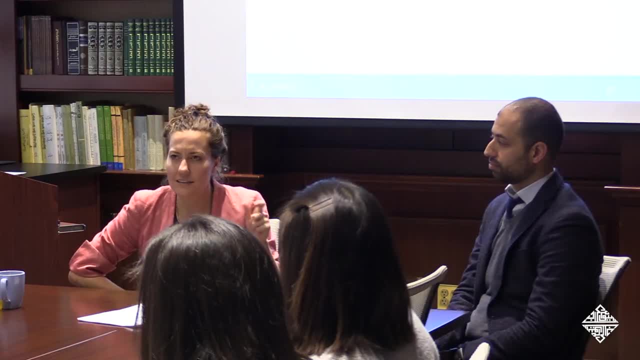 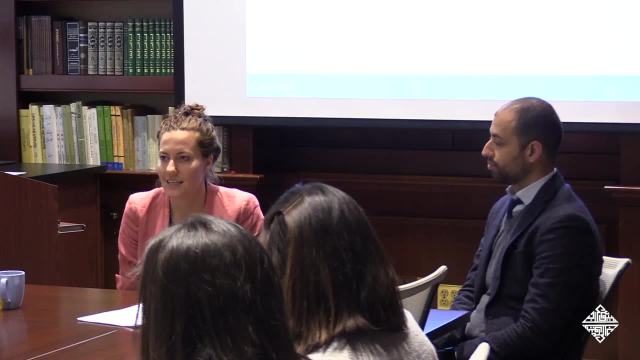 of charging tuition. in some cases, You know, although it's not in, you could see them taking off in, like the pharmacy or the medicine programs there as well. But there I think it was sort of in all of the countries where there's sort of. 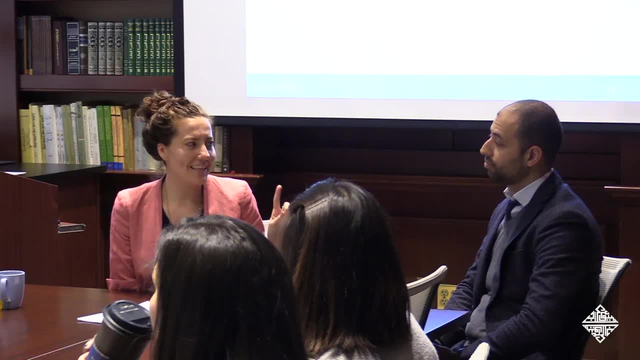 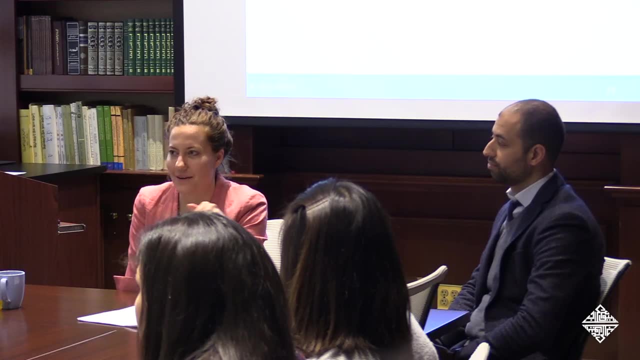 I don't know well. I guess it's taking off in Egypt too, But in Egypt they're very contested. They went to like the Supreme Court had to rule on them and they actually like struck them down at one point. 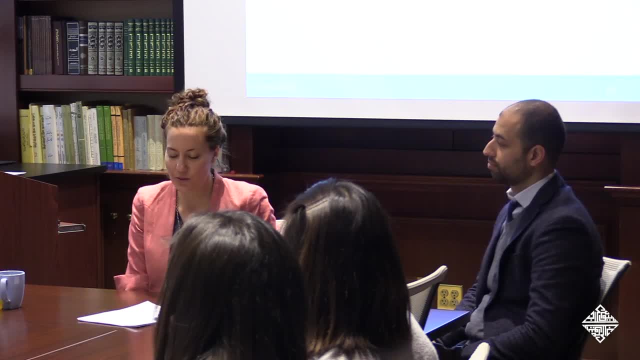 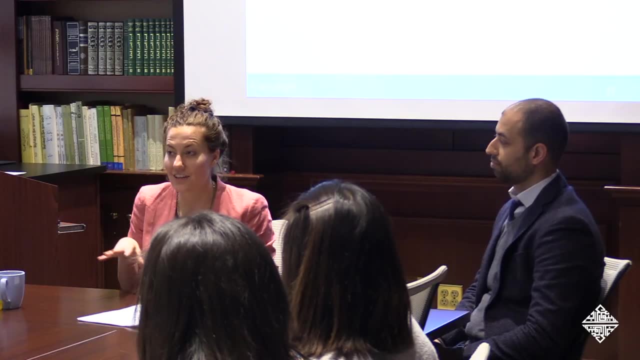 because they were, you know, because tuition- they were seen as tuition and tuition is in the Constitution. you have to have free public higher ed. So like I do think it makes sense that they are less contested in Jordan, where there's sort of the implicit. 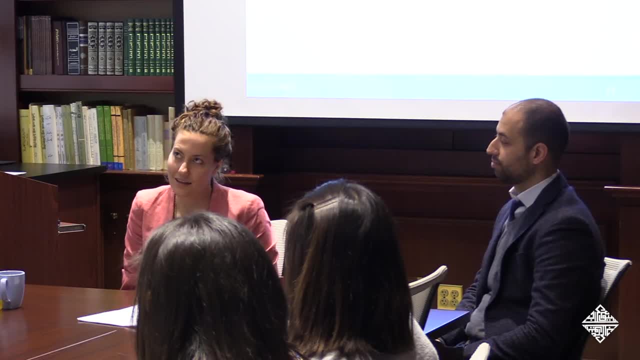 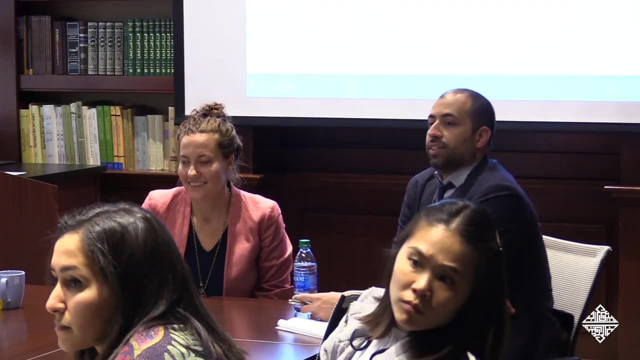 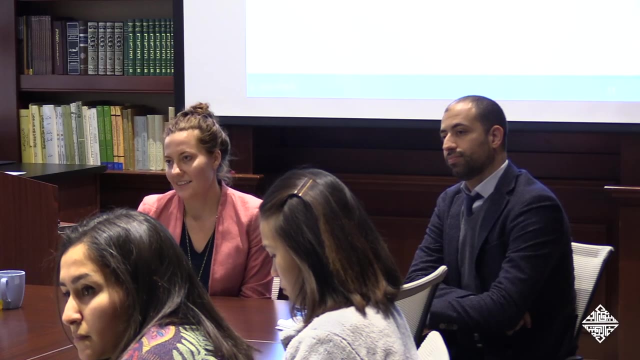 we're already in the public system. people are paying some tuition and whatnot- than in North Africa. Time for one last question. First of all, thank you so much for sharing all this information, Like when we talk about equality education or education for employability. 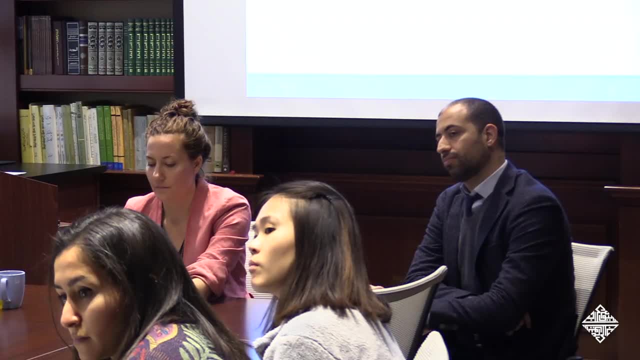 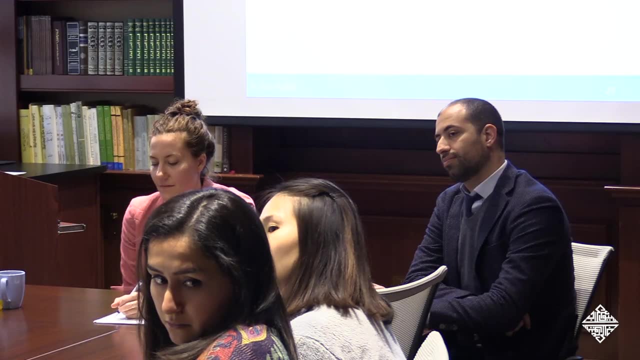 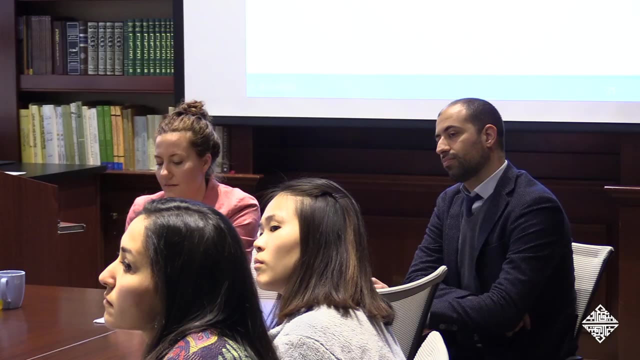 we always focus, exclusively focus- on what the institution is doing to help the students, But isn't this actually not the reality, in the sense that students, particularly in the context of economic despair, do exhibit agency creativity and initiative in improving their education? 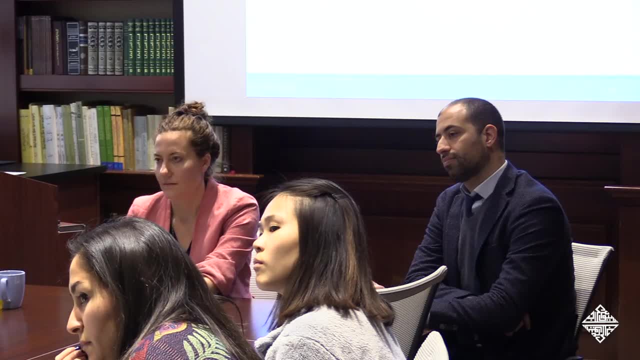 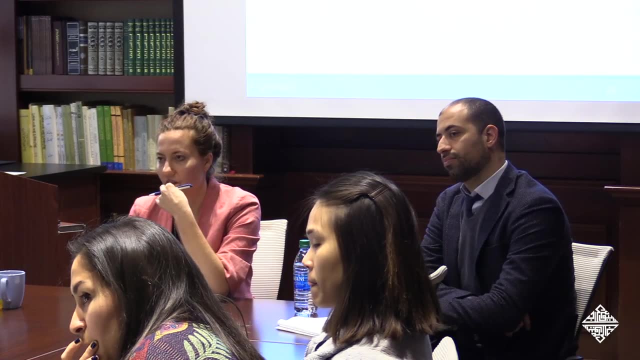 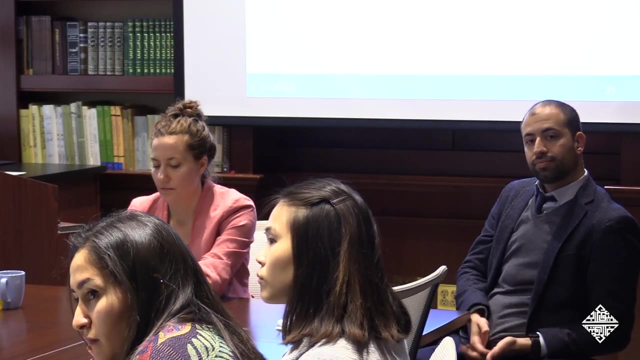 In their overall learning experience and employability. I'm just again, of course, two studies of Jordanian students, and you know they showed that you know these students and learners do exhibit these levels of agency and effort, individual and independent effort. 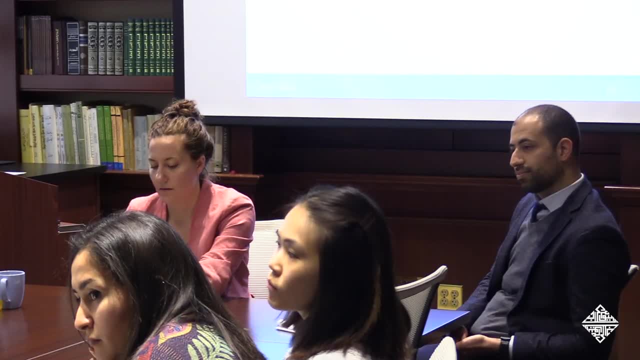 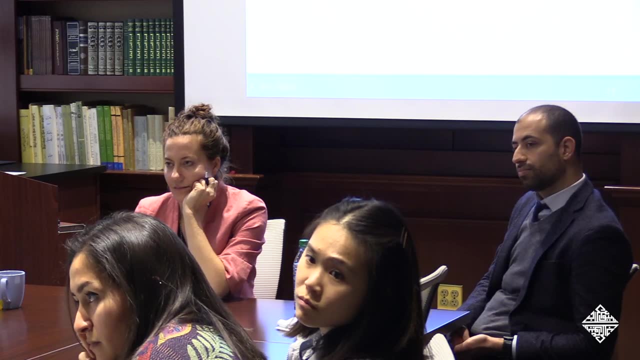 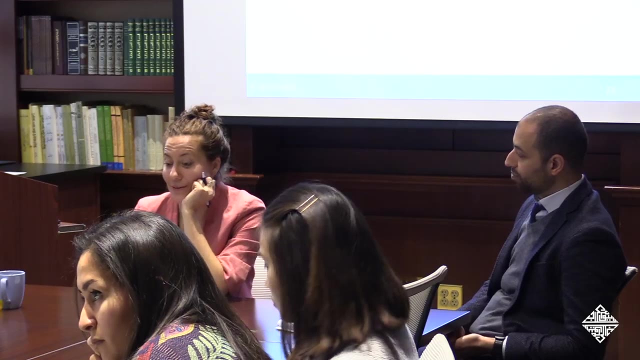 in improving their learning and employability. So I'm wondering whether it is time to include in scholarly discourse non-activity in both areas of equality, education for employability and the role of learners. Yeah, I think that's a great point. I definitely agree. 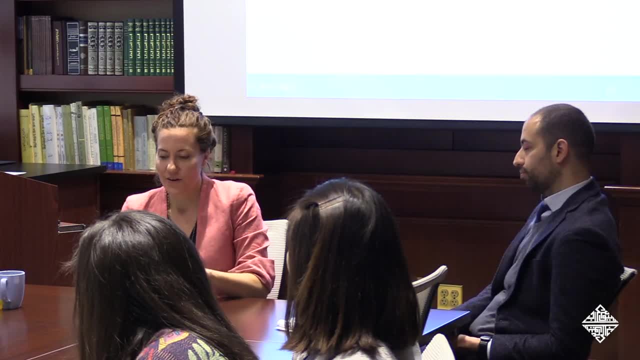 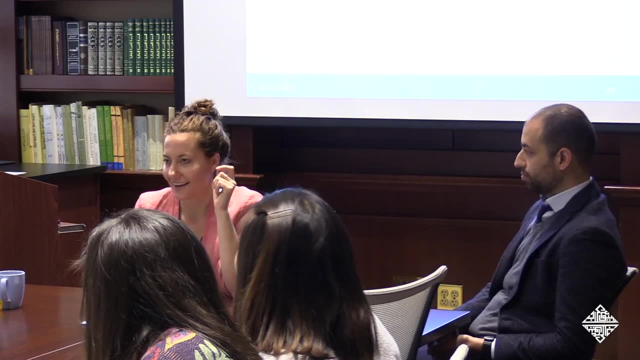 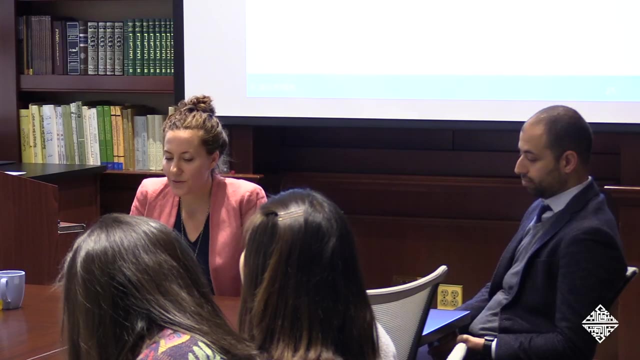 Like students are, you know, they do exhibit a ton of agency and independence and creativity. They're, you know- hustling is the word we sometimes use here- to describe, like, how people are pursuing, you know, internships or like any number of things. 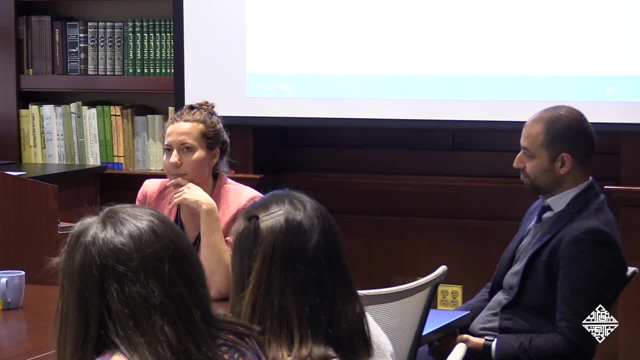 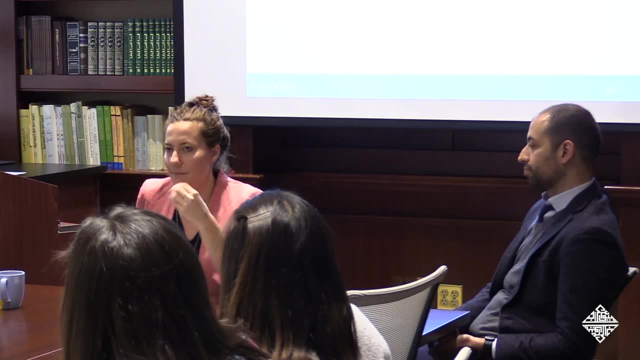 Yeah, They're training courses, But also- and yeah, so I definitely agree with you, It's not. I mean, I focus on what the institutions are doing in many cases, because they are sort of the institutions are the ones being criticized so much. 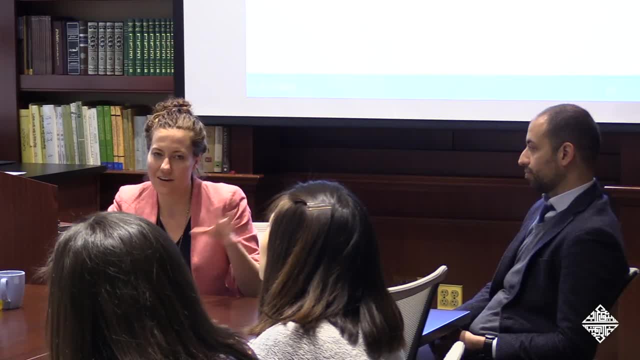 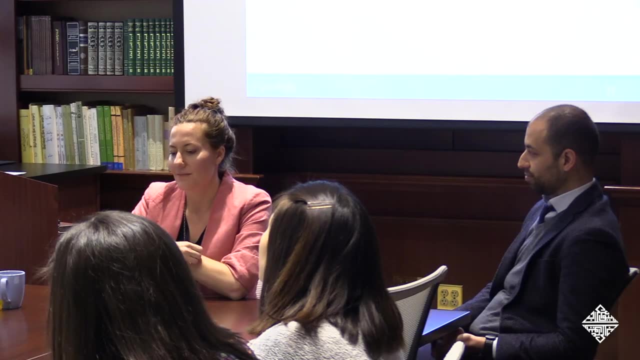 It's like the discourse doesn't- I mean doesn't often focus on it, like doesn't often portray students as like lazy and not and just, but I mean, sometimes it's like maybe portraying them as like. 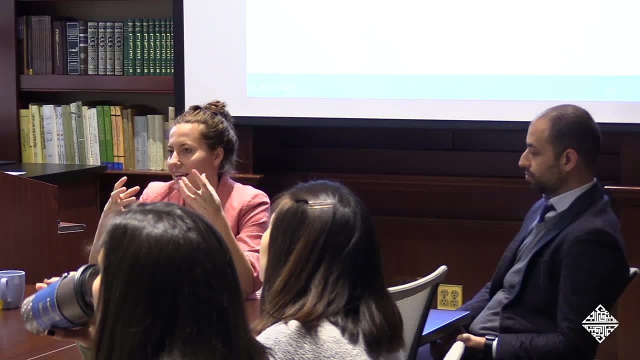 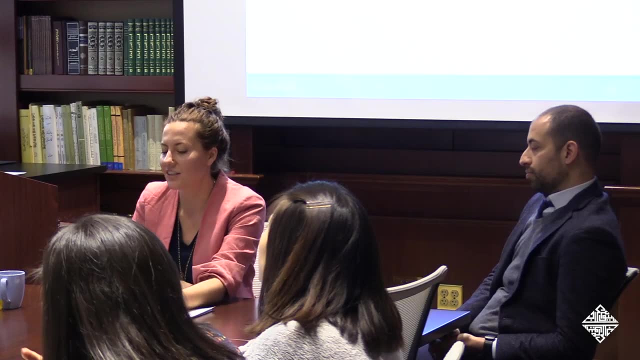 passive, yeah, in the wake of and just taking in their pedagogy. But I would also say that, yes, the students are independent and agent, and also that's where I see like faculty in many cases are too. 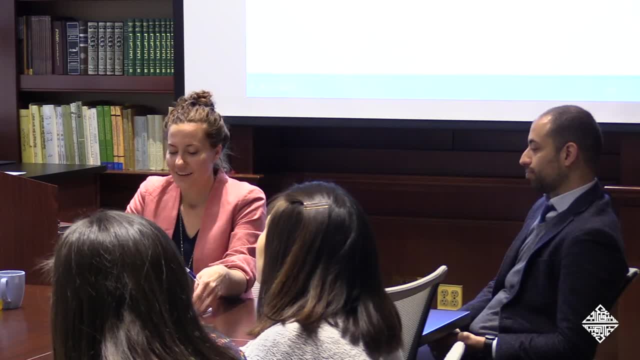 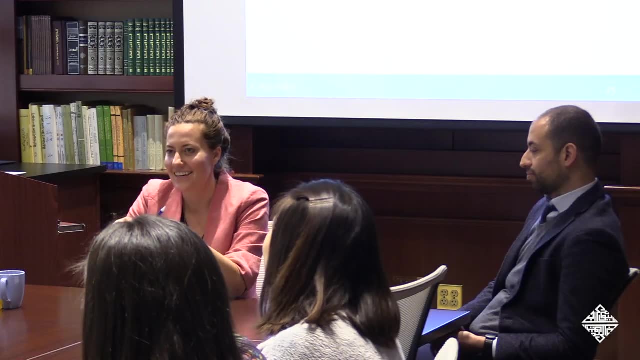 They're trying really hard. They're like, in some ways, you know, creating new. you know they're like evading these systems, too, in different ways and trying to educate their students as well. And so I, yeah, I agree.